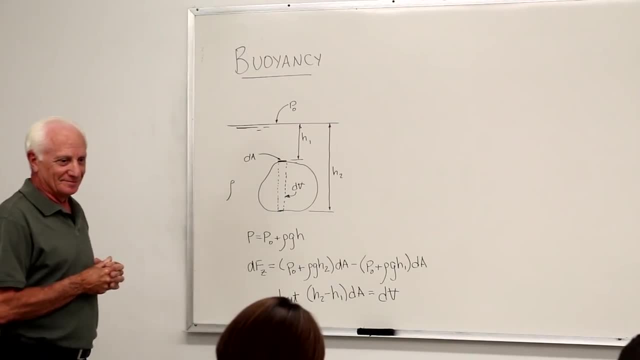 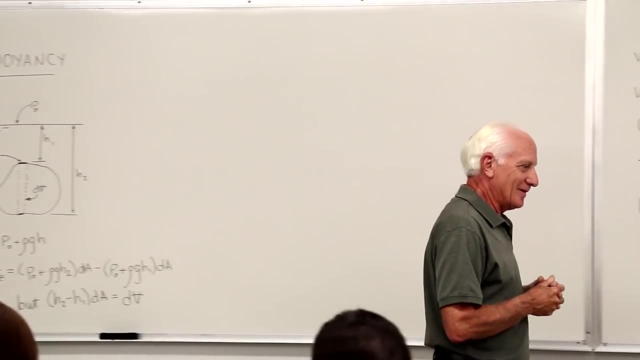 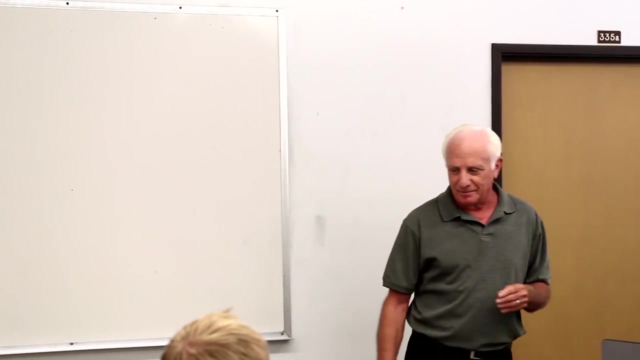 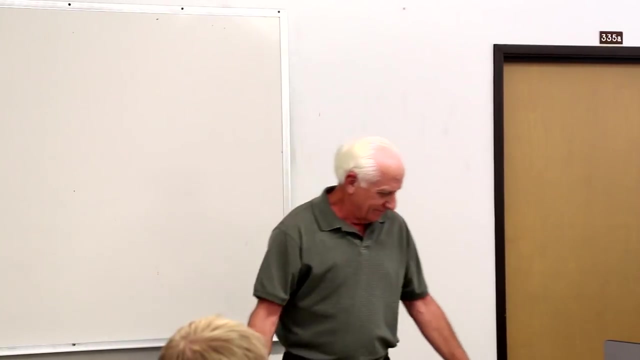 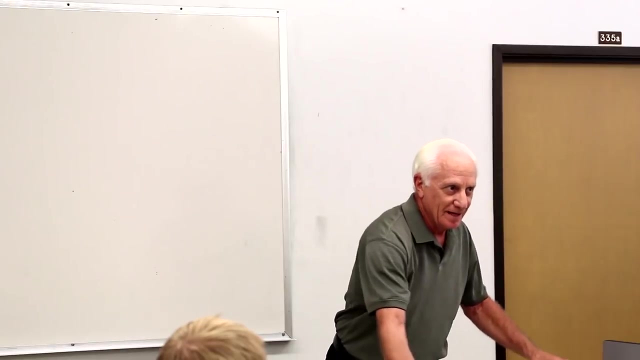 You're buoyant. So let's talk about buoyancy a little bit. Everybody has a good intuition about it, but you know, if A cup of water I'm not drinking tea, I'm not going to do this today. It's not that bad a day, Monday- but I'm not that desperate to do it. 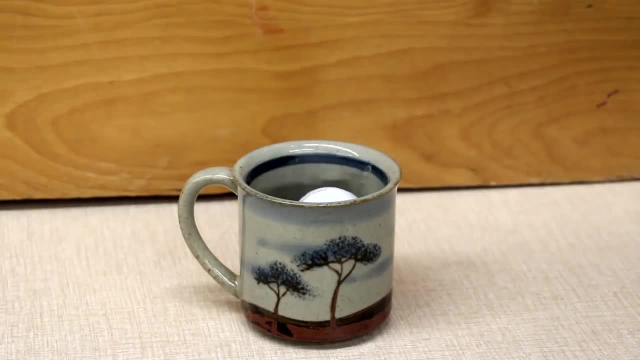 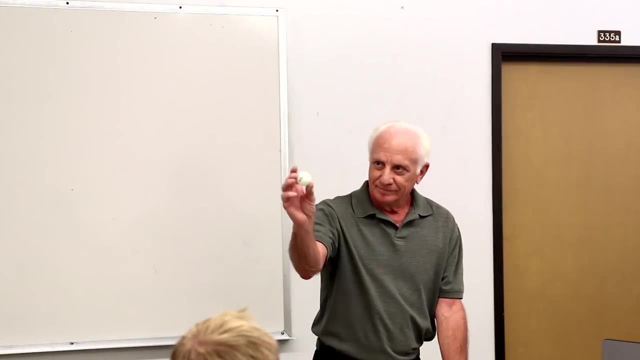 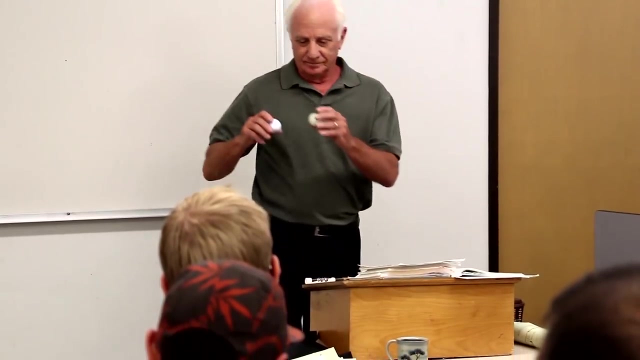 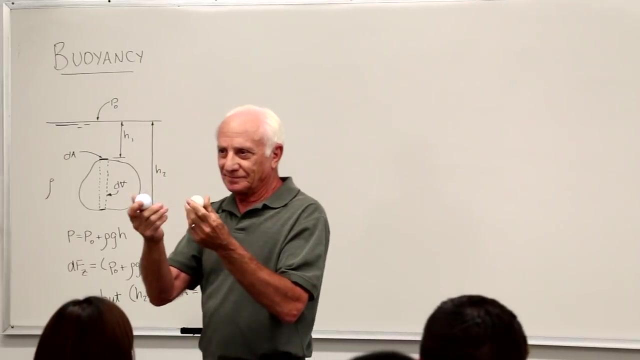 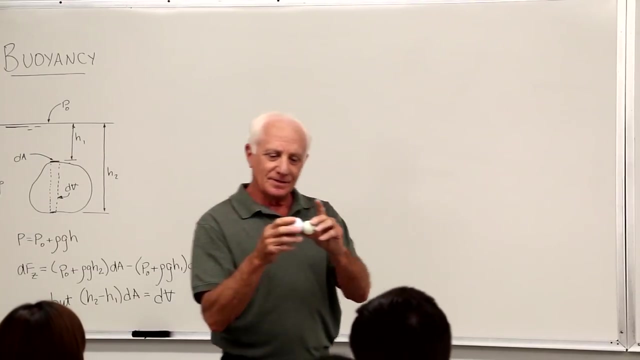 Golf ball: This is down at the bottom. Ping pong ball: It floats on top. They're roughly the same size. Why does one sink? Because of its weight. Density and the weight. That's right, It's the same, fine. so density or weight. 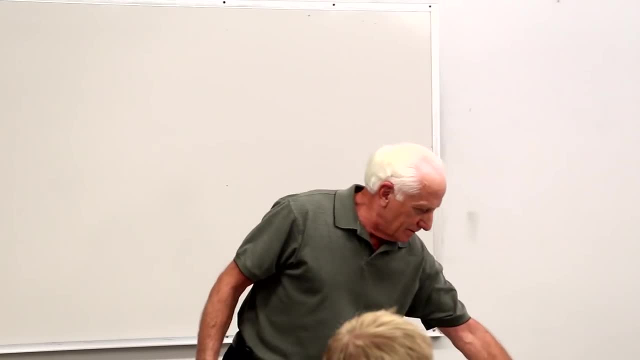 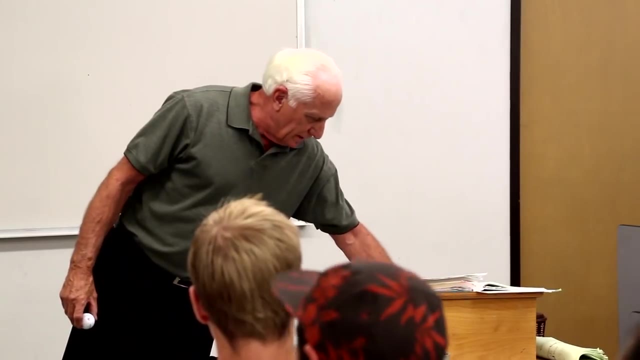 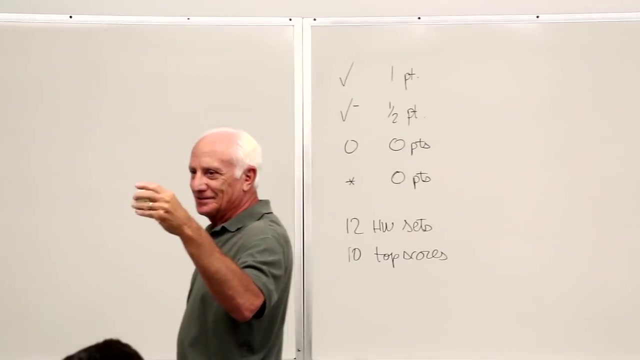 What makes the ping pong ball? It's not halfway down. even It's not halfway down, It's mostly floating. It's into the water way down here. So there's something else acting. there too, There's something else acting. 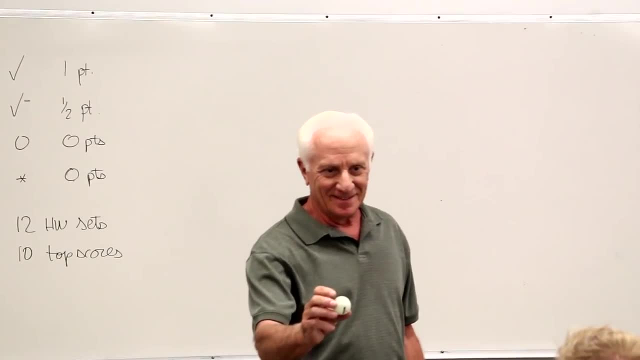 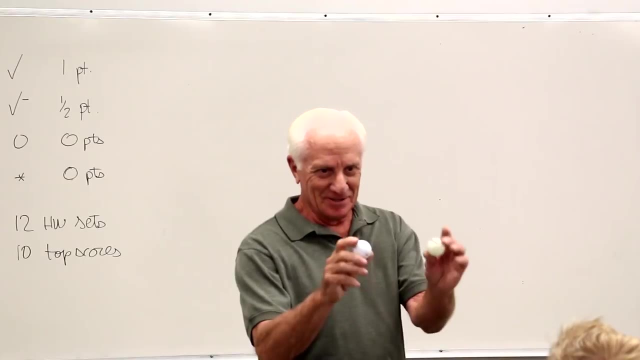 What two forces do you think act on it? What do you think act on it? What two forces? Buoyancy is one of them, Okay, And Gravity, Which one's heavier? Well, gravity, Yeah, This one's heavier, So this one's lighter. 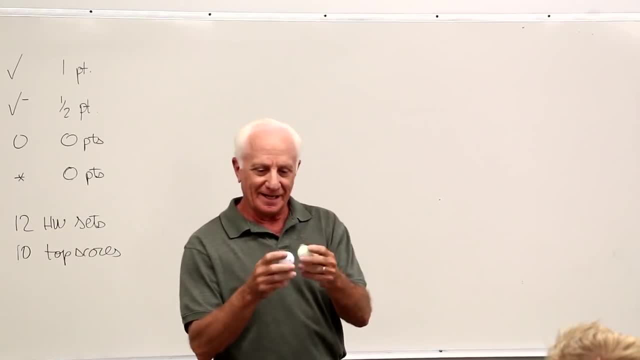 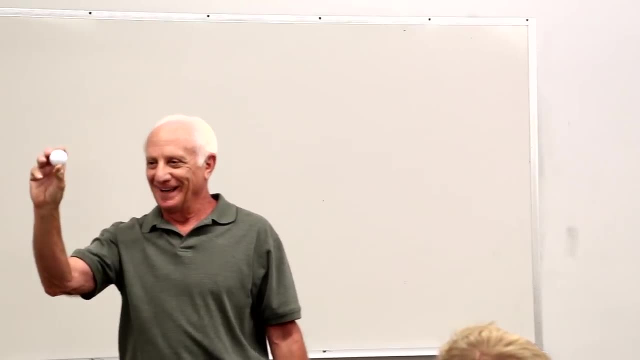 Okay, So that's right. A buoyant force and the weight, If it sinks to the bottom, guess which one wins: The weight, The weight Float on top. What do you have? Buoyant force up, Weight down. It's floating on top. 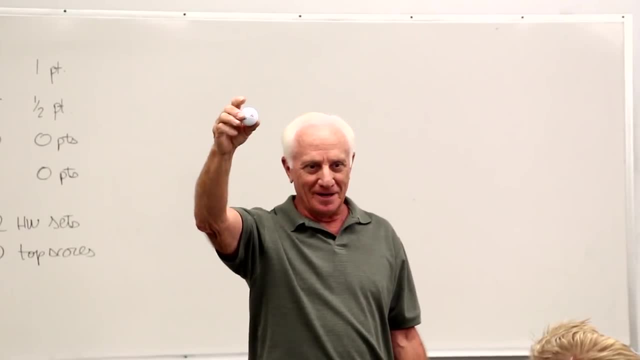 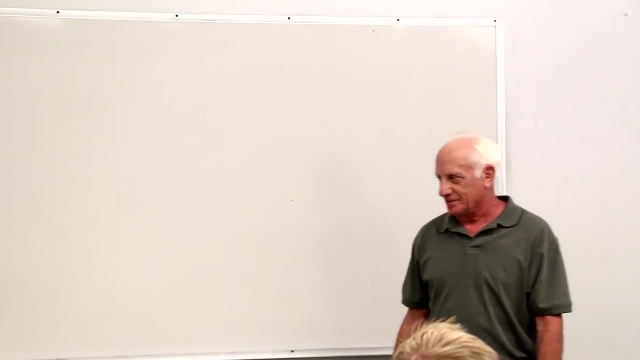 Let this thing go in the ocean, It'll sink a long way, Okay, So yeah, It's something about the weight. Well, you know what causes a buoyant force? You can say buoyant force, but so what I mean? I could say it's the Vesuvius force. 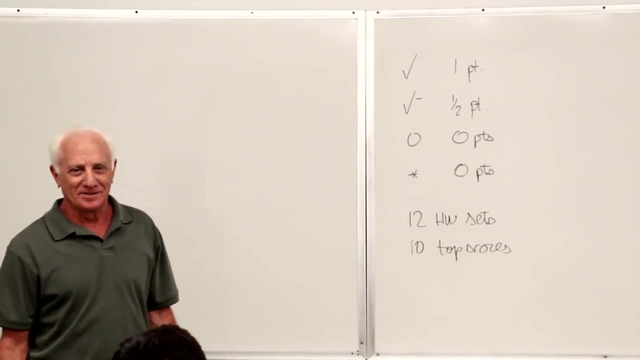 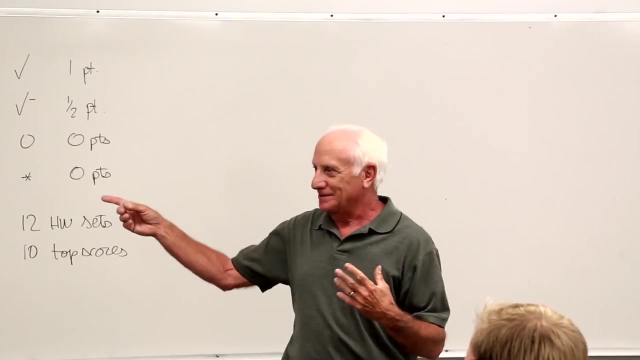 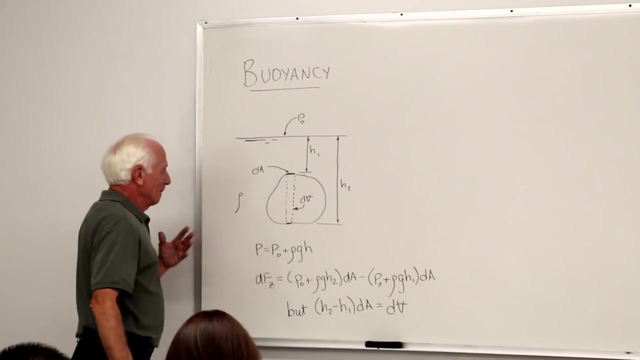 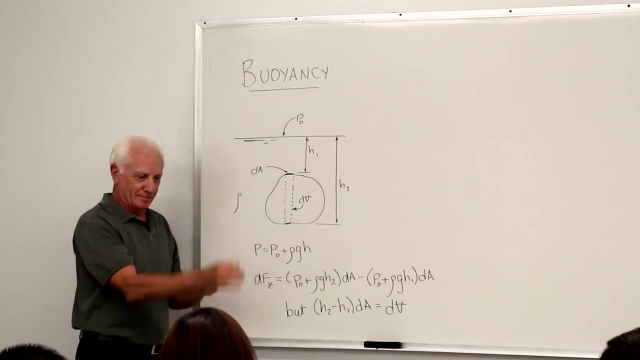 What's that? A Vesuvius force? No, Why is there a buoyant force? Well, that's what this picture here is going to show you. Here's an object: golf ball, ping pong ball, whatever Top. Take a slice of a little circular sliver of a cheese stick. 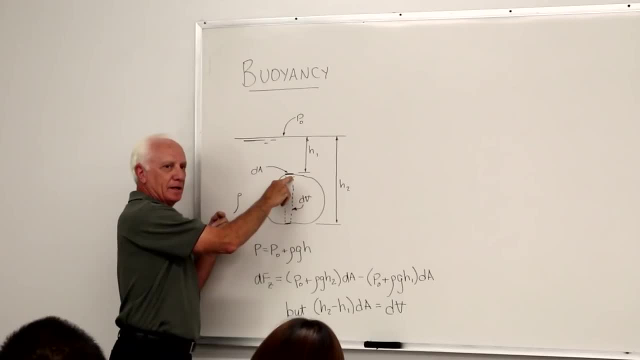 The pressure up here, Not too big, Okay. The pressure down here, Uh-oh. Bigger or deeper. Bigger pressure, Bigger pressure, Smaller pressure- Which one wins? Bigger pressure, What's the buoyant force? want to do? 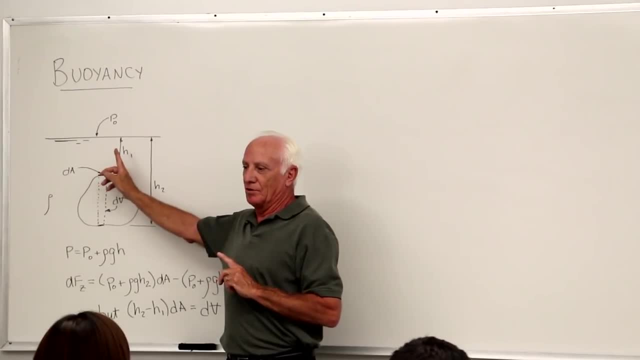 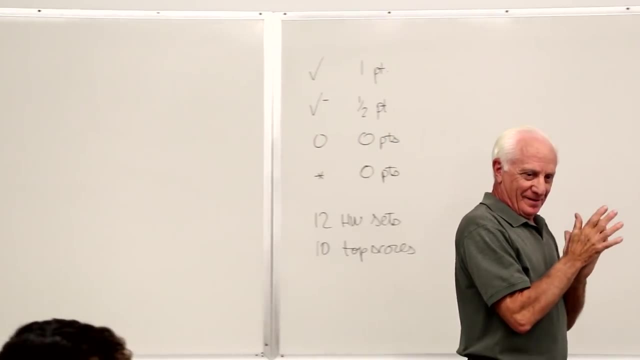 Raise this thing up. What's holding it back? Obviously the weight going down. So it's like a balance between the weight. If the weight's too big, the thing sinks. When you fill your lungs with air, you're floating it back. 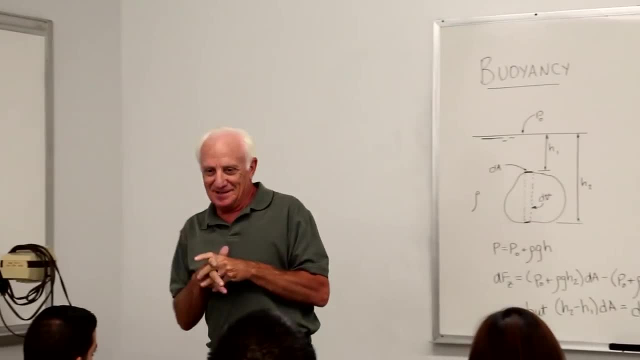 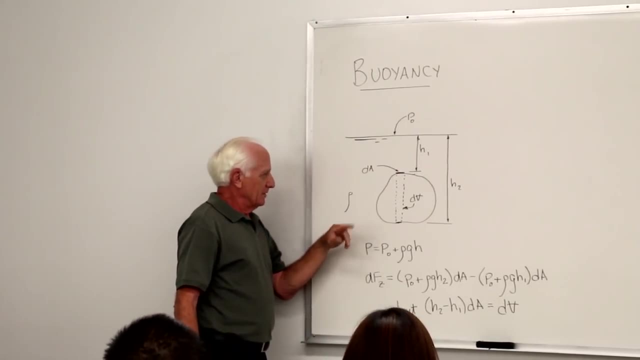 Yeah, That's right. Tensity goes down your air in your lungs, So, yeah, So here's our little circular area. DA, for instance, Do it vertically. Here's the free surface Pressure up here is P naught. 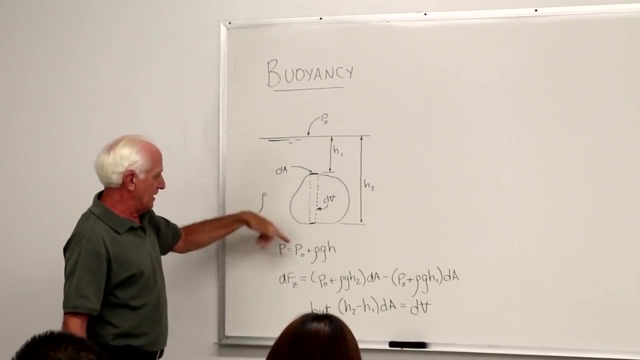 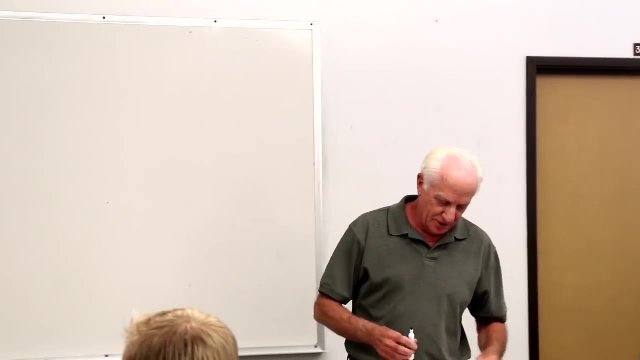 The equation: pressure goes up as we go down in the fluid. P naught is the surface pressure at the very top, And this is in your book. I'm just repeating what's in your book, but I want to go through it so you can see it more clearly. 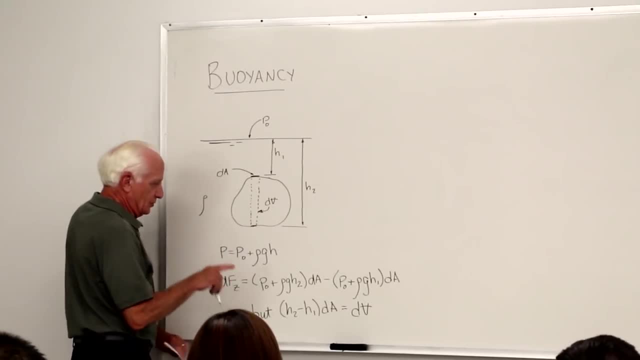 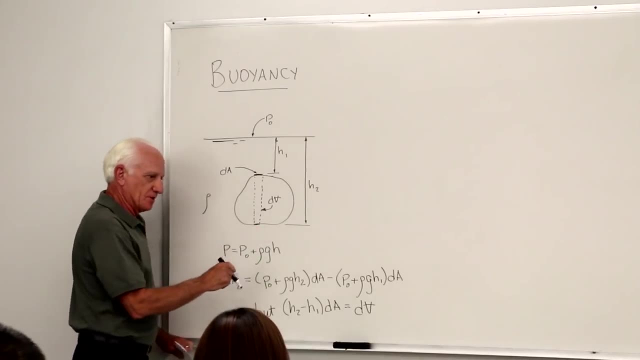 The sum of the forces in the Z direction due to pressure, Due to pressure At the bottom, big pressure. Which way does that pressure point? You know the rule: Pressure is a compressive stress. It always points on the surface into the surface. 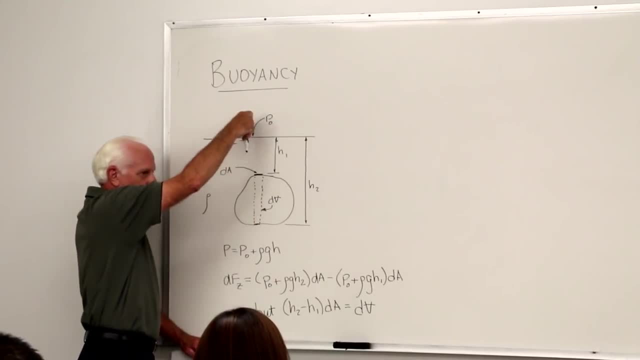 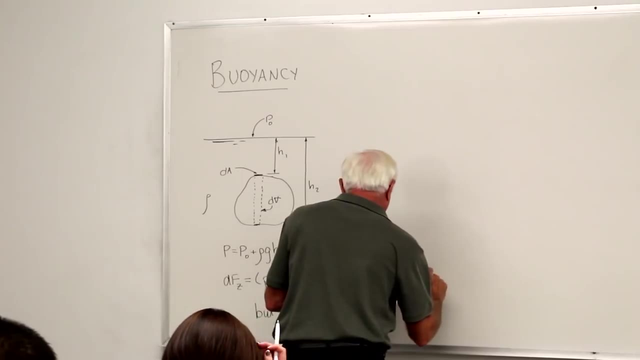 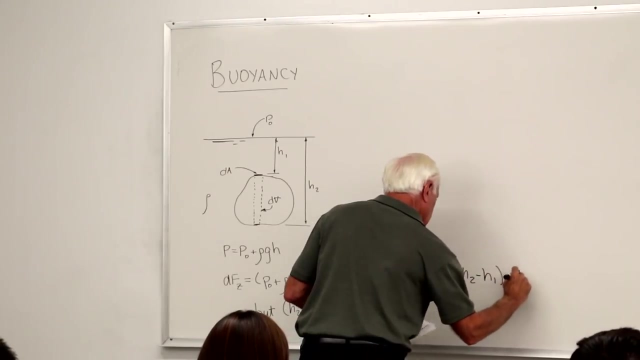 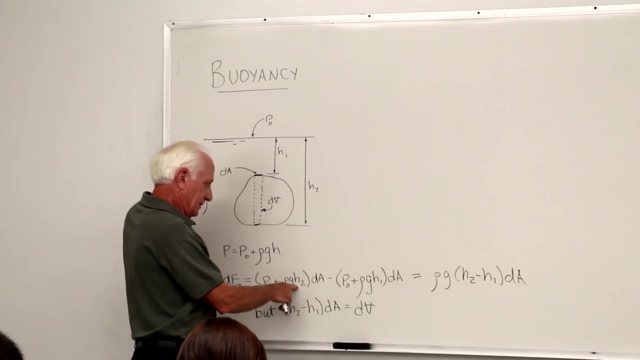 Pressure at the top, minus pointing down Normal stress. Subtract the two, This little piece off here. Subtract the two. The P naughts. cancel out Rho G times. H2 minus H1 times DA, There it is. 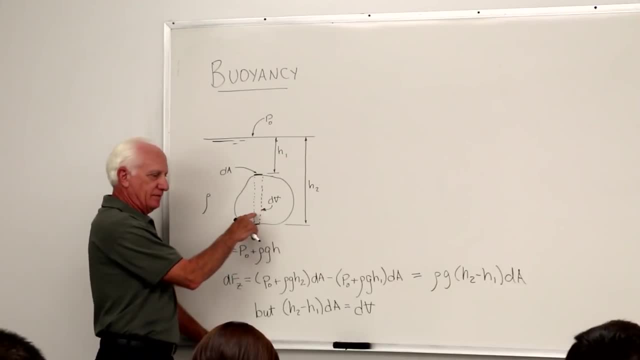 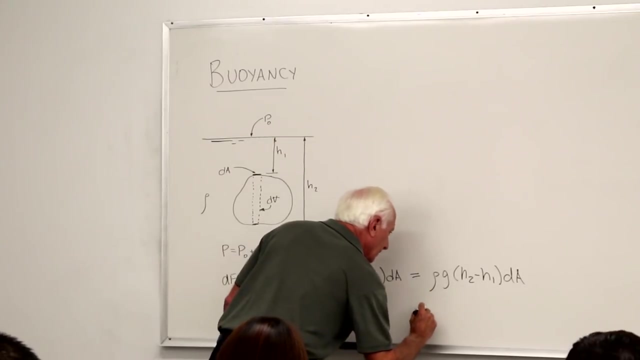 But notice what the differential volume, DV, is. DV, the differential volume, It's the area times the height. What's the height? H2 minus H1. So this is like a differential volume. So replace that with the differential volume. 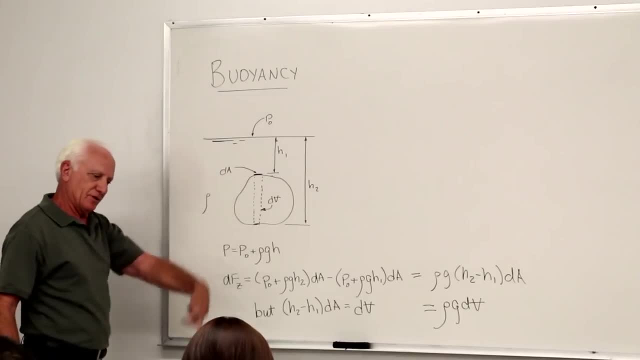 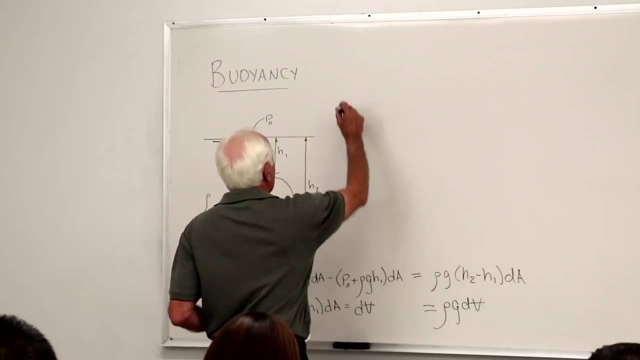 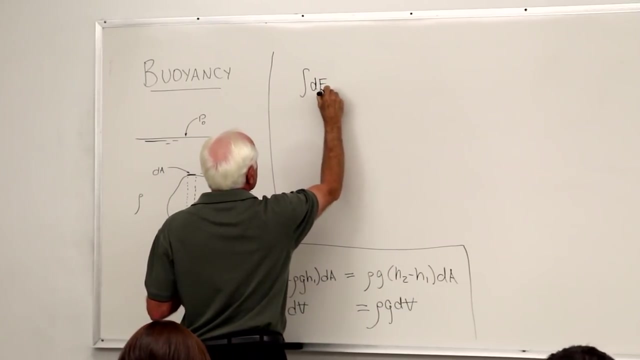 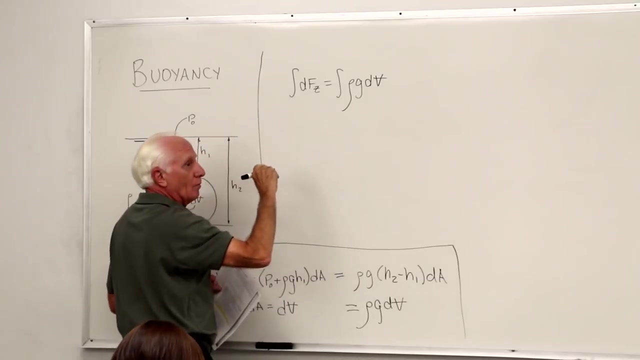 So DF of Z is the Z direction. Z direction is vertically in this picture. The net force in the Z direction equals this guy here. Integrate both sides. Integrate over what? Integrate over the volume? total volume B. 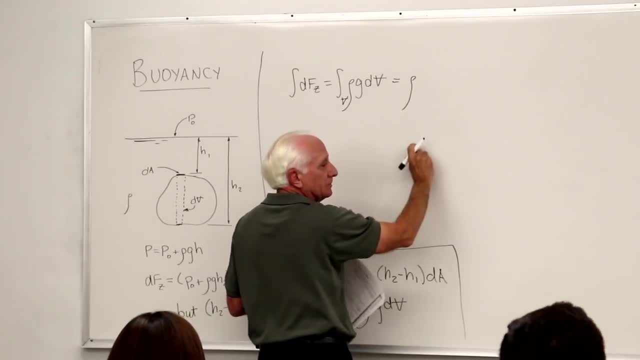 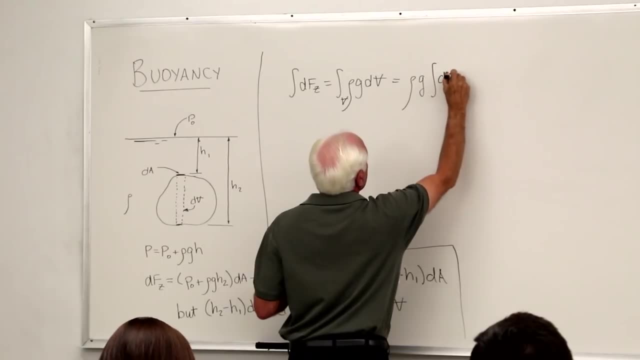 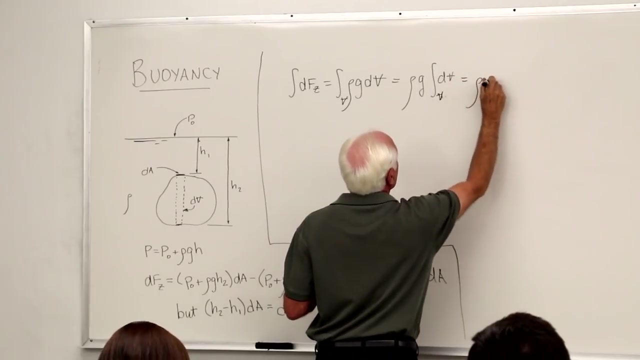 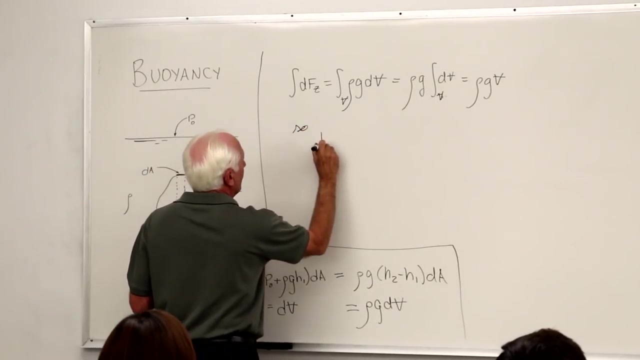 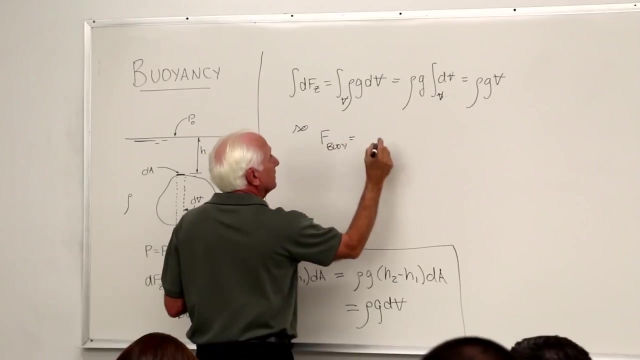 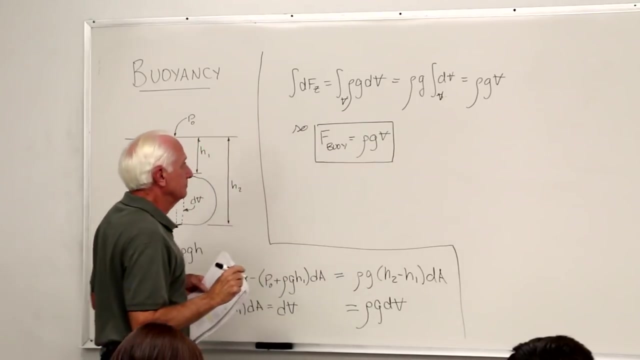 Bring out the constants. We assume incompressible: Rho is a constant, We assume G a constant, Integrate DV over B Over B And we end up with Rho GV. So F buoyancy equal Rho GV. 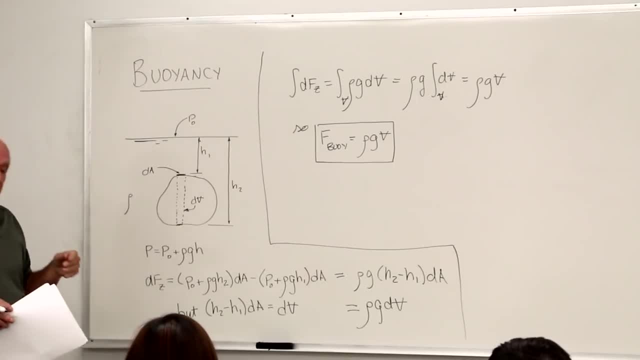 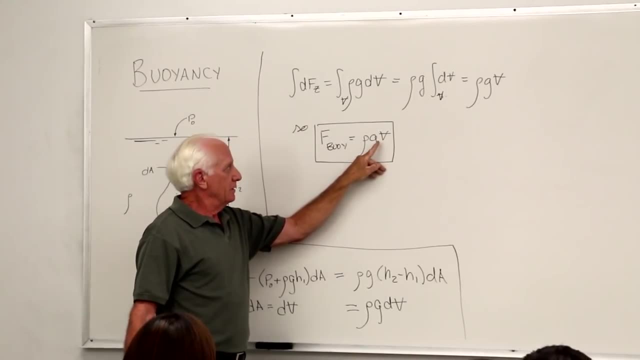 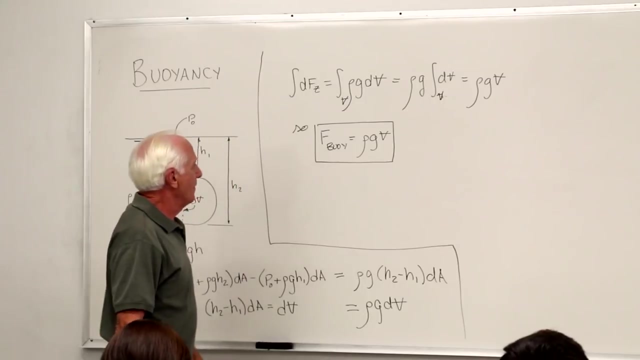 What's Rho G Gamma? What's gamma? Newtons per cubic meter. What's B? Cubic meters? Newtons per cubic meter, times cubic meters, Newtons- Yeah, That supports newtons. Okay, What's the volume? 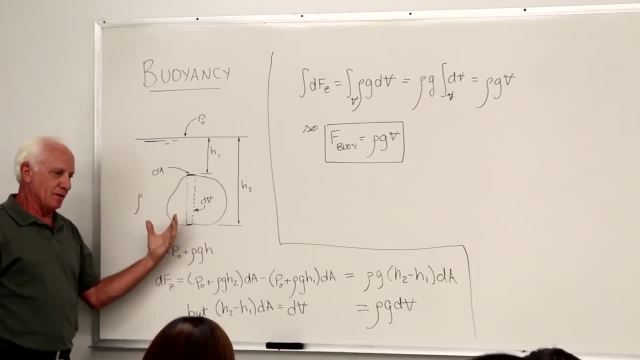 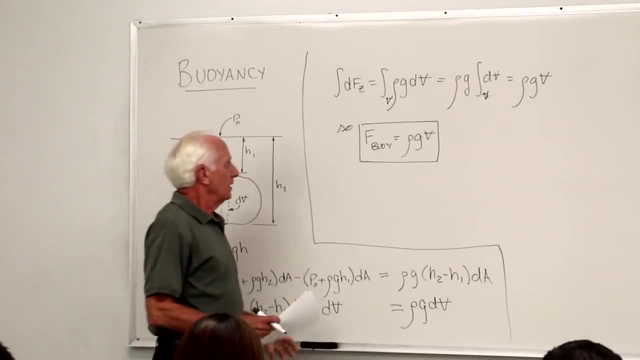 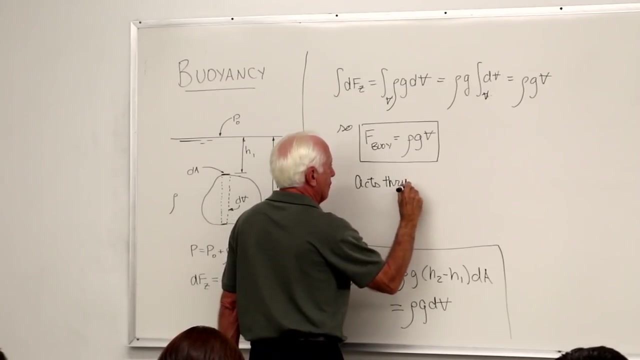 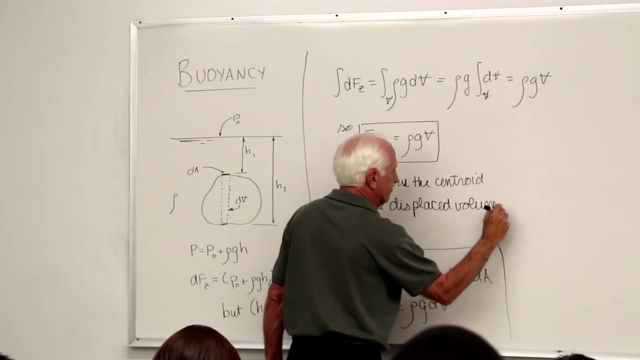 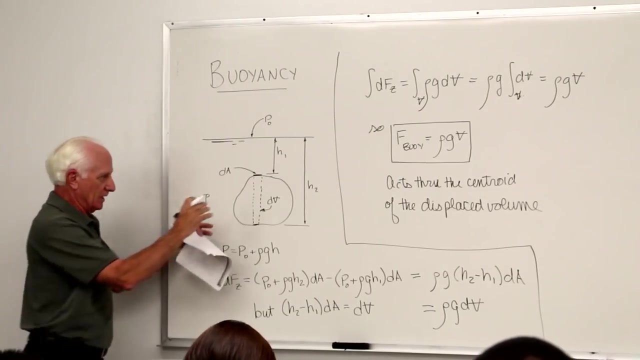 It's the volume occupied by the part of the object submerged into the liquid. Okay, It acts through the centroid of the displaced volume. Through the centroid of the displaced volume. What does displaced volume mean? It means the volume of a liquid pushed out of the way by the object. 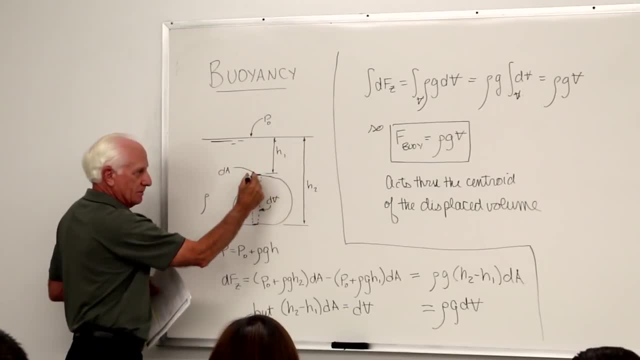 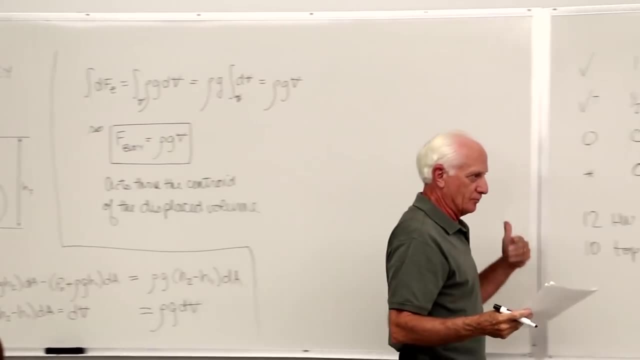 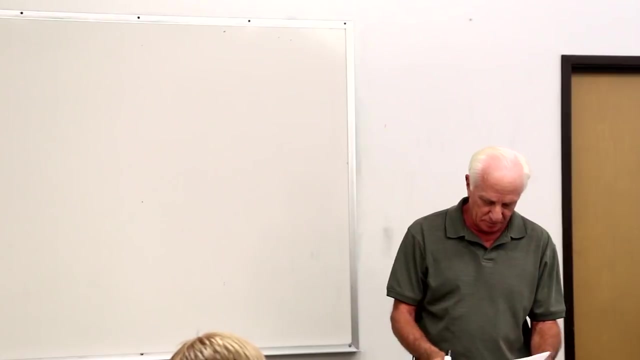 That's the displaced volume. It's this volume inside that line right there. That's the displaced volume. Oh, you can go through the proof just like we did previously. The textbook doesn't do it, They just say it goes to the centroid of the displaced volume. 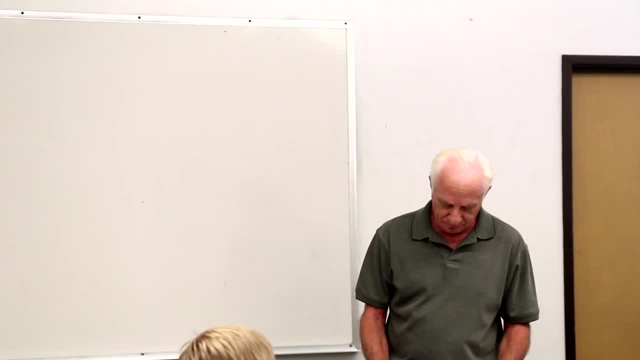 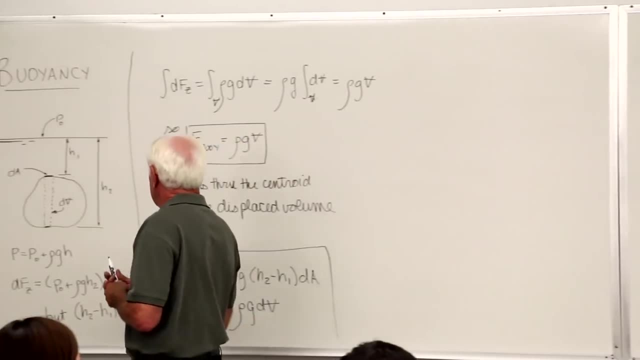 But you can go through all the gory details. Archimedes' principle, of course. Archimedes' principle from science. So which way does buoyant force act Upward? Okay, What does it act through? The centroid of that volume? 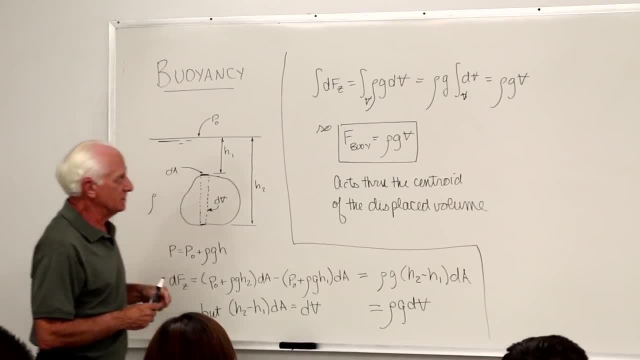 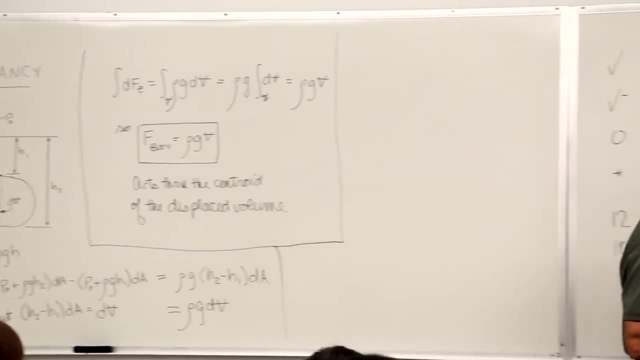 Okay, So that's the concept of buoyancy. You've got a couple of problems for homework on buoyancy. I'll do an example here. Okay, Example, An example of buoyancy. Okay, Okay, Okay, Okay, Okay. 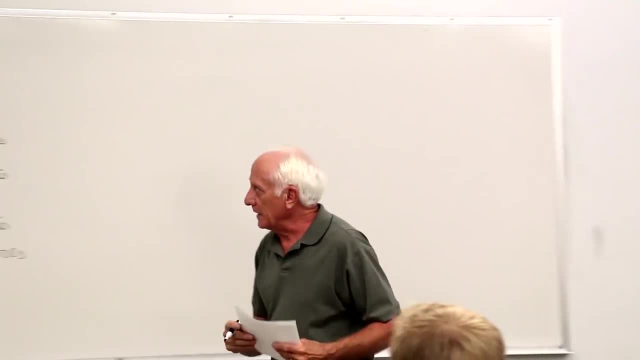 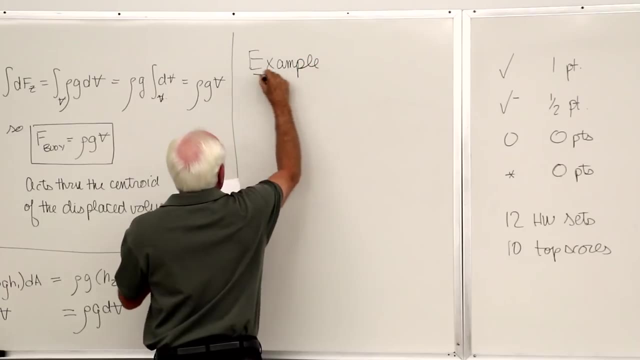 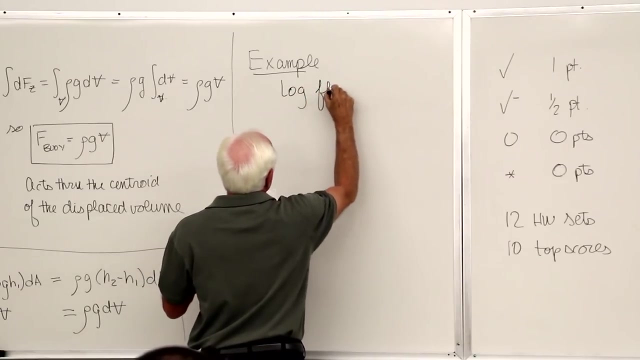 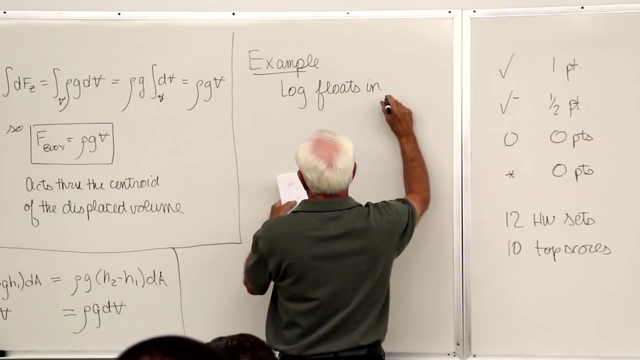 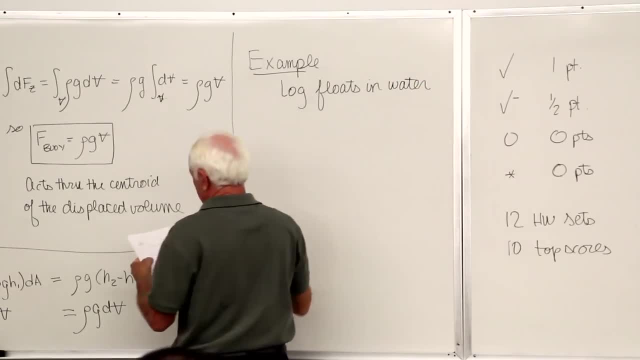 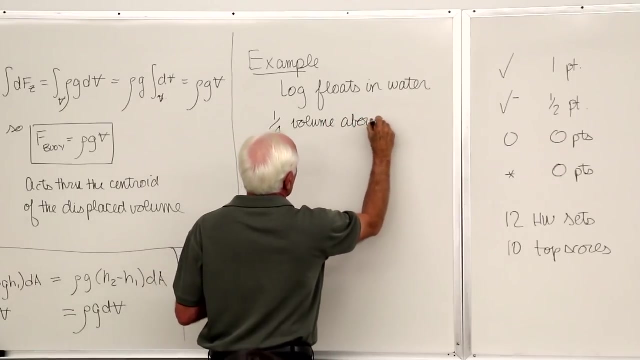 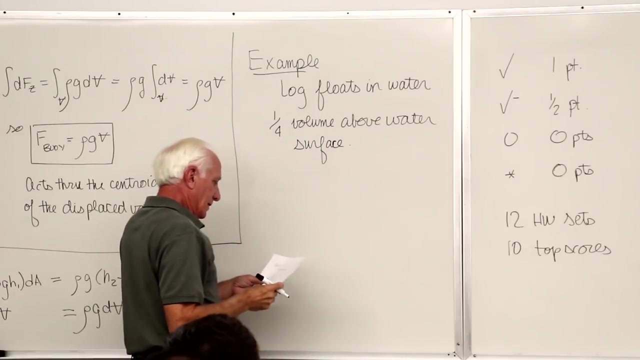 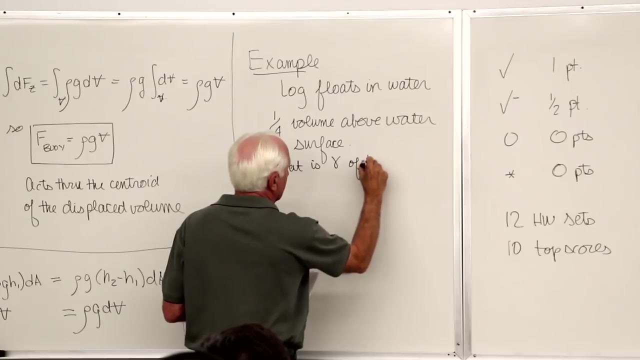 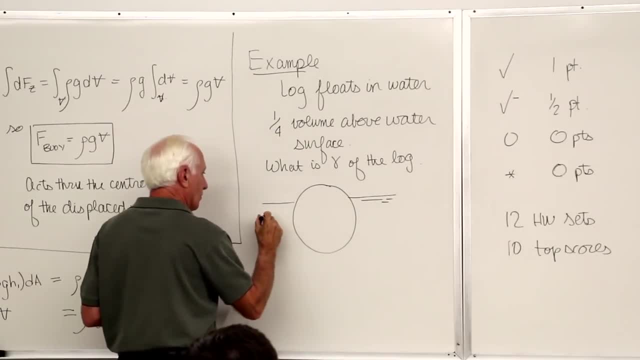 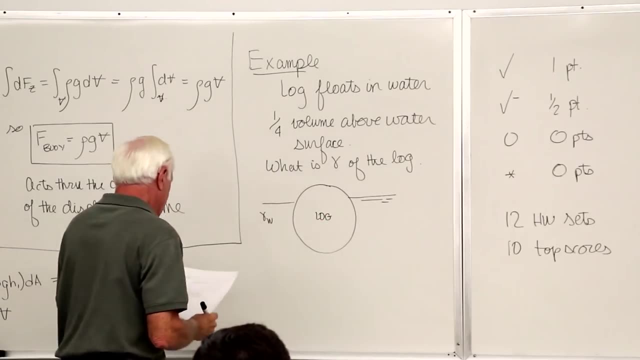 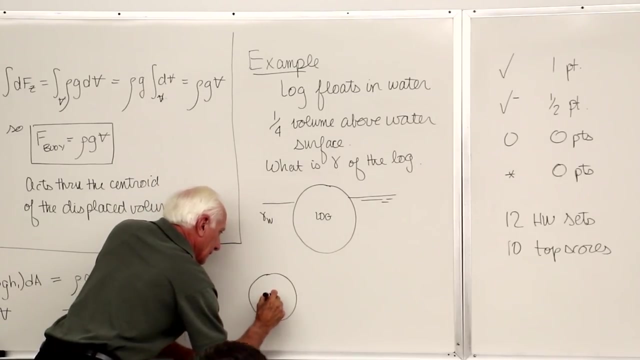 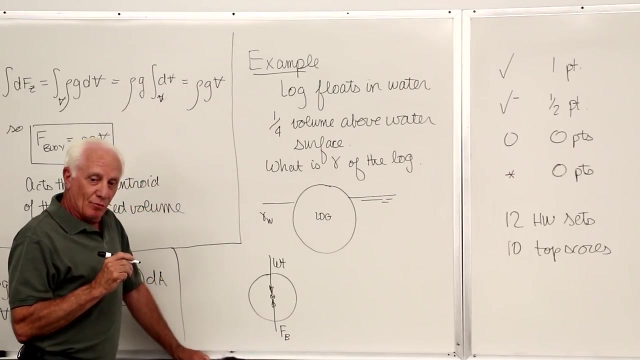 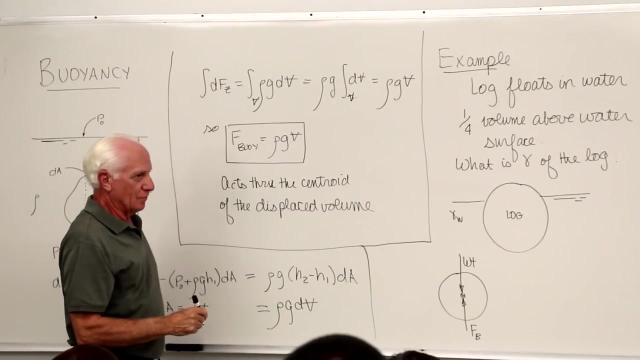 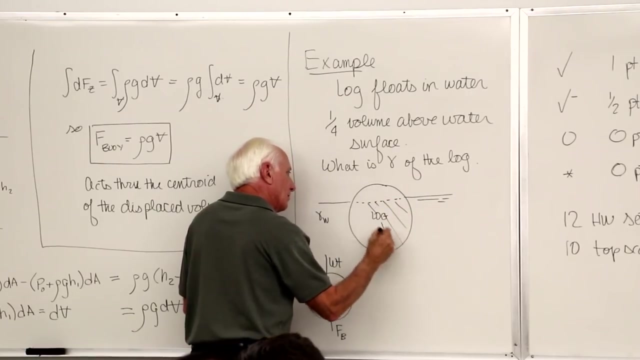 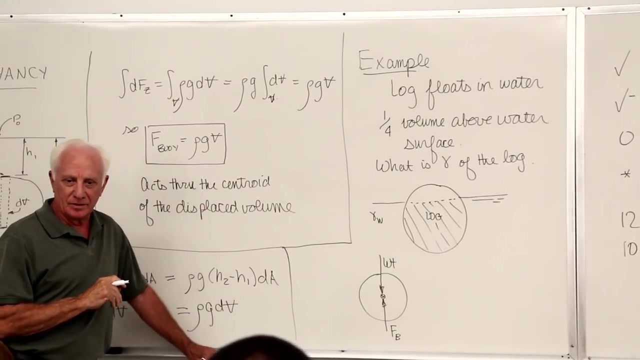 it is protruding above the water surface. draw free my diagram, boy. of course, wait. the weight acts through the center right of the law. the buoyant force acts through the centroid of the displaced volume. where is the displaced volume? that's how much water was pushed on the way when the law went down, the water that's called the displaced bone. 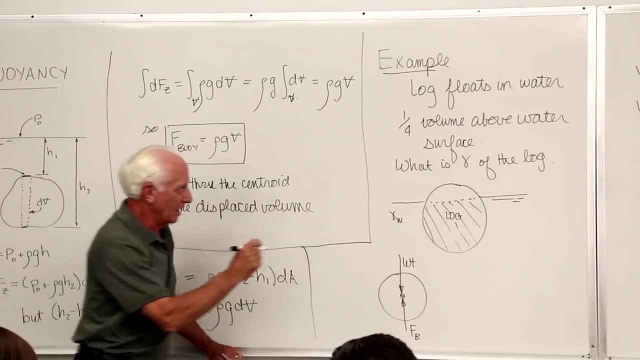 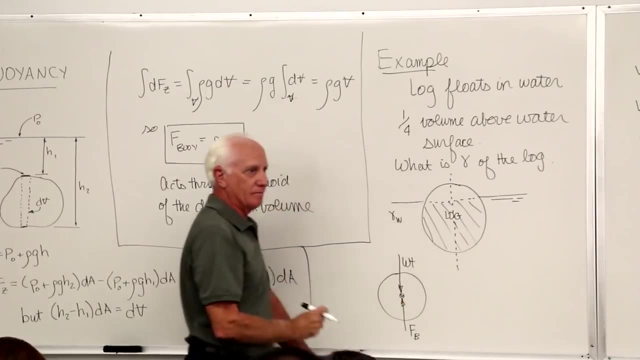 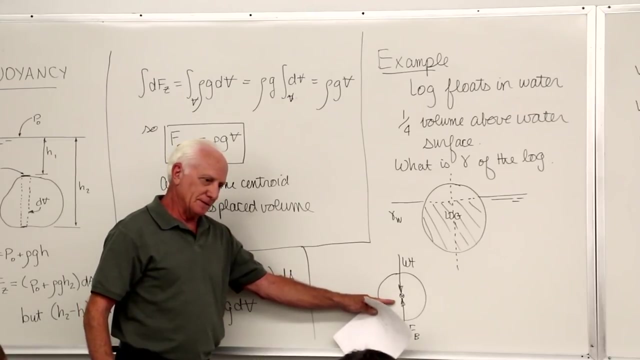 where's the centroid of the displaced volume? right there, somewhere, i don't know up or down right, but i do know it flies along that line right there. that's why i put fb there, acting through, not through that. there's two things okay: the center of gravity and the centroid of the. 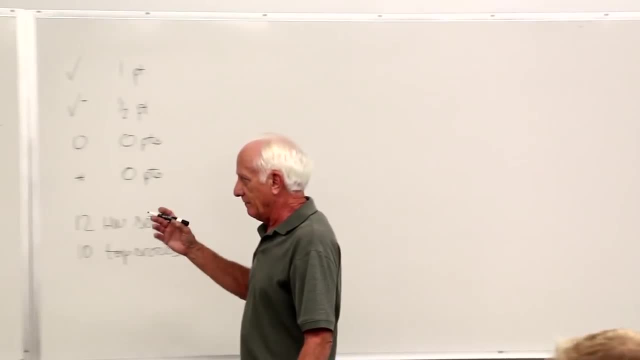 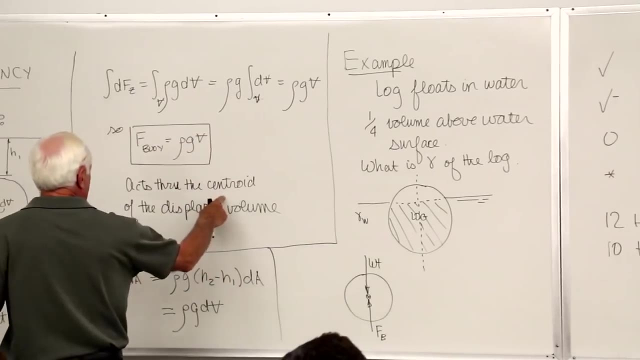 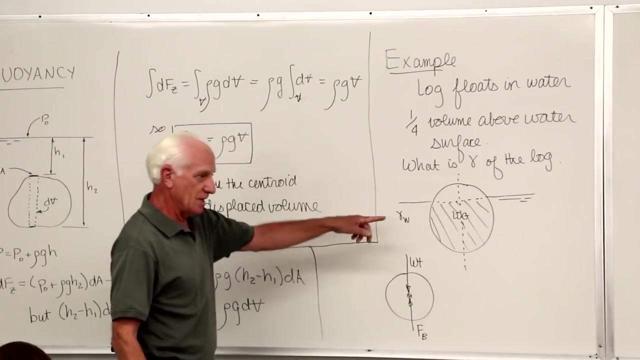 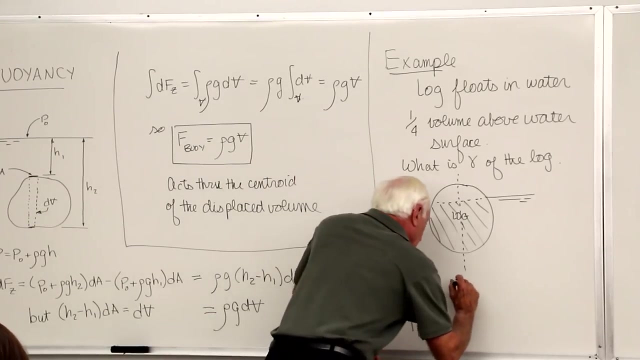 displaced volume. the weight acts through the center of gravity. fb acts through it different place. okay, it acts through the centroid of the displaced line. sometimes they're on the same line, sometimes they're not. it depends on the geometry. anyway, here they are. so some force in the y direction equals zero, the weight equal fb. 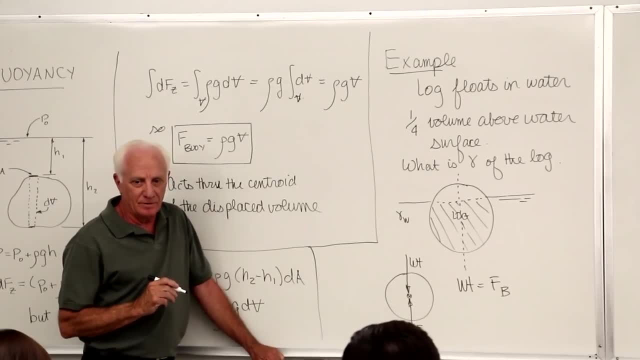 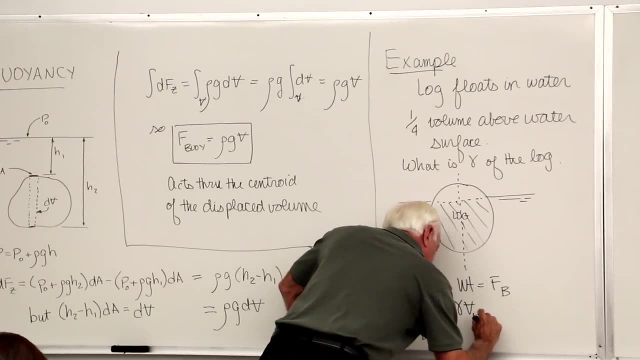 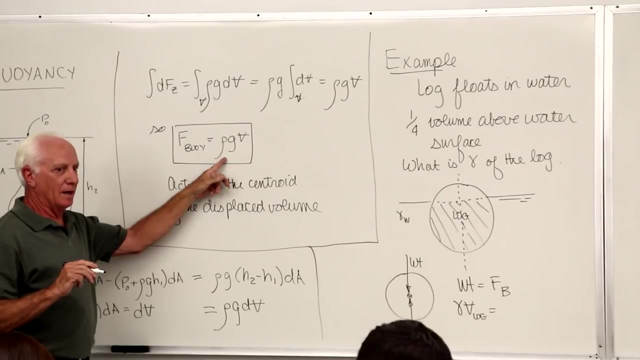 okay, the weight of what, the log, the whole log, of course, the whole log. okay, gamma of the log times, the volume of the law, fb. here it is gamma of what, what you push out of the way water, the volume of what, the volume pushed out of the way, displaced volume. 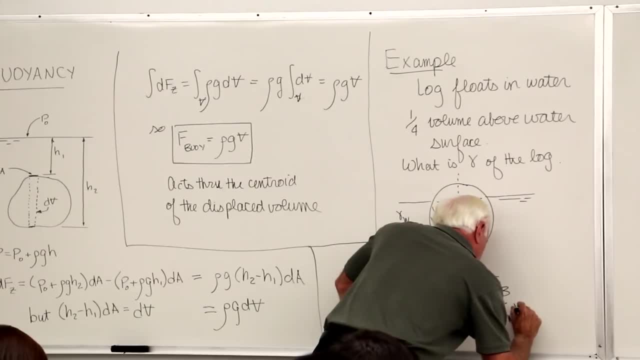 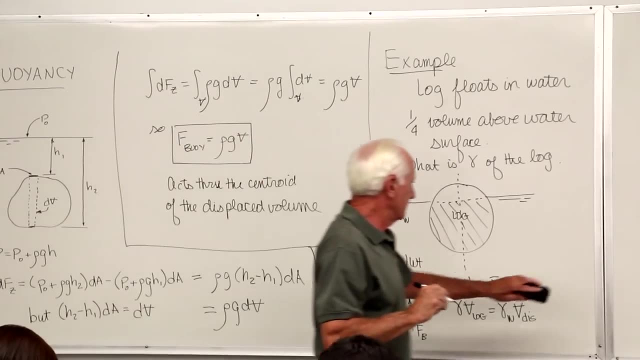 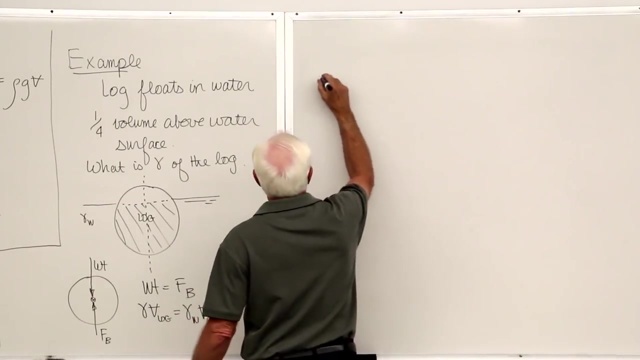 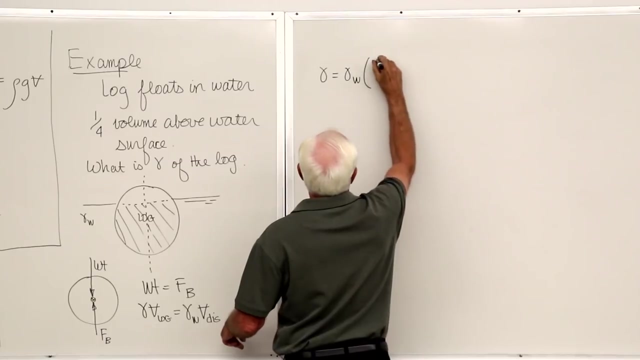 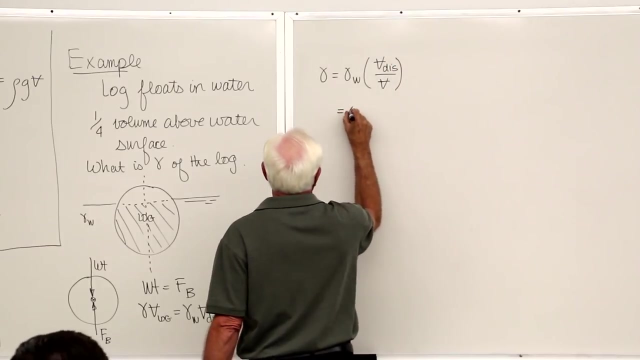 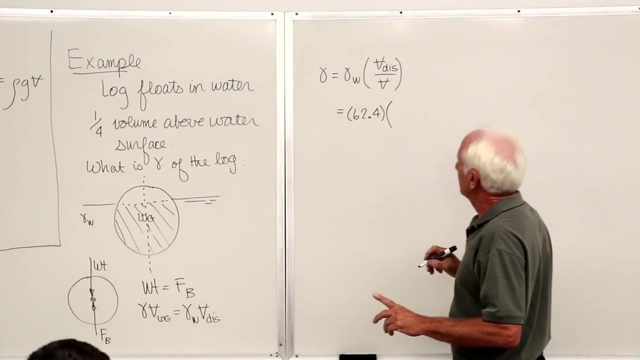 gamma of water times the volume displaced. okay, again, we want to find gamma gamma equal gamma water times the ratio volume displaced over the volume of the log: 62.4 pounds per cubic foot. now you have to be careful, of course. where's the displaced volume? that's the line volume here, the 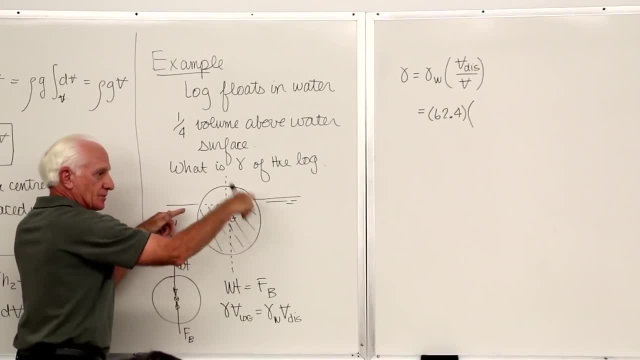 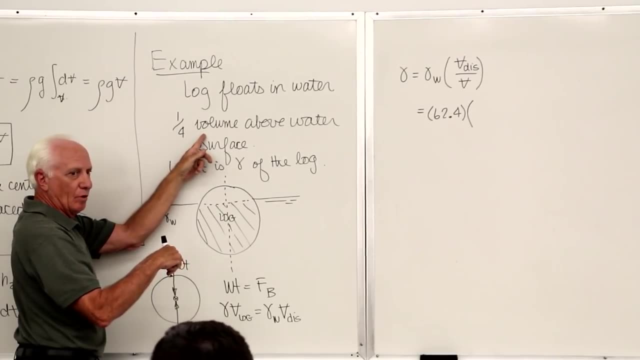 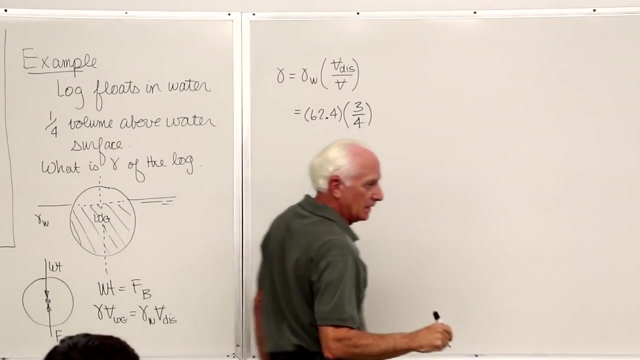 line volume. where's the volume of the log? that's the circle. that's three-fourths. one-fourth is above water. three-fourths is below water. three-fourths is below water. displaced line ratio: three-fourths, which comes out to be 46.4 pounds per square foot. 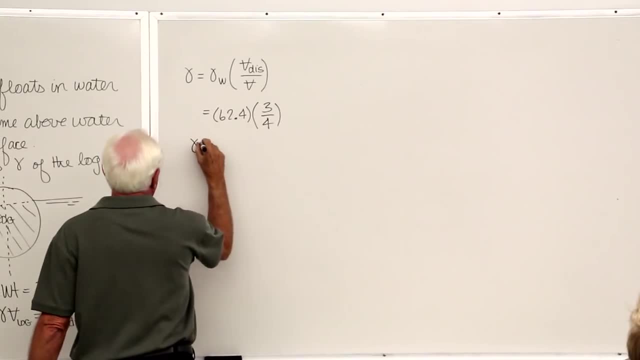 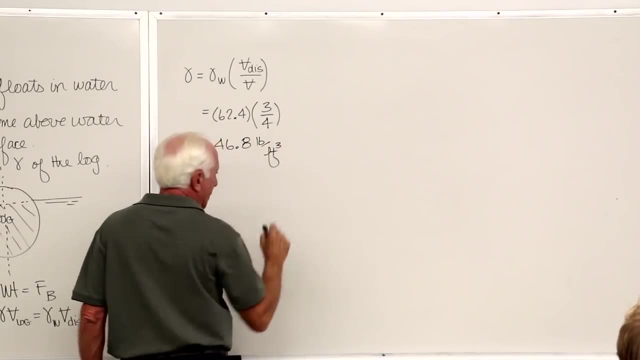 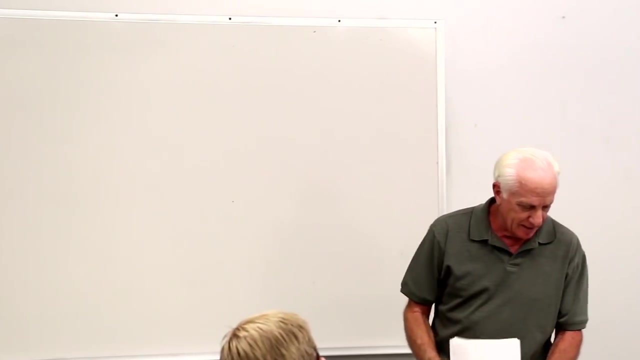 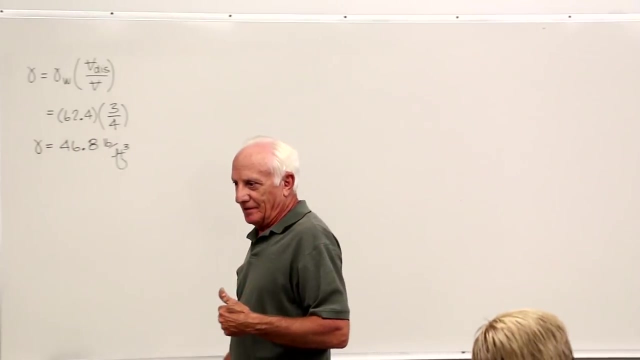 to be 46.8. okay, so you should be able to work the homework. uh, it's pretty straightforward. on that topic, you can also get into what we call stability, when something might tip or not tip variable: too many people on one side of the top deck or something, and it's a wave that goes over it. 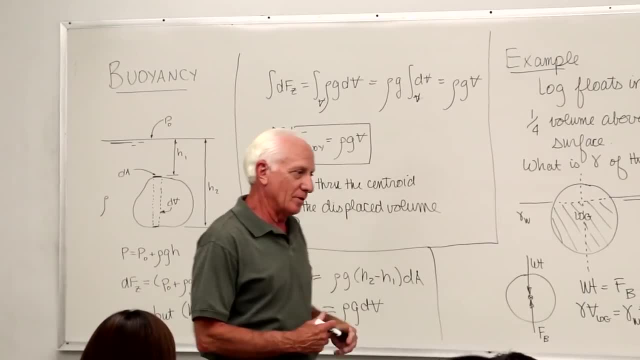 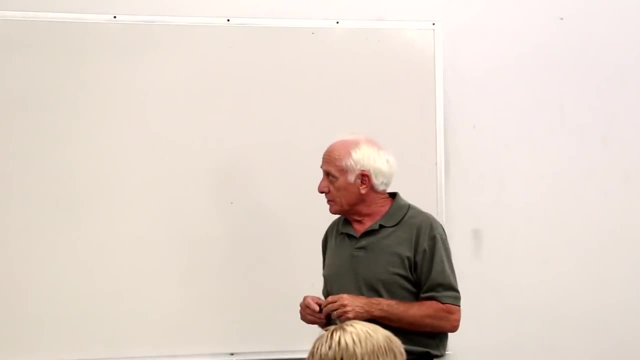 i want to come back and write itself. well, that is part of the point, of course, but there's no homework problems on on stability, so they're just on the white horse. okay, that pretty much wraps up chapter two. it's pretty long we've been in this chapter, since the 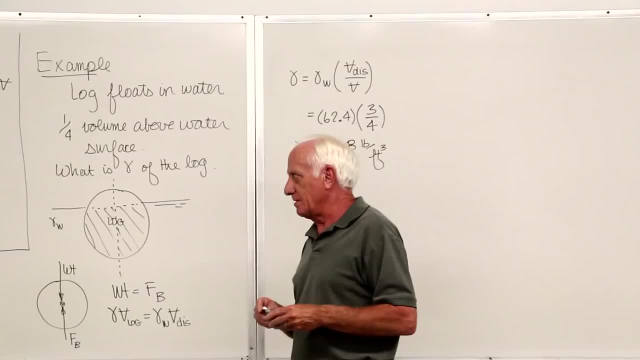 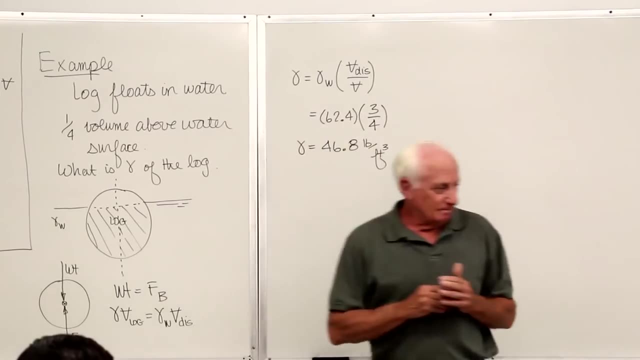 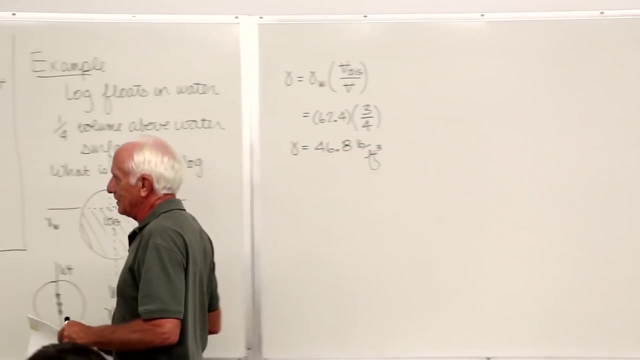 second class meeting about. so yeah, it's pretty long. that's why that first midterm includes chapter one, chapters two, because two is such a big long chapter. okay, now, let's, we're gonna move on to chapter three, but we're not going to have any of chapter three on the first midterm. 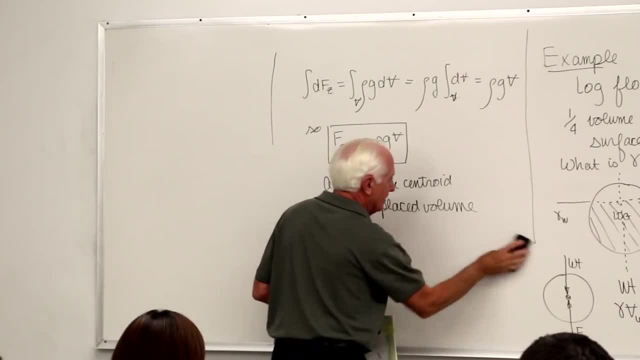 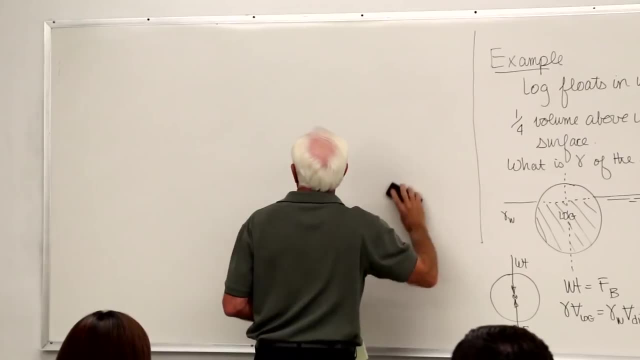 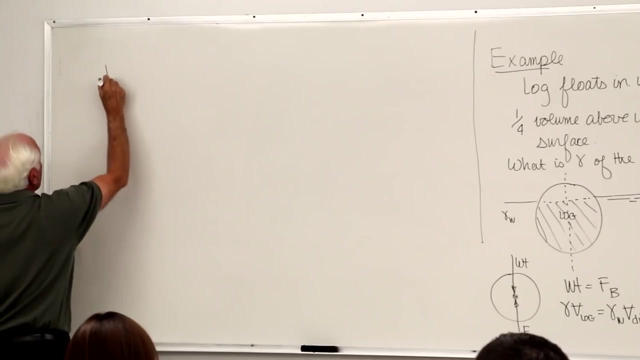 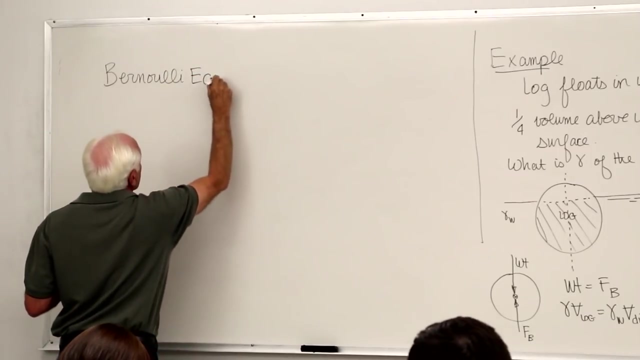 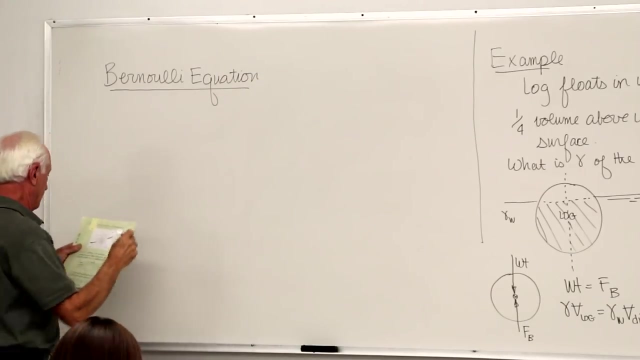 some people cover the material in chapter three. later i'm going to follow the textbook on this one, so we'll follow what's in your textbook and we're going to uh, look at the bernoulli equating. all right, i'm going to start off and uh, 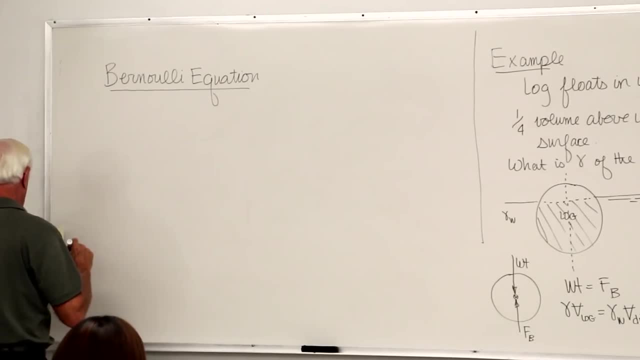 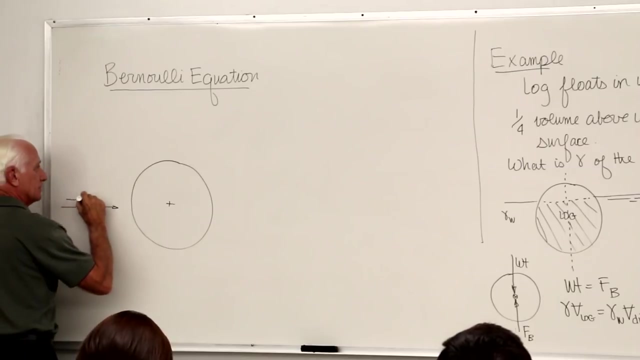 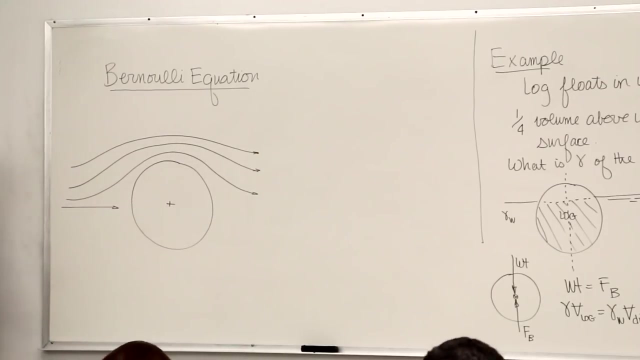 maybe we'll define a streamline first. okay, so here is uh, some cylindrical object and we have flow around the object, so it goes around like this. i won't draw top and bottom, i'll just draw the top, the bottom symmetrical. this is like a piece of pipe in an airstream. 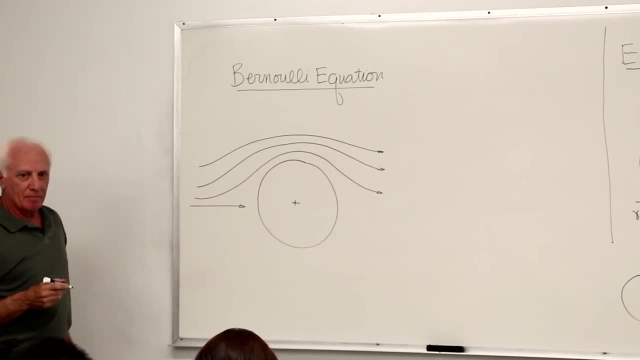 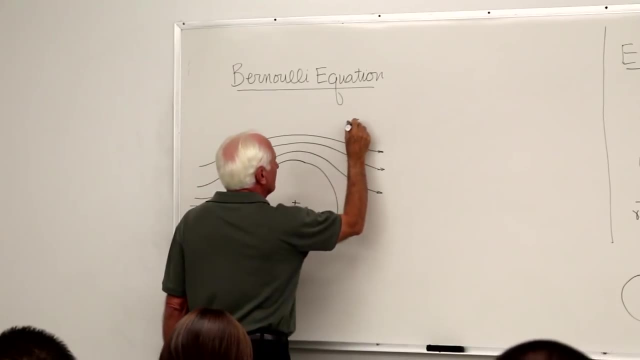 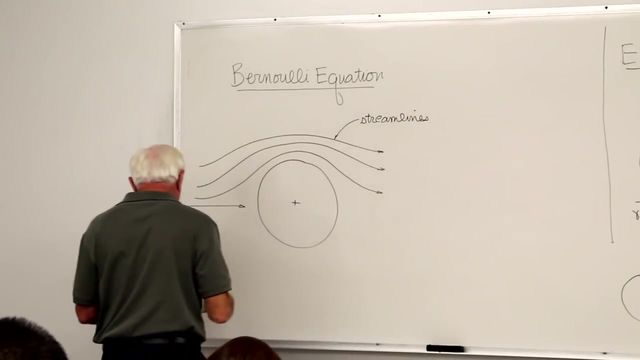 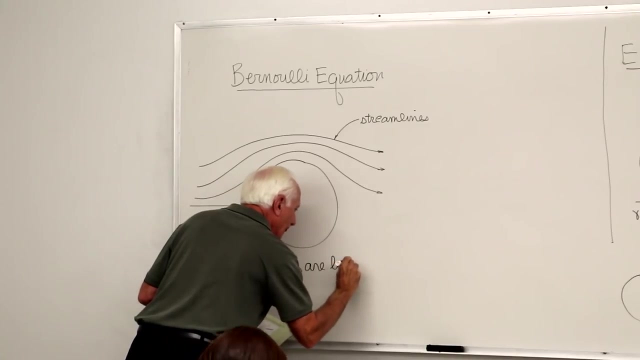 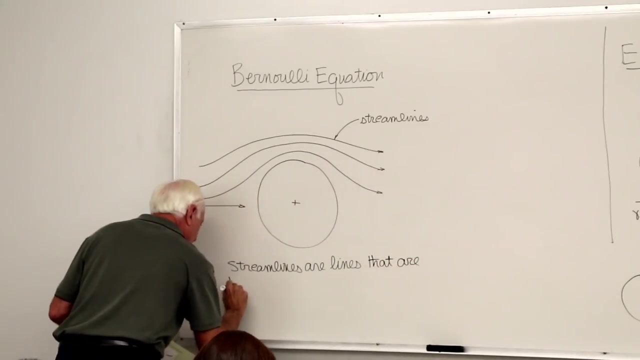 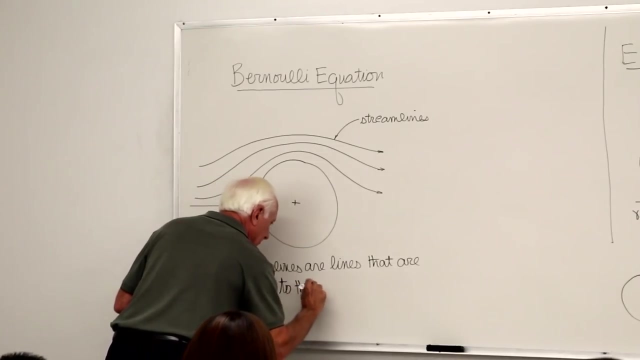 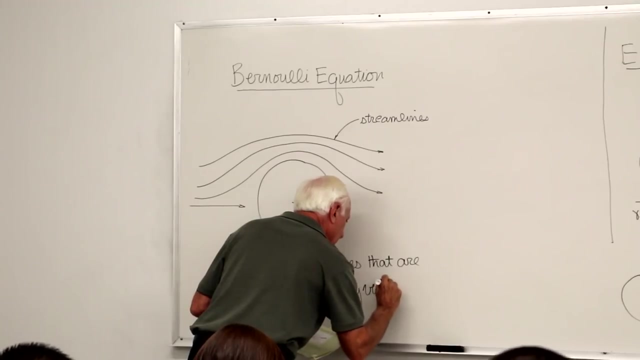 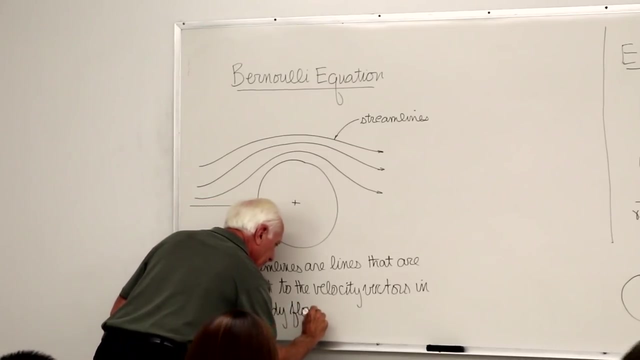 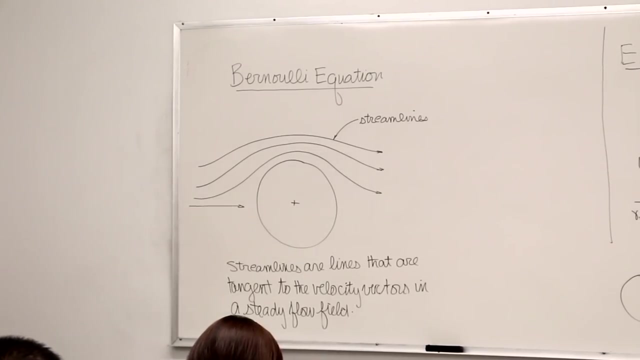 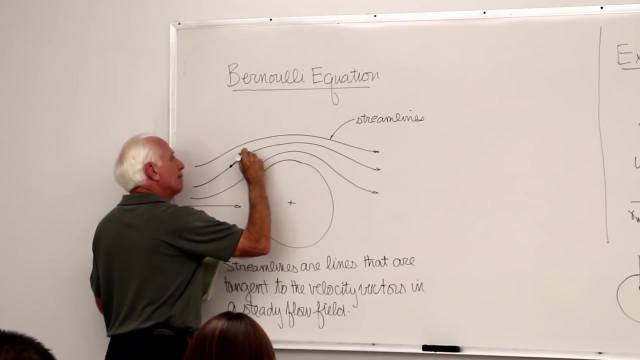 and the top is like a funnel. when people draw pictures like this, these lines they draw are called streamlines definition, the official definition Tomorrow. Okay, that's the definition of the streamlines. So here's the velocity vector at this point. Here's the velocity vector at this point. 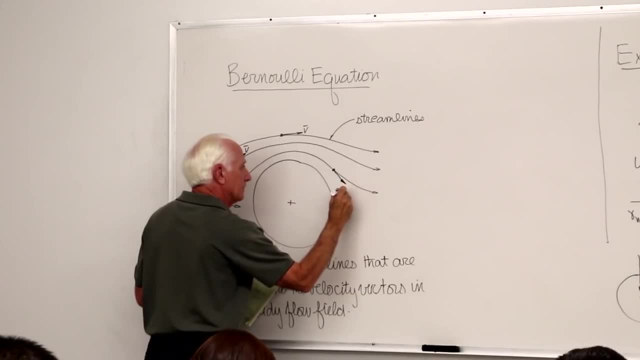 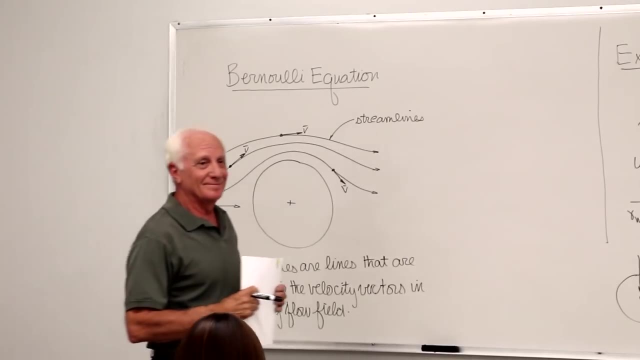 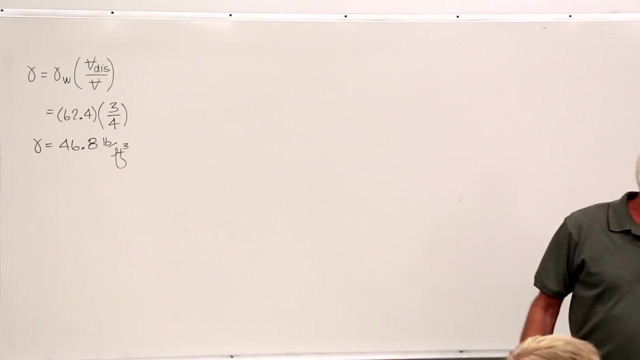 Here's the velocity vector at this point. Well, you can see what we're doing, You. okay, man? Okay, The streamlines are lines. I mean you can see the streamlines are lines. I mean you can see the streamlines are lines. 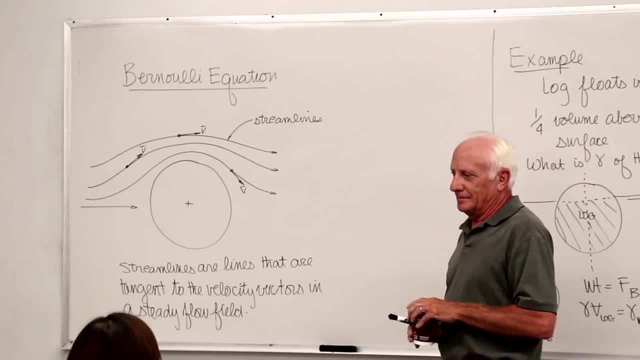 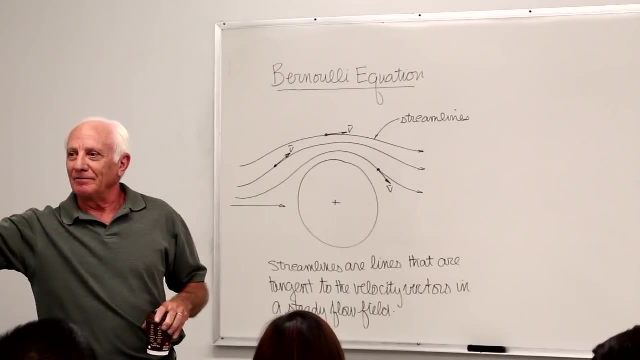 I mean, do you see them in the real world? Of course not. no, Sometimes you do. You've seen the ads for cars in a wind tunnel with smoke and you'll see the streamlines go around the car, follow the back contour and they break off in the back. 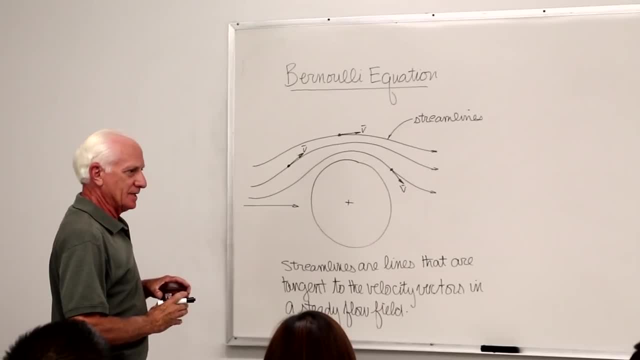 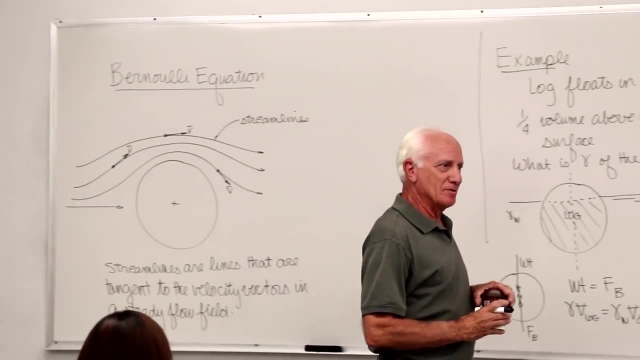 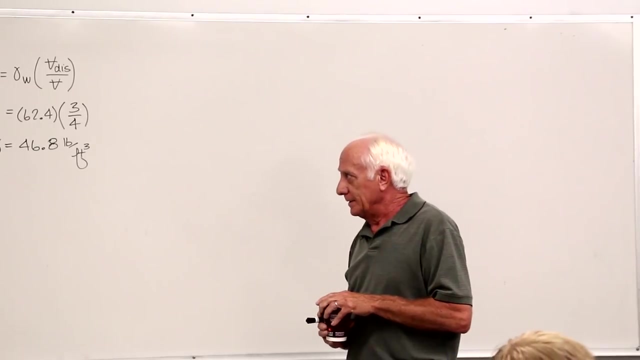 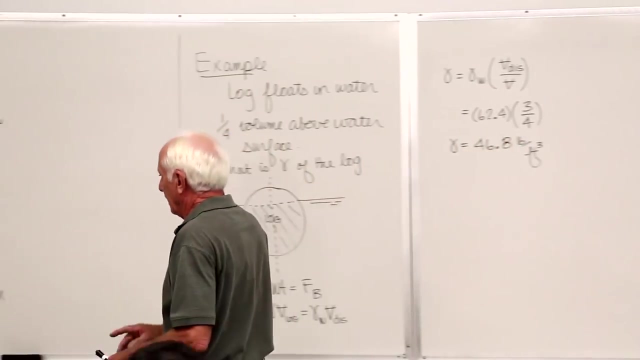 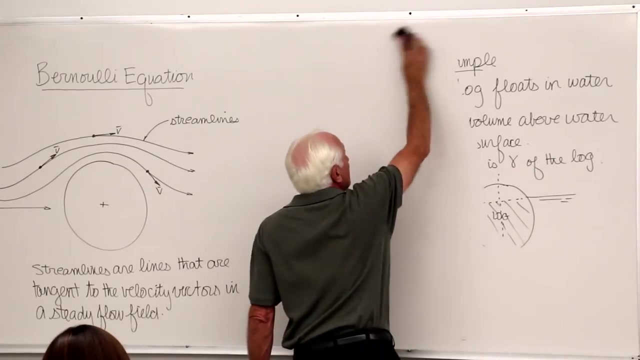 Those are streamlines in steady state, So we can't see them by adding smoke or hydrogen bubbles to a liquid flow field or smoke to a gaseous flow field. But that's what they look like. That's their official definition. We'll talk more about streamlines and pathlines and streamlines later on. 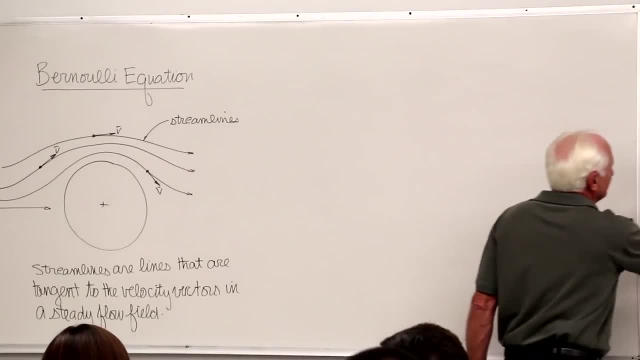 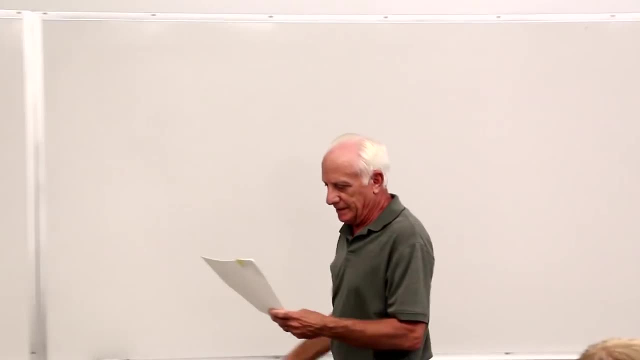 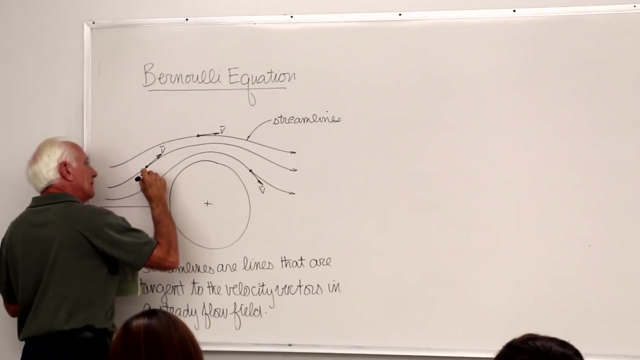 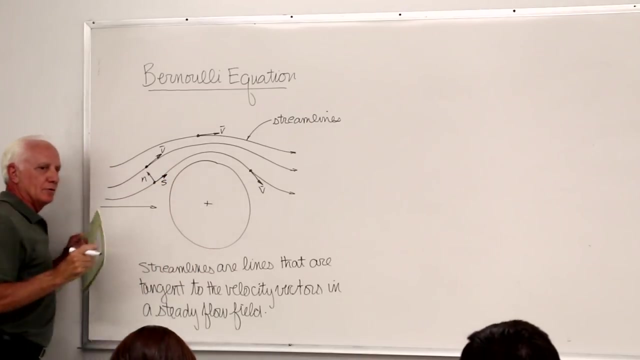 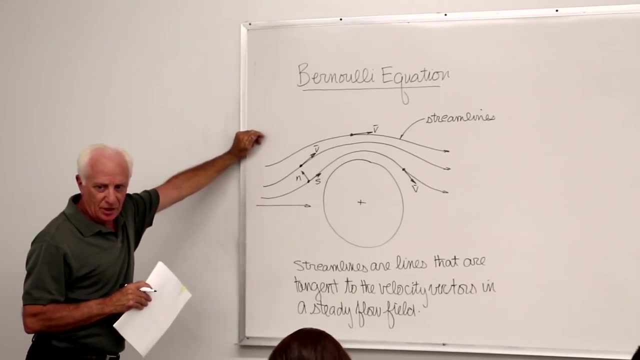 But for right now we're just concerned with streamlines And we're going to define N and S. N means normal N direction, S means along the streamline direction, So we attach our coordinate system to the streamline, So S is along a streamline. 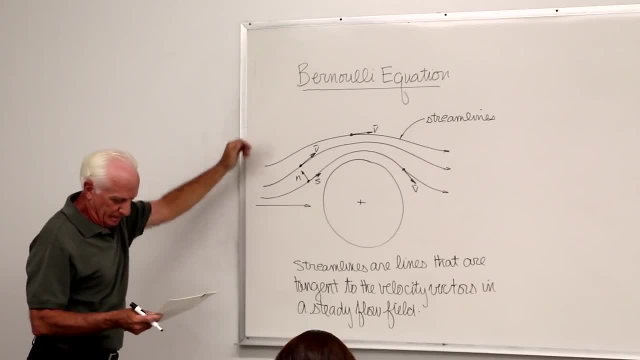 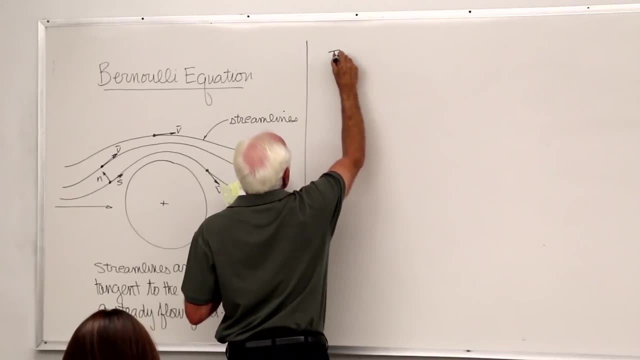 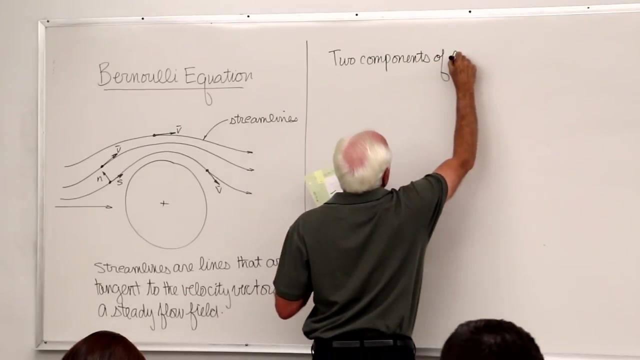 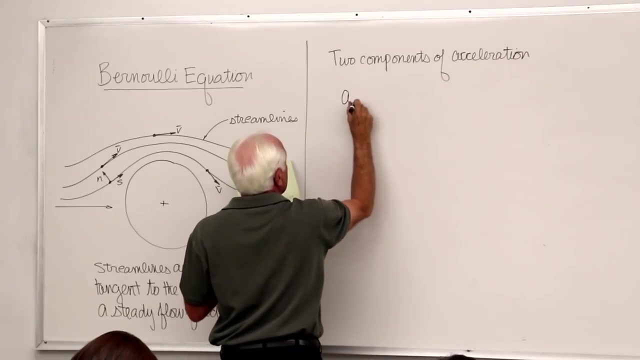 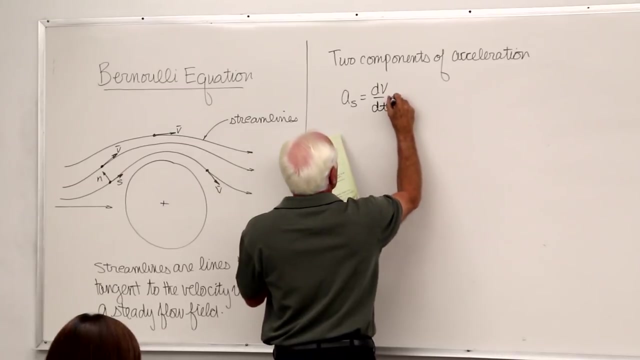 N is normal to the streamline. So we have two components of acceleration: A sub S, D, B, D, T. partial B with respect to S, partial S with respect to T product growth. partial B with respect to S, partial S with respect to T product growth. 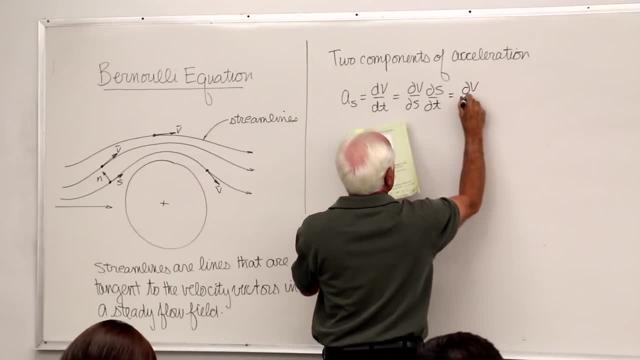 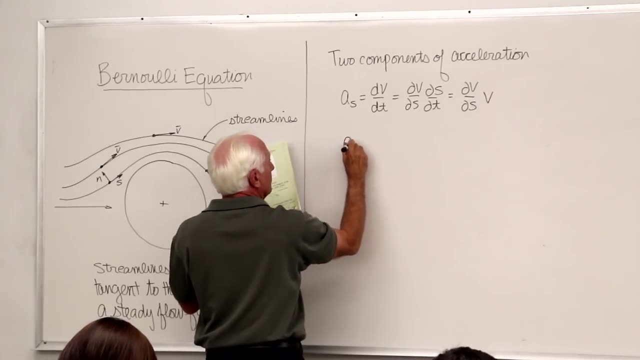 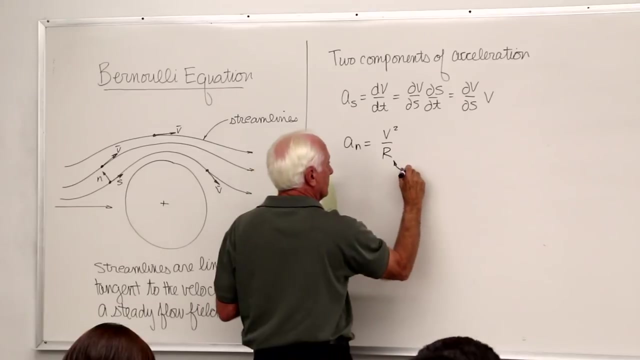 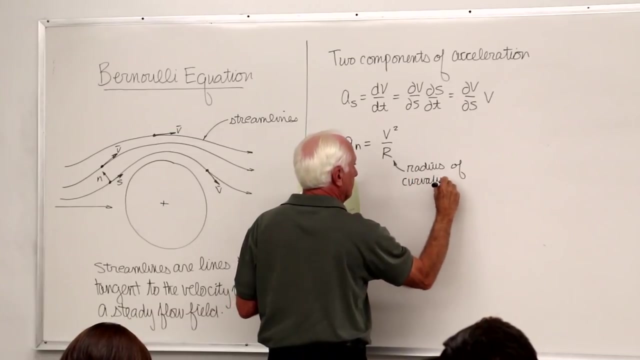 D, B, D, S And, of course, D S, D. T is just the velocity And the normal acceleration, B squared over R, where R is called the radius of curvature. We're going back to our dynamics background. 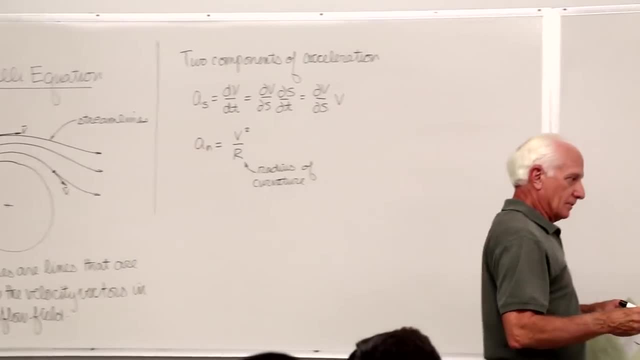 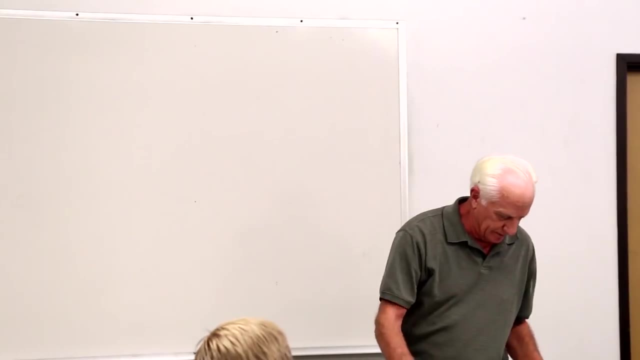 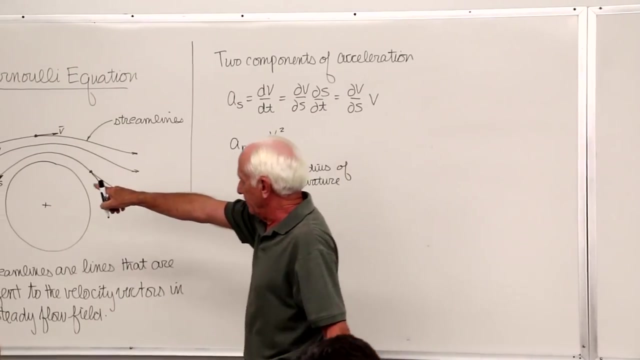 We're going to compare these two guys. So we're going to compare these two guys. You can have both a streamline acceleration and a normal acceleration. We're going to take a streamline out of here. I'll take one over here maybe. 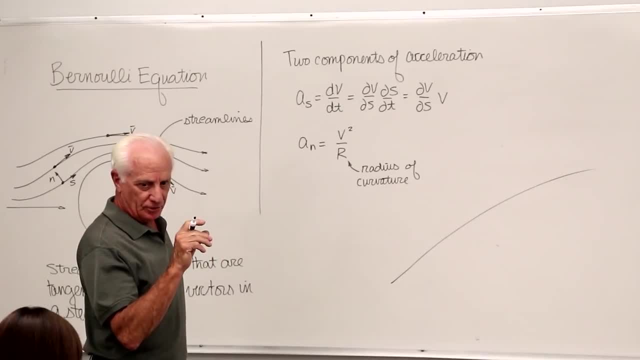 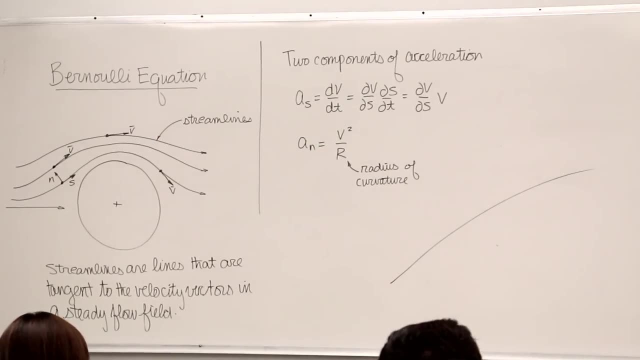 So here's a streamline And on that streamline we're going to show a very small differential volume of, let's call it, a little bit of mu. So let's call it a little bit of mu liquid. so picture, right, I'll go to the picture like it's in the textbook, so you 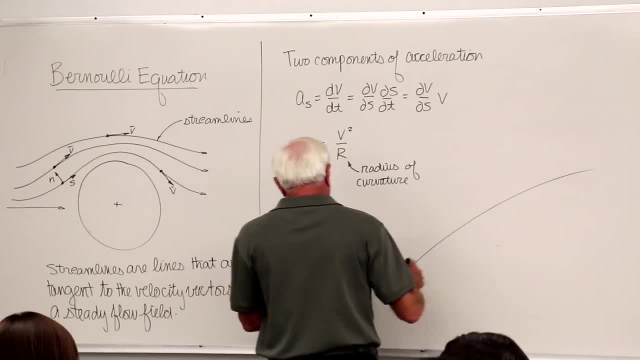 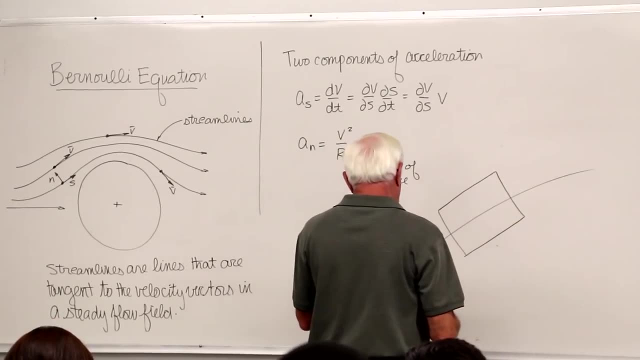 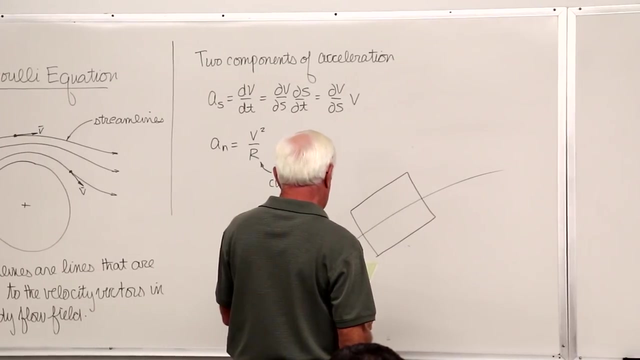 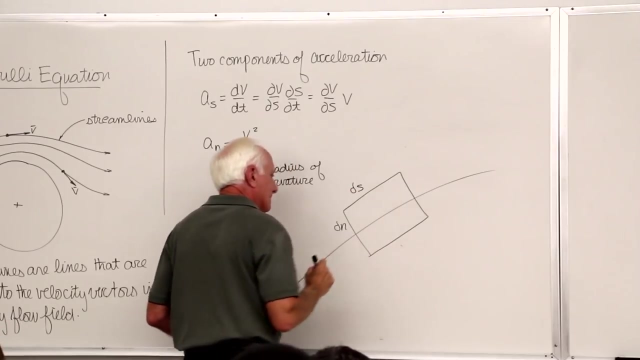 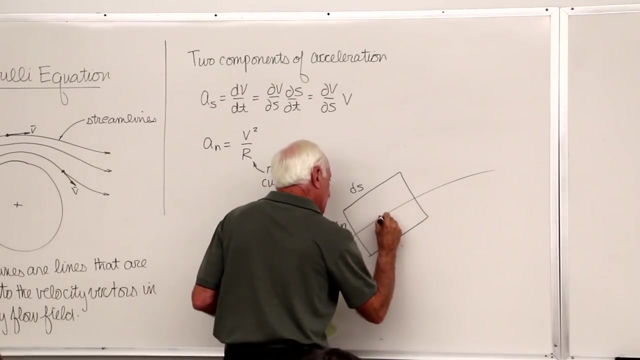 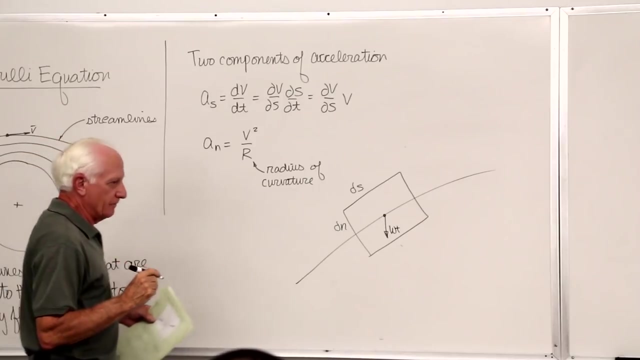 can follow it okay. so we have our little differential element and let's see, we're defining Delta s this way and don't. so here's Delta n, use Delta s and we have the weight of that little differentials element acting down and there's a pressure force on the left. 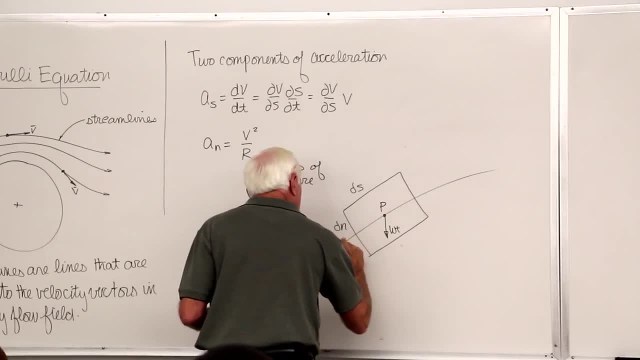 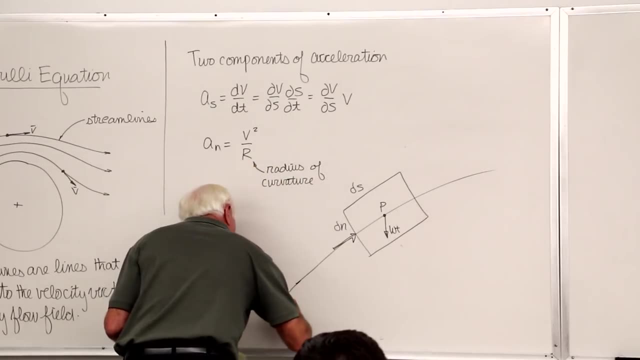 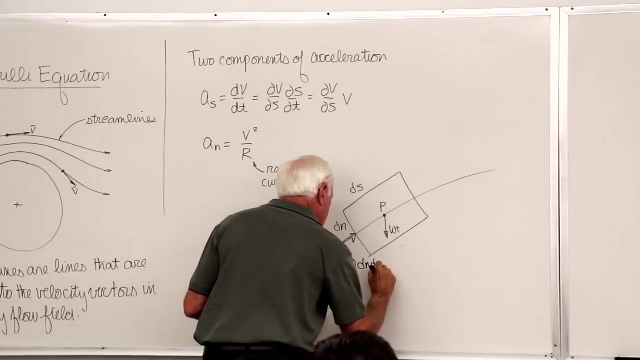 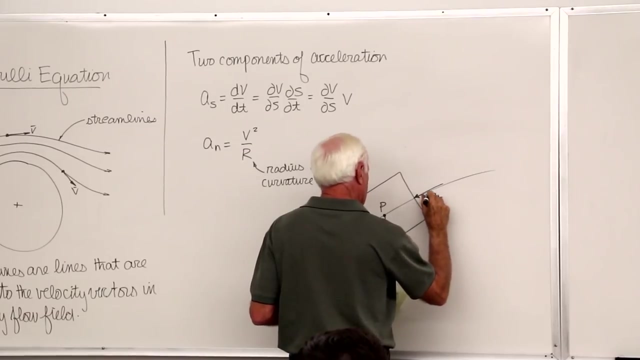 so this is: the pressure in the middle is P the pressure on the left, the pressure on the left, P minus DP. multiply by the area P n dy. The pressure on the right side is p plus delta, p dn dy. dn dy is the area over which the 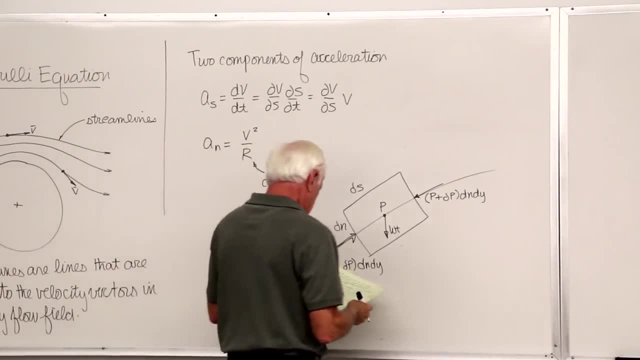 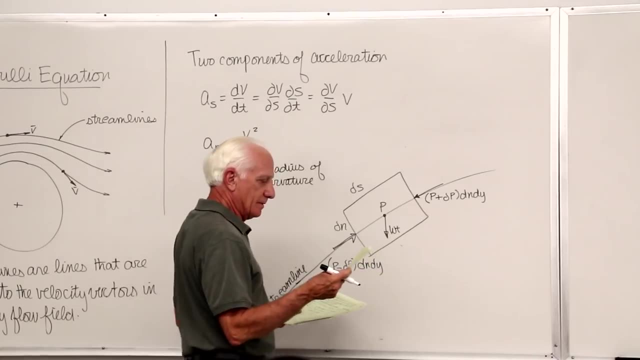 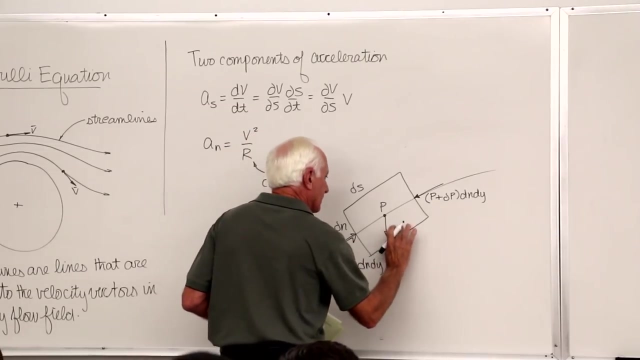 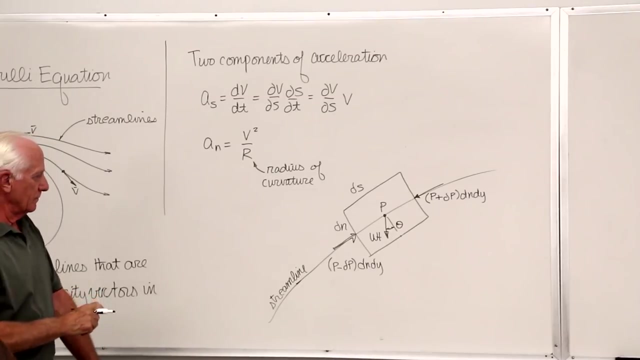 pressure acts and I think that's all we've got in there in that direction. yeah, make sure. yeah, let's get the angle theta. there's the angle theta. we'll need to get the angle theta. we'll need to get the angle theta, we'll need that. so we're neglecting the viscous effects. no viscosity, otherwise. 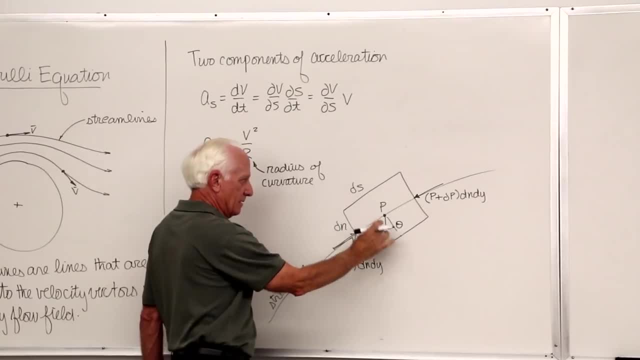 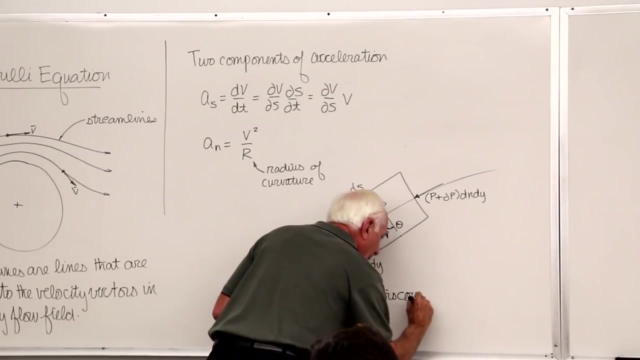 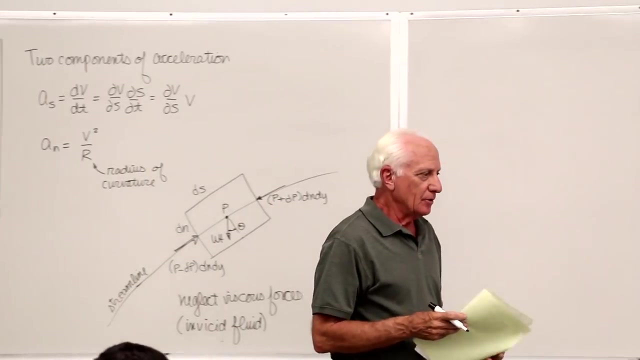 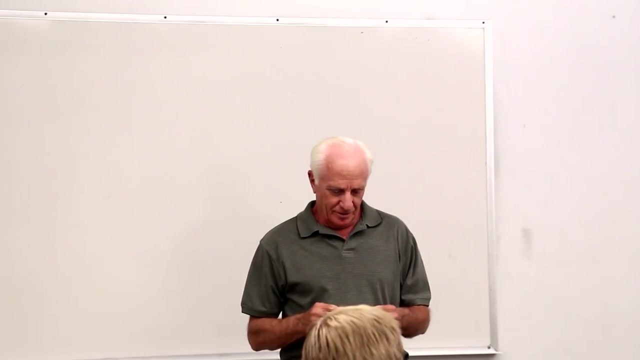 viscosity would act on these surfaces. here we're neglecting viscosity, so put that, put that down. we call that kind of fluid where we neglect viscosity, we call that an inviscid fluid- inviscid. so if you see some words on exam, you know what viscosity means. 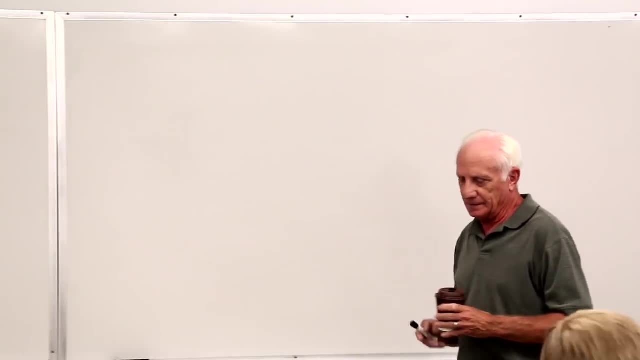 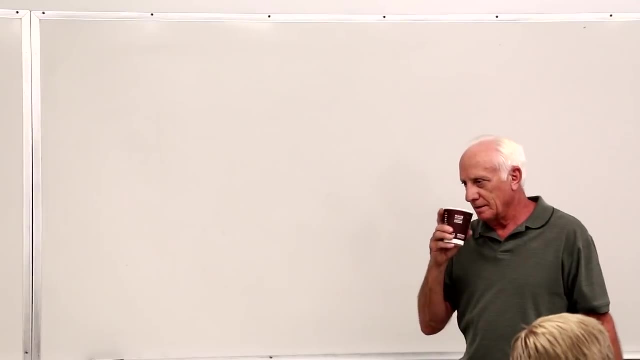 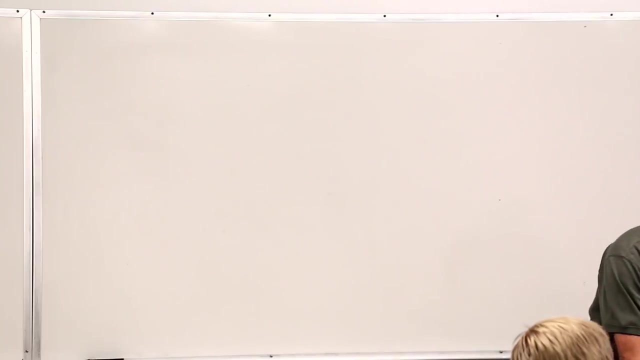 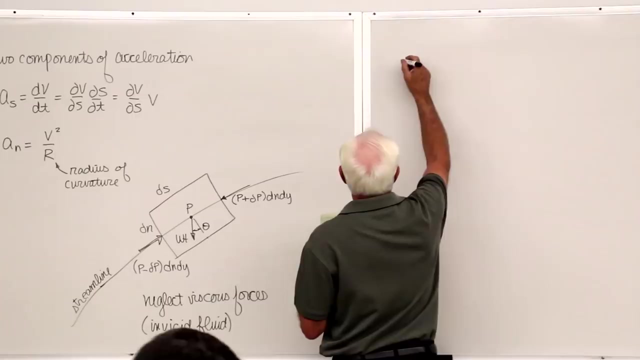 what they mean. inviscid, neglect, viscosity, incompressible densities, a constant you can quote outside the interval sign. okay, inviscid fluid: all right, so let's write the sum of the forces in the s direction. all right, so let's write the sum of the forces in the s direction. 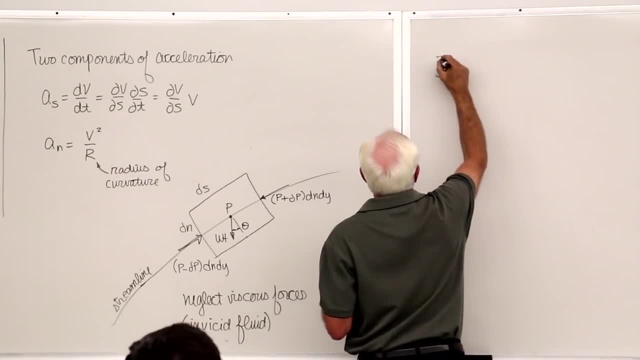 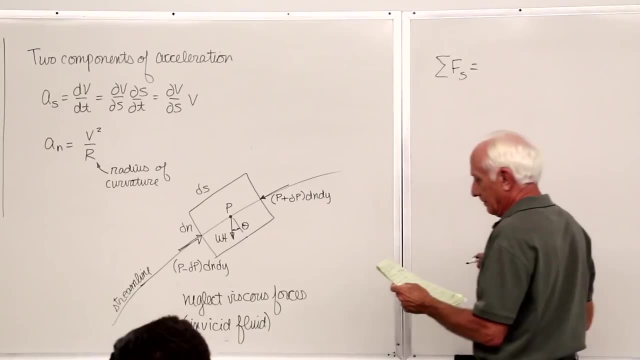 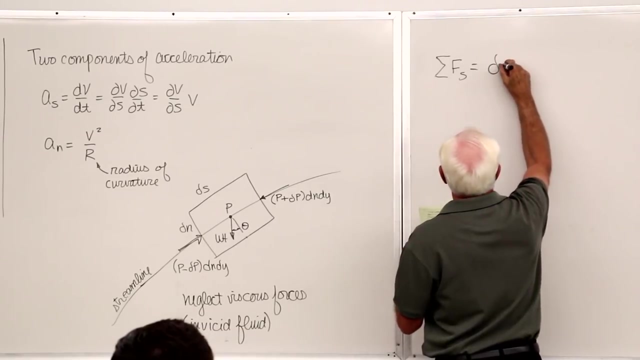 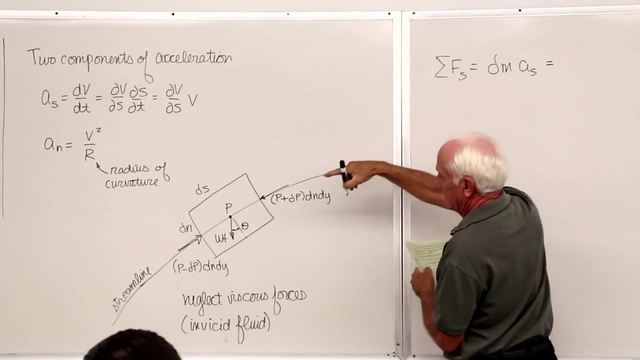 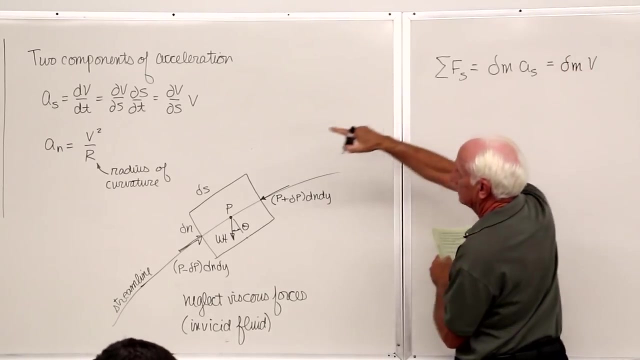 all right. so let's write the sum of the forces in the s direction and see we have obviously two pressure forces left and right. but we know when we do the summation of forces that it's going to be mass times acceleration. let's put that down first: mass times acceleration in the s direction is equal to acceleration in the s direction up there. so we have delta, m, v, dv, ds. 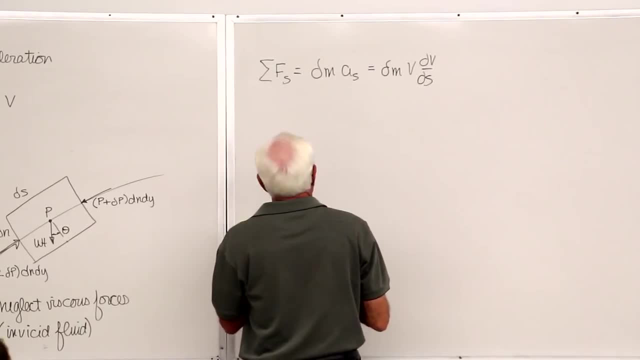 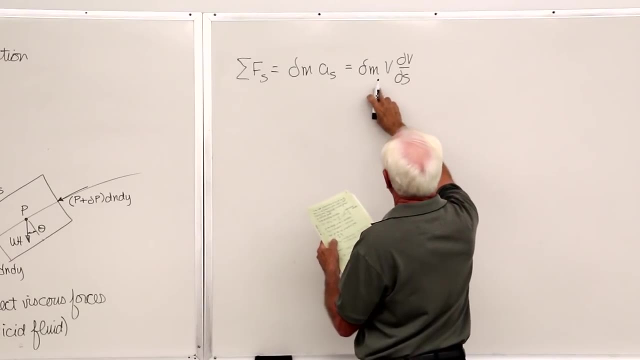 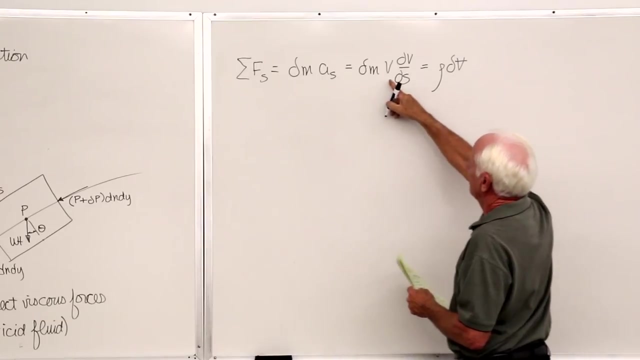 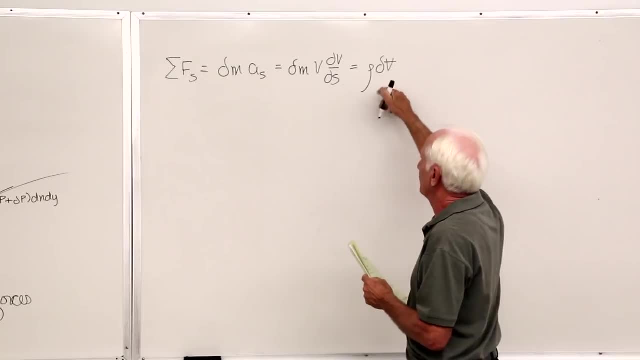 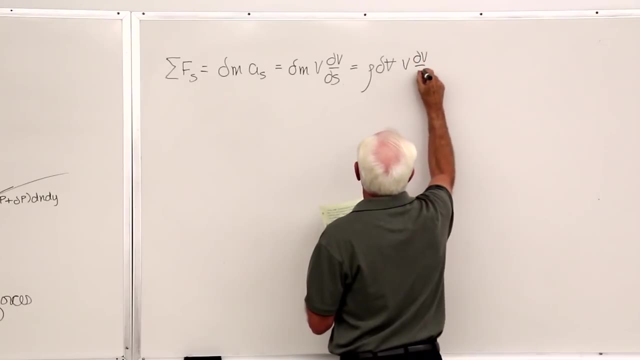 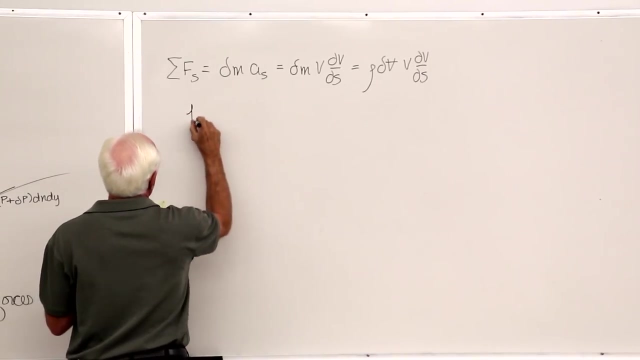 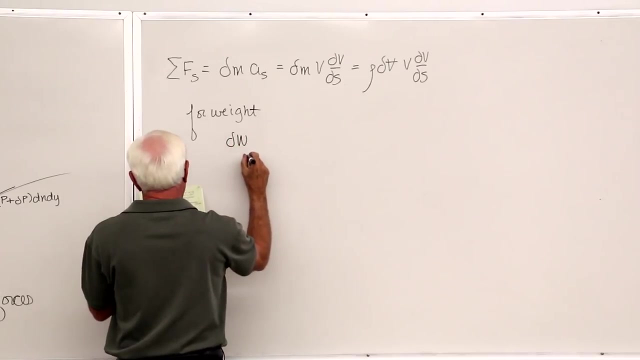 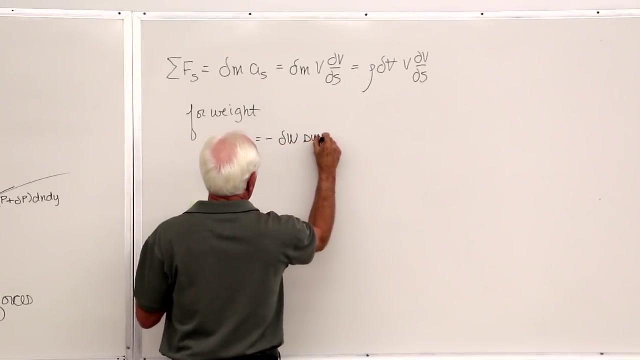 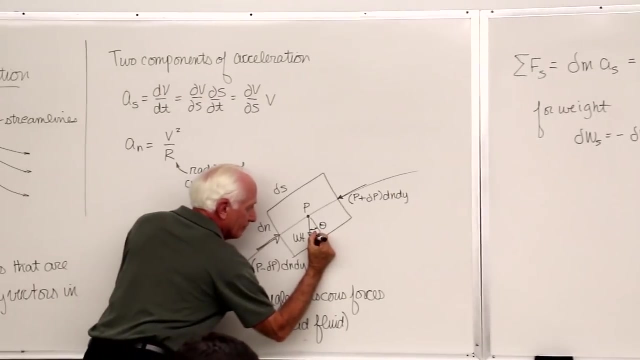 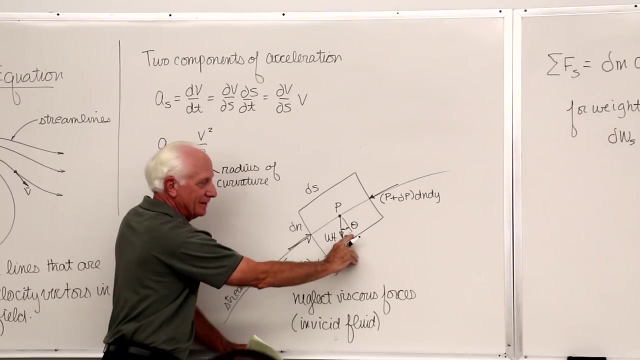 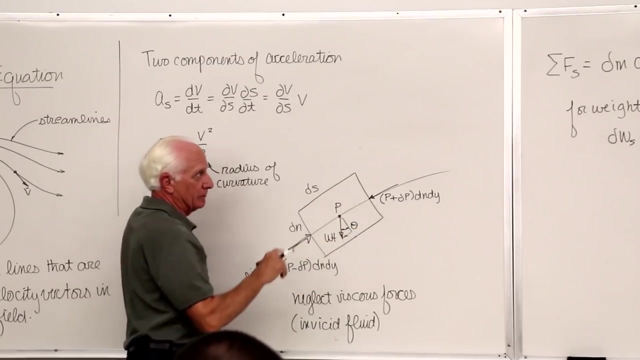 velocity. V slash means volume, differential volume multiplied by V, D, V, DS. okay, and for the weight, Delta W, the weight in the s direction, minus Delta W sine theta, that little guy right. there is the component of the weight in the s direction. notice which way it points, minus the sign. 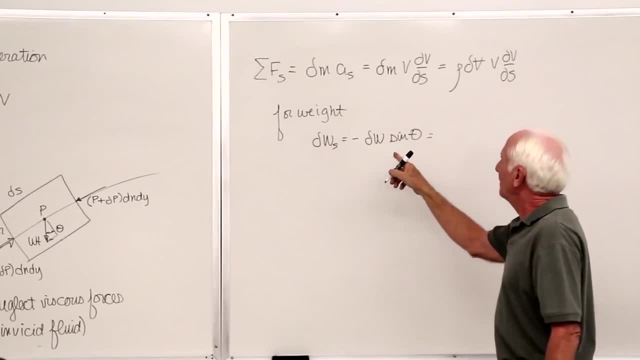 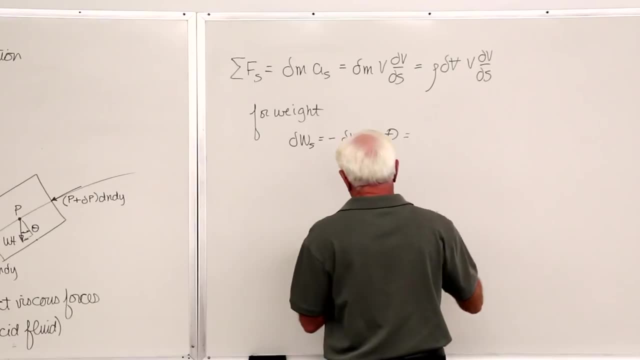 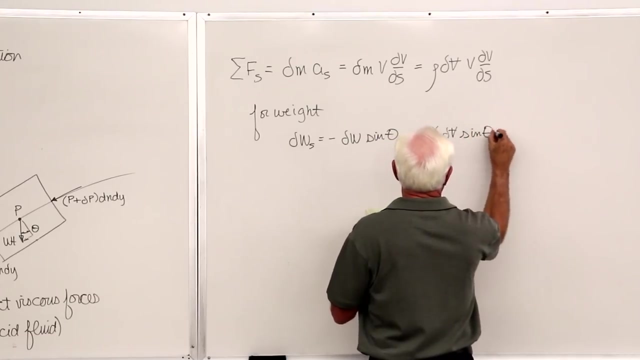 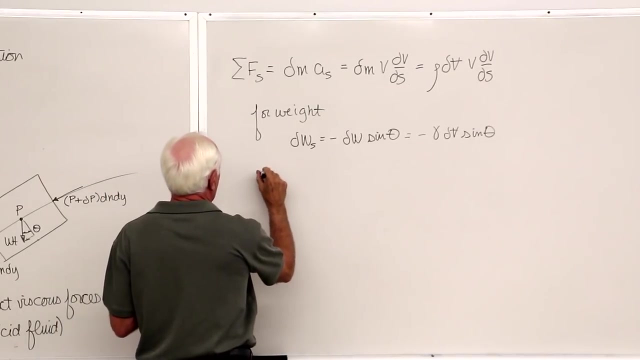 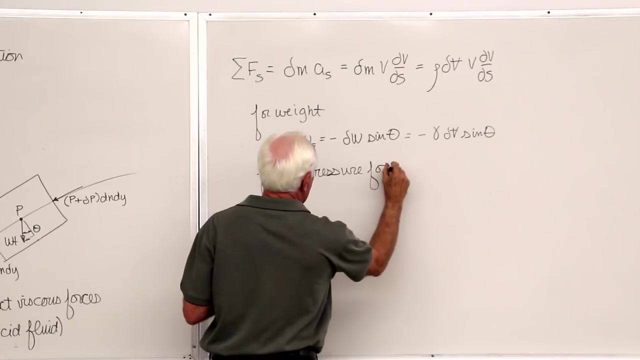 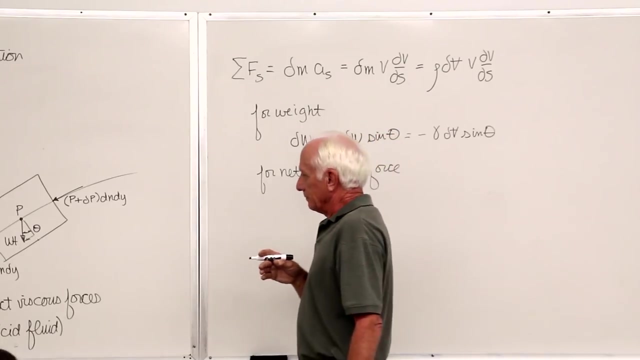 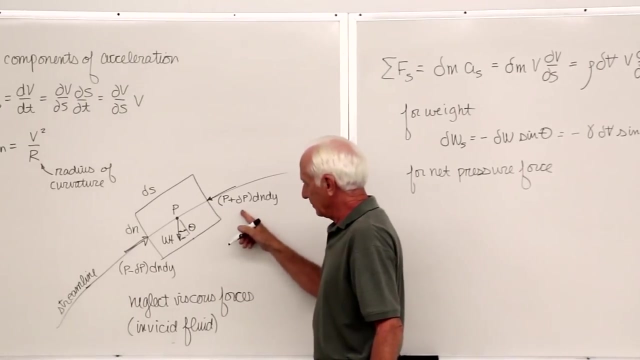 okay. what's the weight? gamma times the volume. so, minus gamma delta volume, sine Data component weight in the s direction: the net pressure force. the net means subtraction something, Net always means subtract something. So if we subtract this guy and this guy, the two pressure forces, the two pressure forces subtract them and we end. 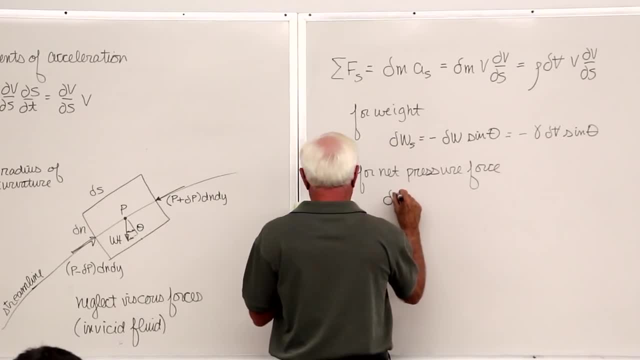 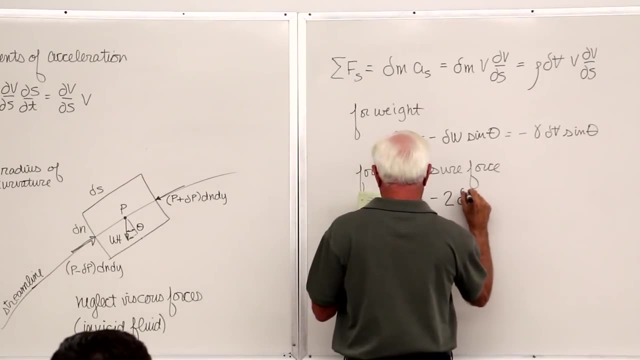 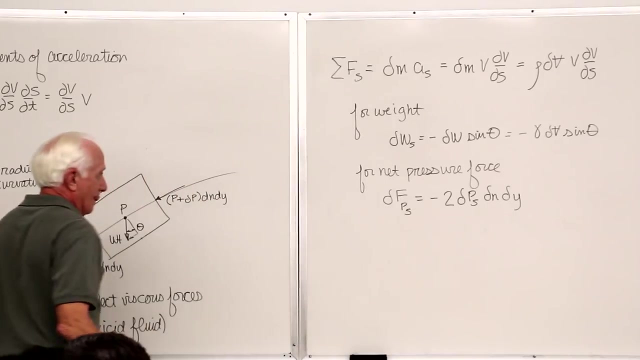 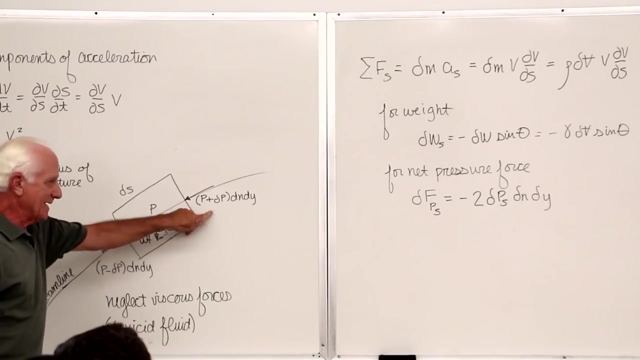 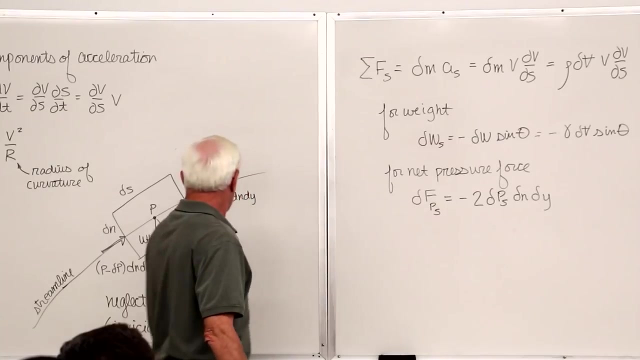 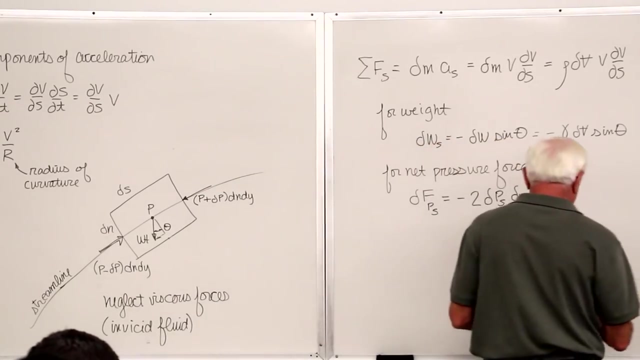 up with delta F pressure force in the S direction. Okay, this guy minus that guy, the P's, cancel out. plus P minus P. minus Delta P. minus minus Delta P minus 2 Delta P. yes, that Delta PS again just means in the s-direction. don't need to keep that such on there. so this then: 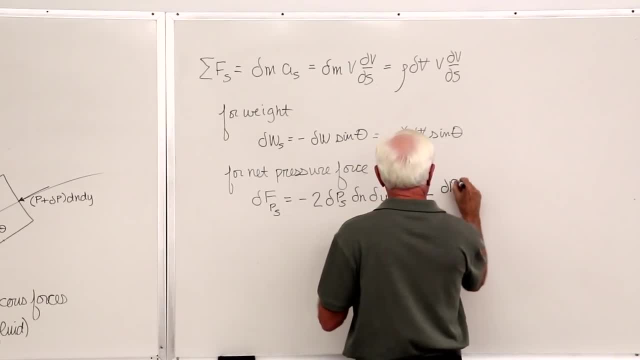 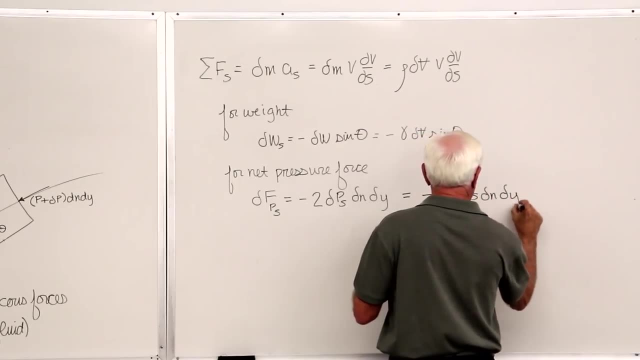 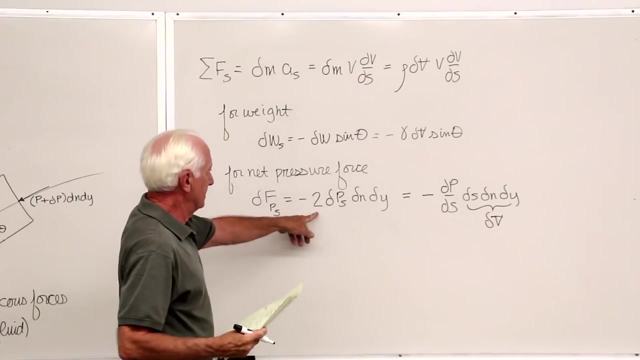 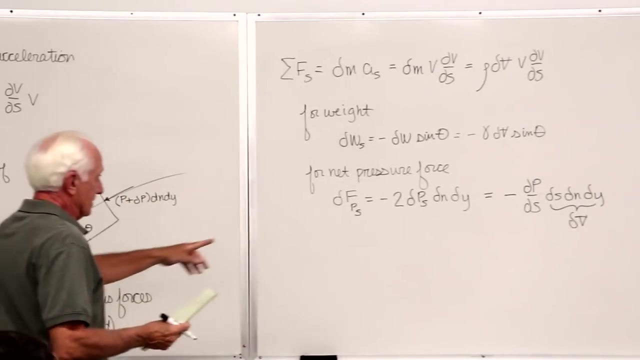 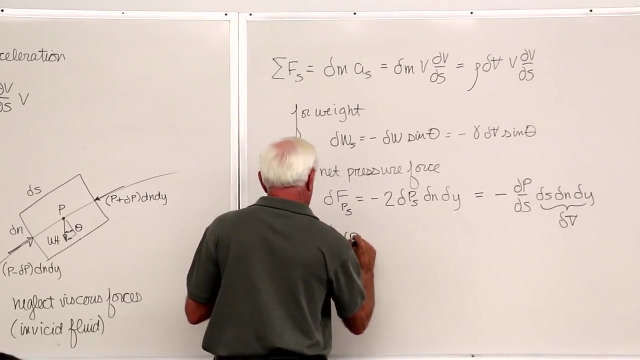 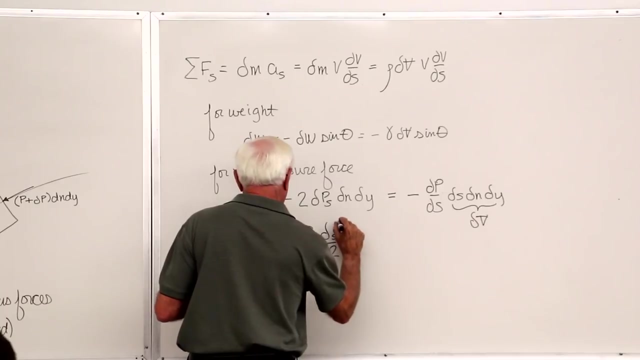 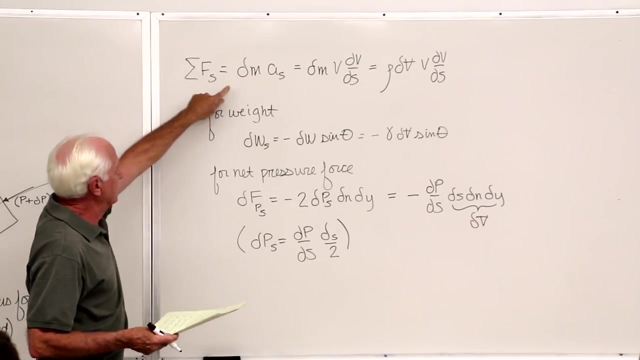 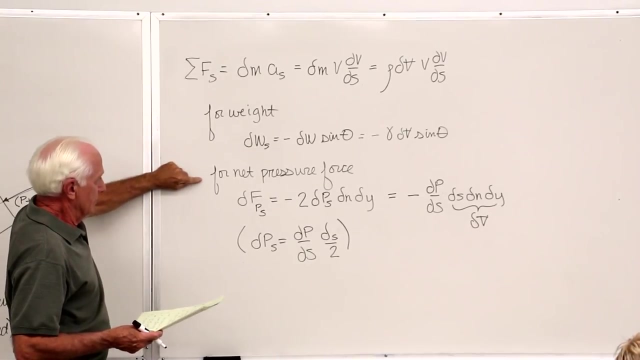 becomes replacing the Delta PS to this guy right here. okay, that gives us that, using this all right summation of forces, equal mass and acceleration. what are the forces? the weight of force to the weight in the s-direction. the force to the pressure depression in the s-direction. so here's our components. okay, so next step put. 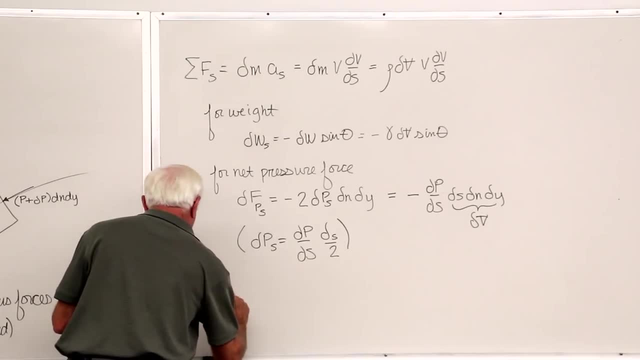 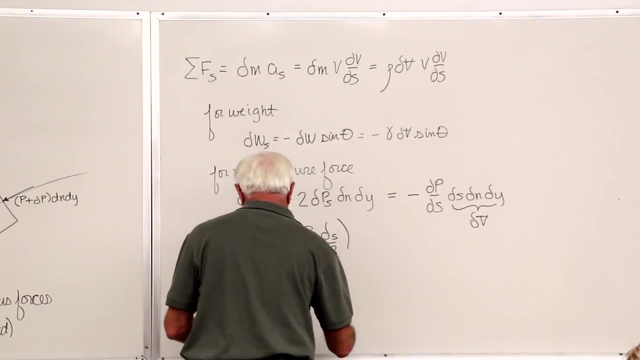 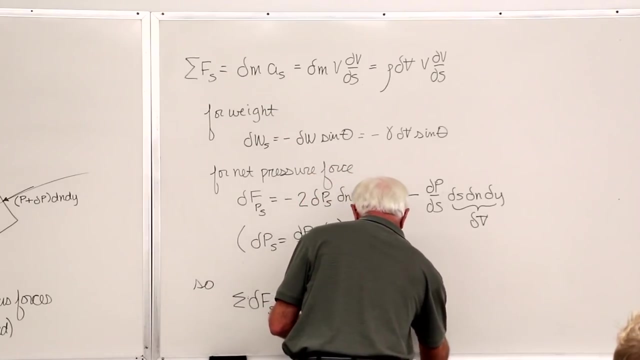 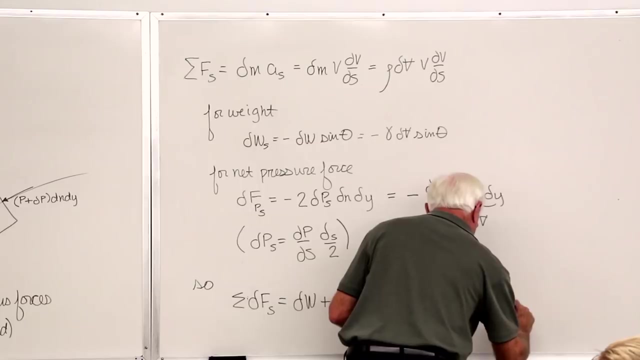 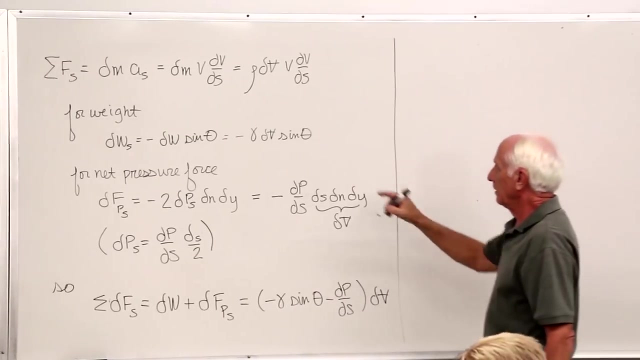 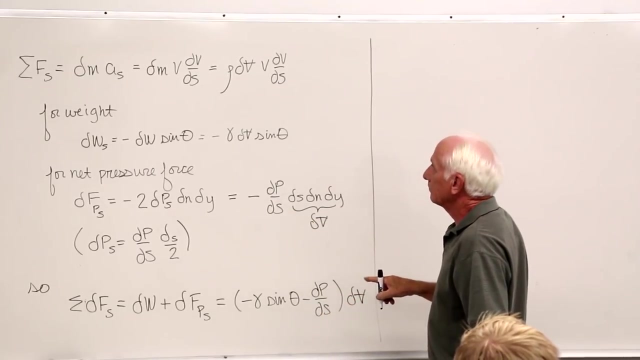 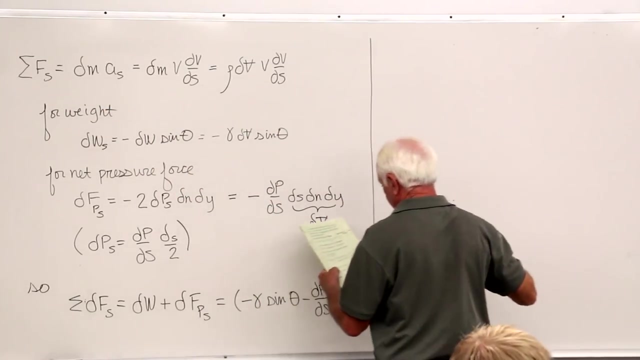 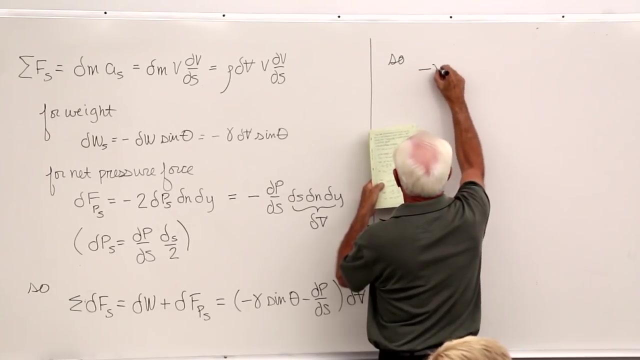 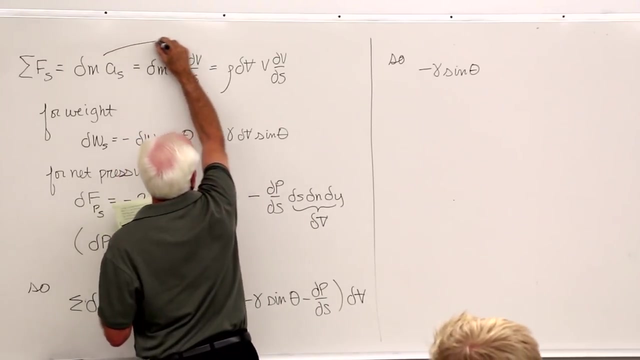 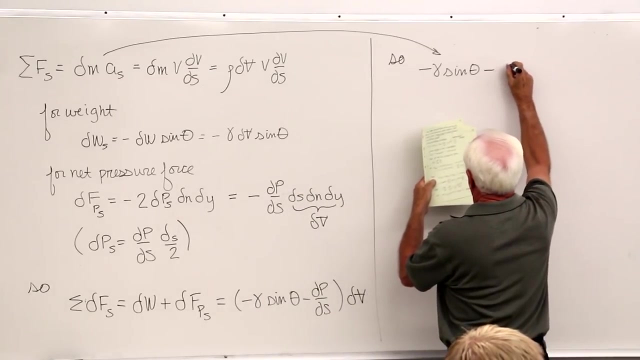 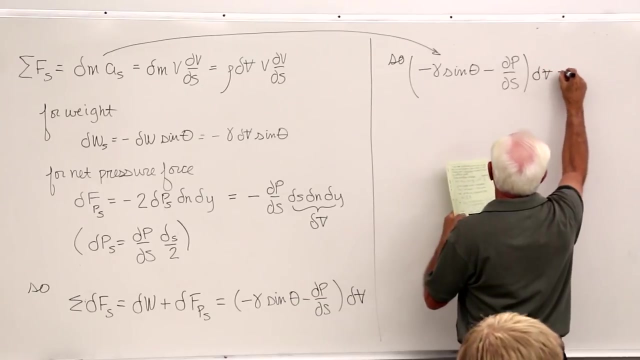 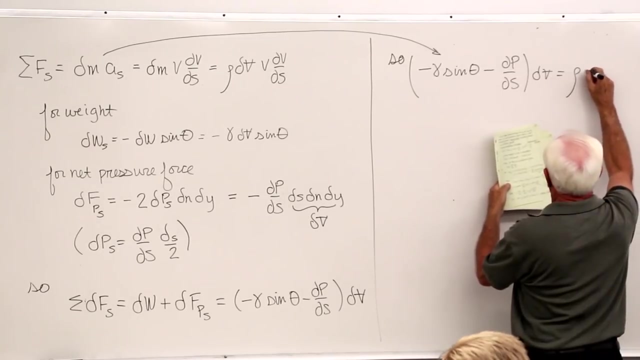 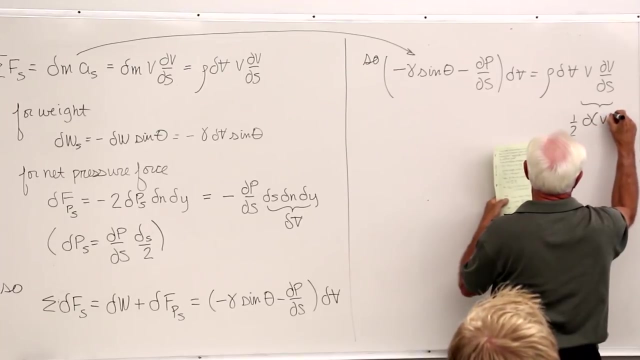 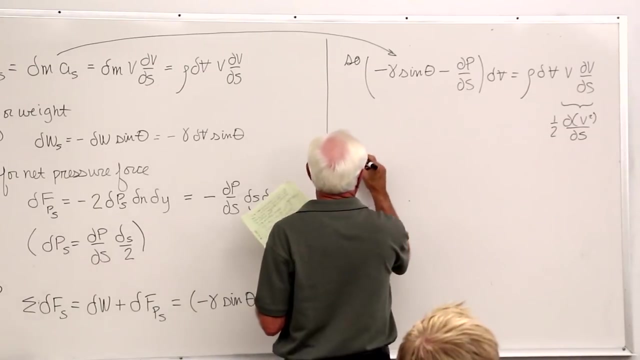 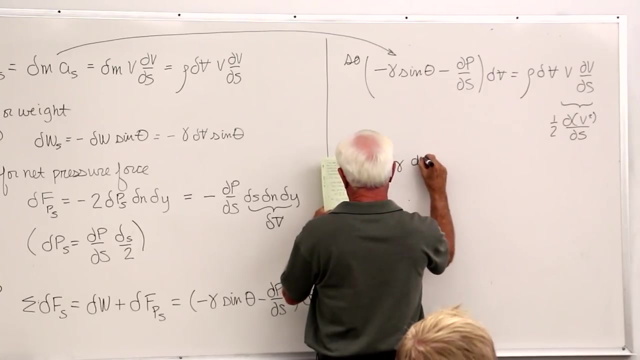 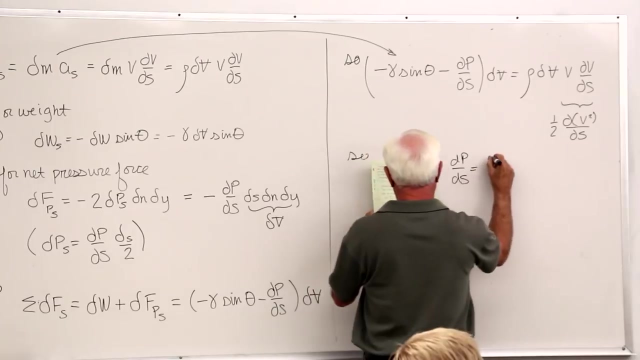 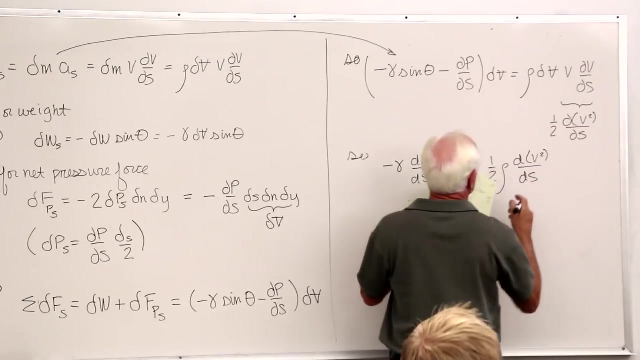 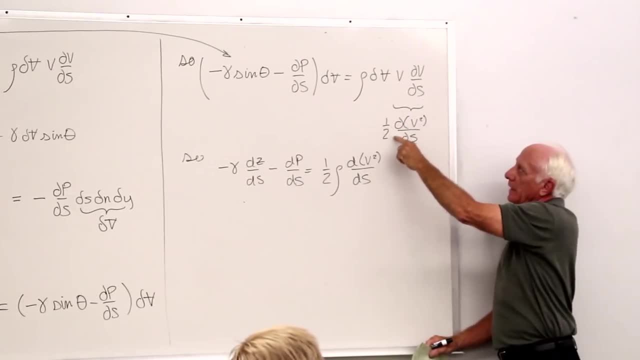 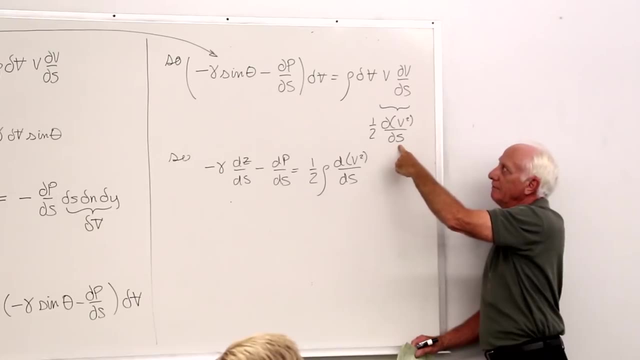 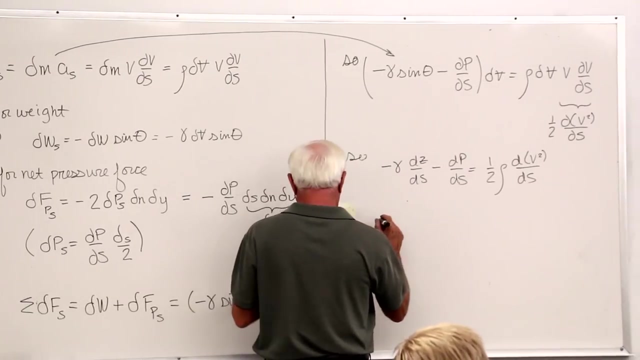 There it is The differential: one-half dv squared ds. dv squared ds is 2v dv ds. 2v dv ds times a half is v dv ds, so they're the same thing. Finally, we get expression vp. 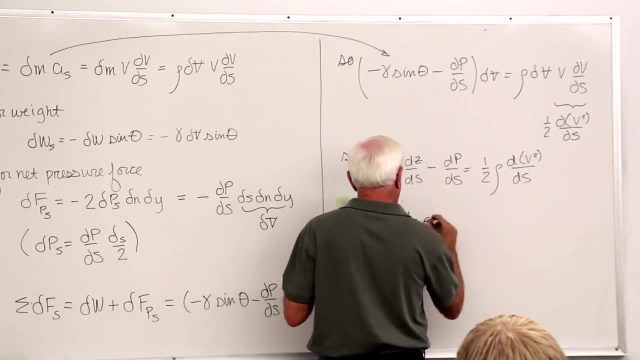 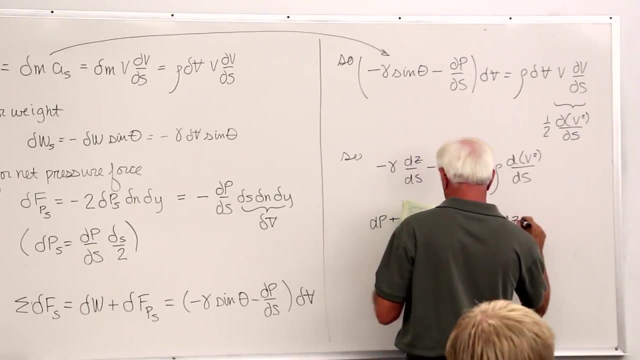 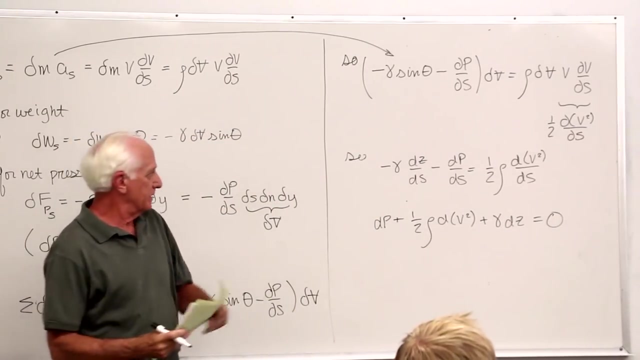 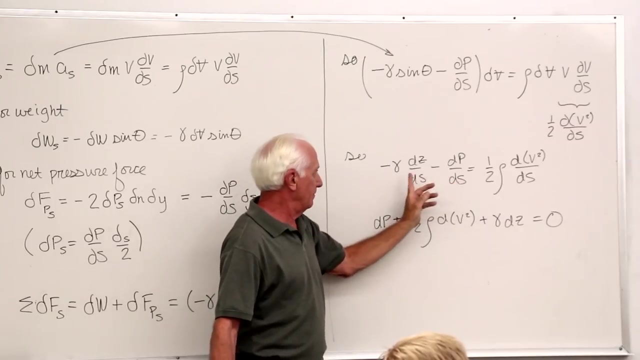 Let's de-peak them out of there. Remember: multiply through by ds. multiply through by ds, cancels out, cancels out, cancels out. You're left with dp. change. move these two guys, right-hand side plus dp. 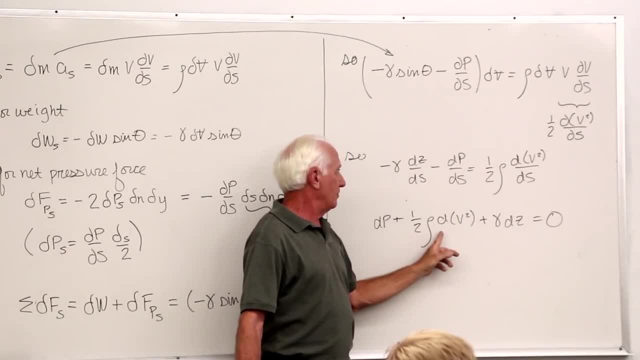 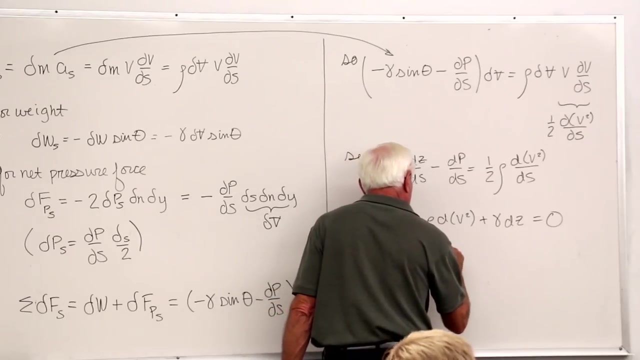 He's over there. one-half rule dv squared. Put them over to the right-hand side. change the sign gamma dc. there it is. So this is only valid, though, along the stream line. Okay, Okay, Okay. 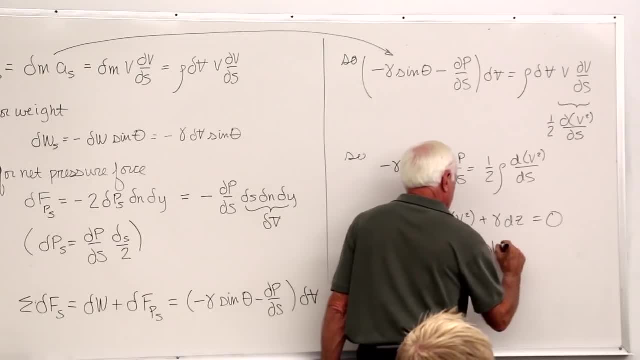 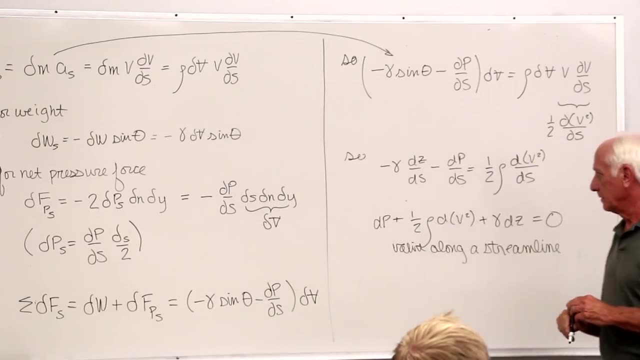 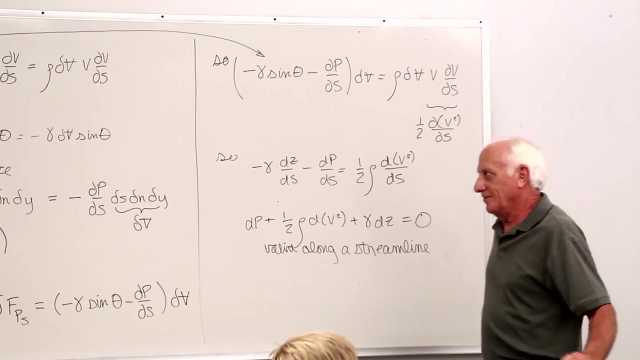 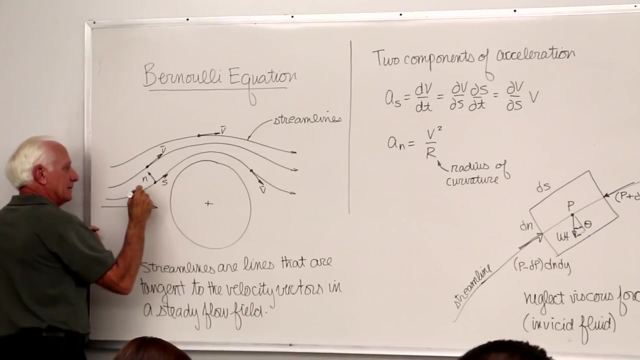 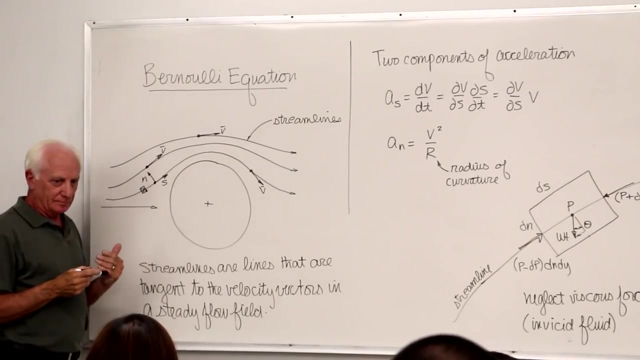 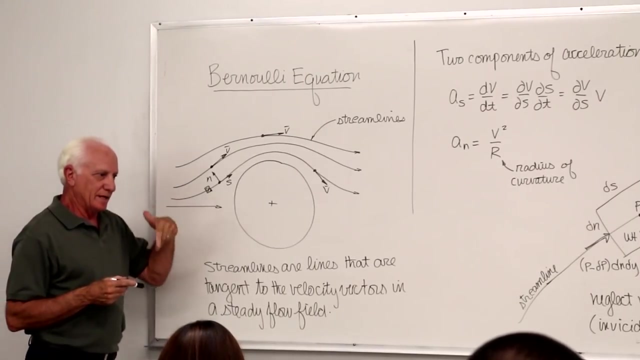 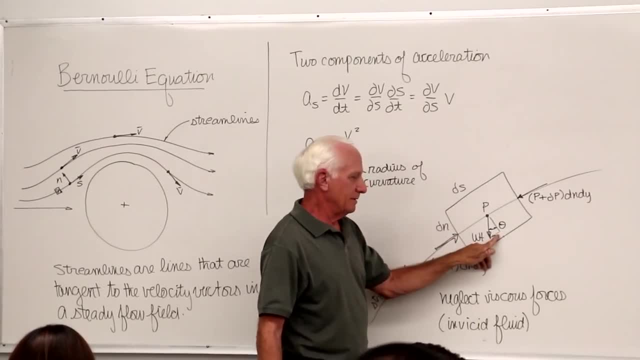 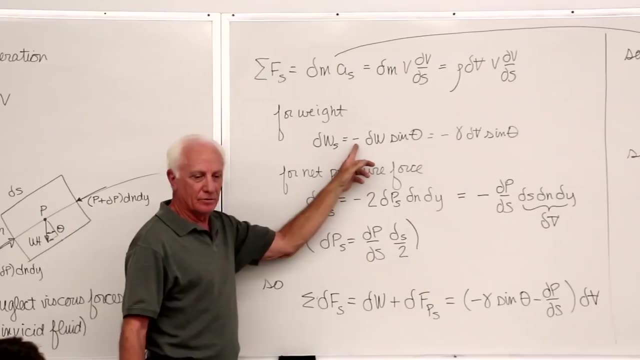 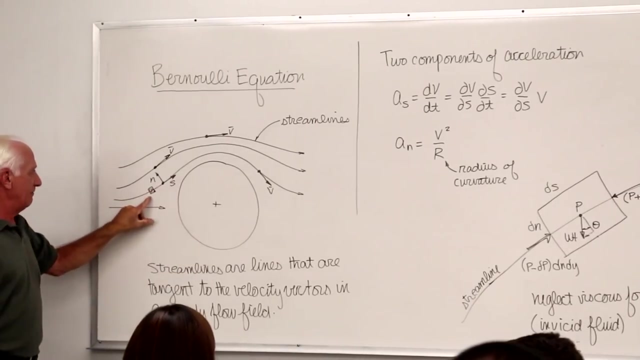 So the weight, The component in s direction, sine of theta, okay, that's the weight Acts down minus sine, of course, The pressure acting on the left and right-hand faces of the element number one, call the pressure in the middle p. 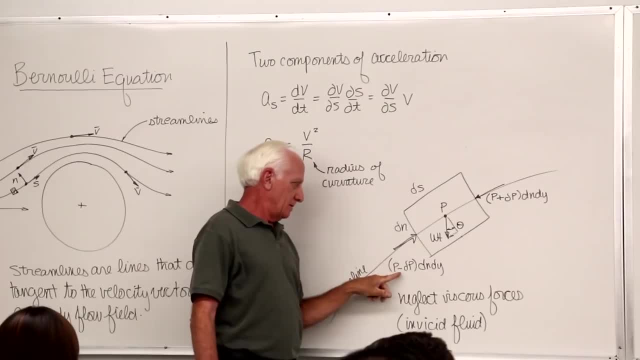 If you go in the negative s direction, that's towards me, of course, the pressure is p minus dp. If you go in the positive direction, that's minus dp. If you go in the negative s direction, that's minus dp. 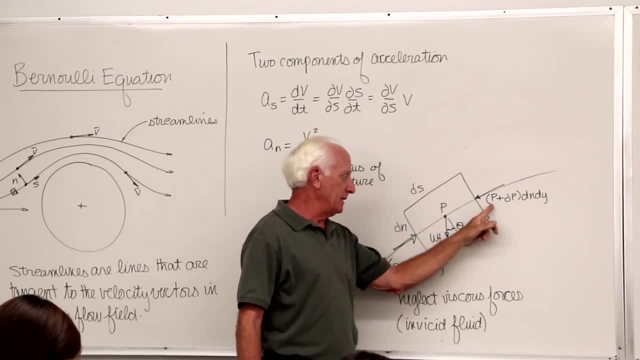 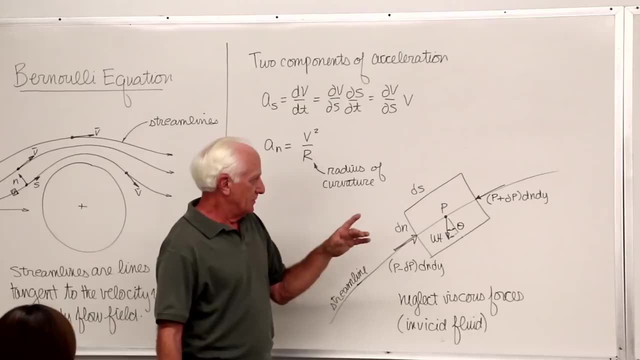 If you go in the positive s direction that way to my right, then it's p plus dp. Multiply a pressure by an area that gives you a force. If you take the difference in these two pressure forces, left and right-hand sides, 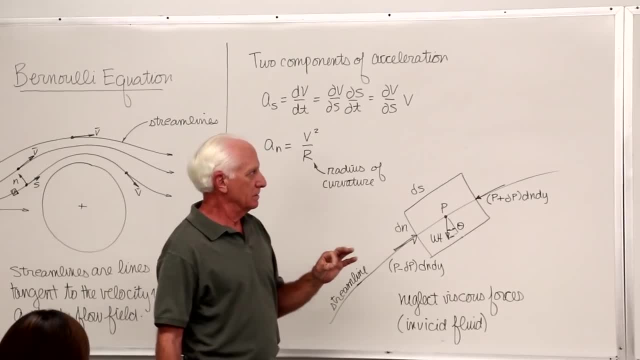 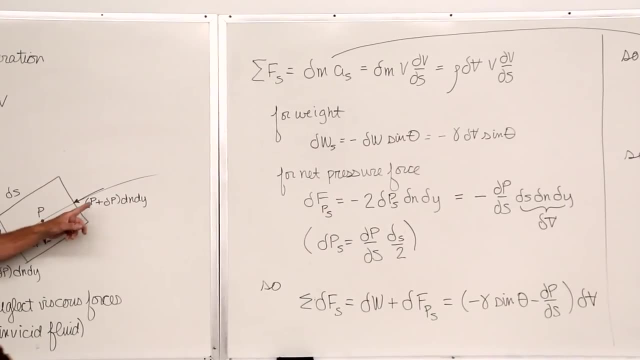 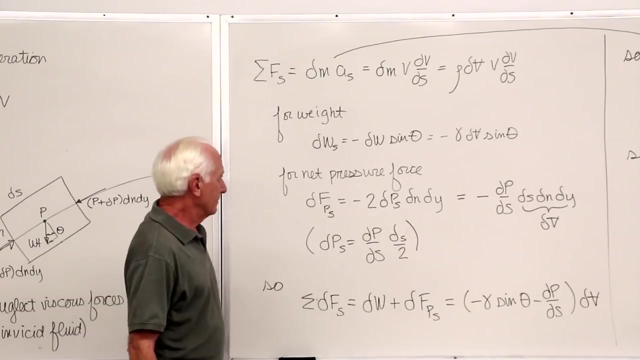 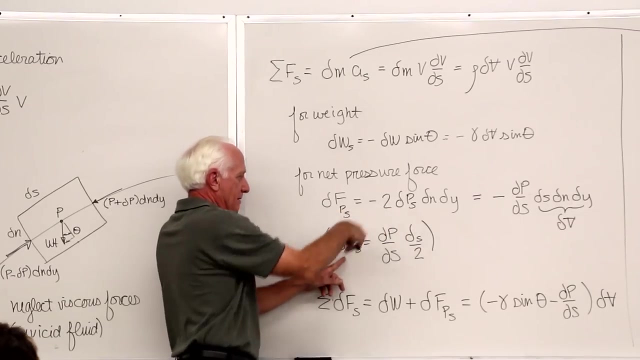 it's going to give you a net pressure force, Net pressure force. So take this guy minus that guy and you end up with this one. Use this guy in here. Okay, Delta p s right here, Put that in here. 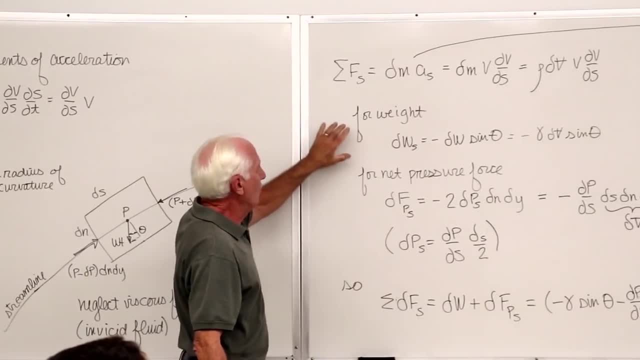 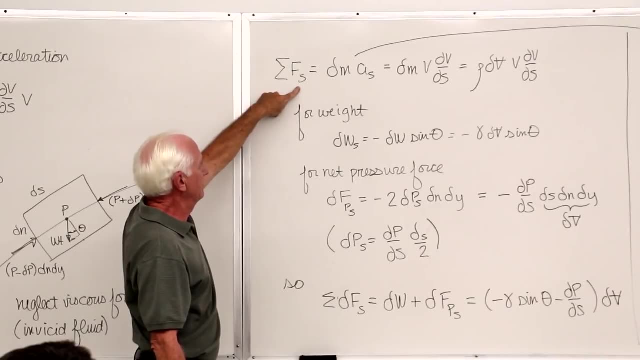 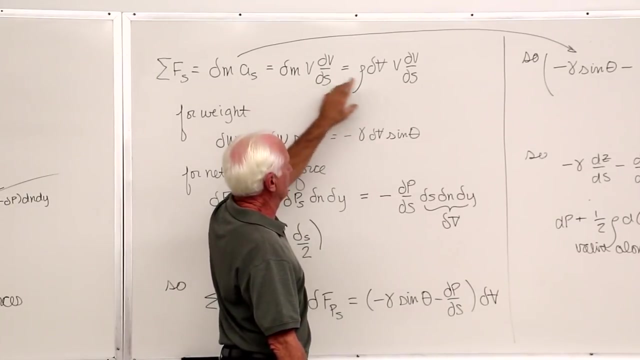 Okay. so net pressure, force in the s direction, Weight in the s direction. Put the equation: summation of forces in the s direction: Equal weight plus pressure, Equal mass. something Equal mass, something. Acceleration: this term is mass times. acceleration redone in a little better format. 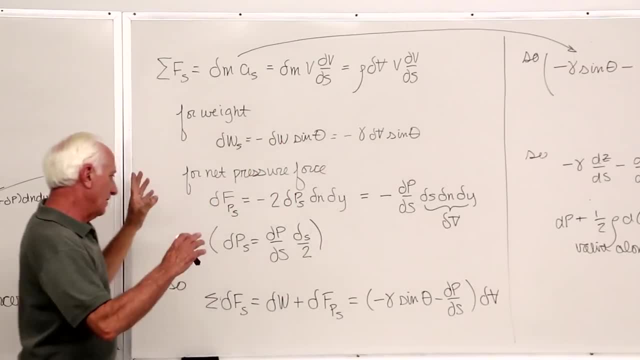 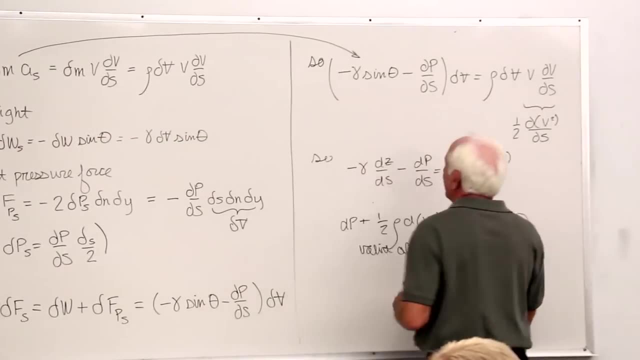 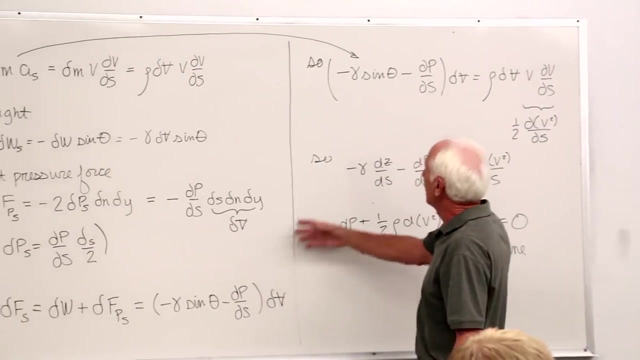 Rho, dv times, velocity, dv, ds. Put all that stuff in the equation Here. it is down here. Play with it some more. Get it in a form that's useful. Get it in a useful form. That's our object. It's not a useful form yet. 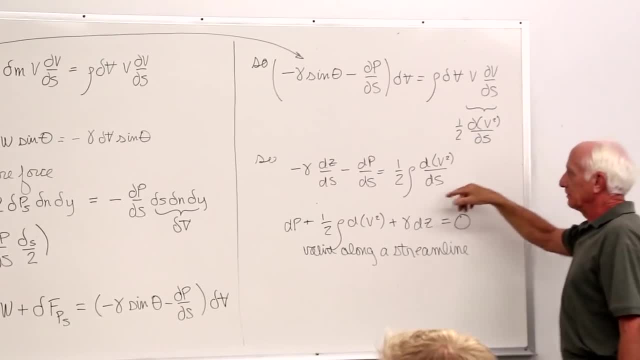 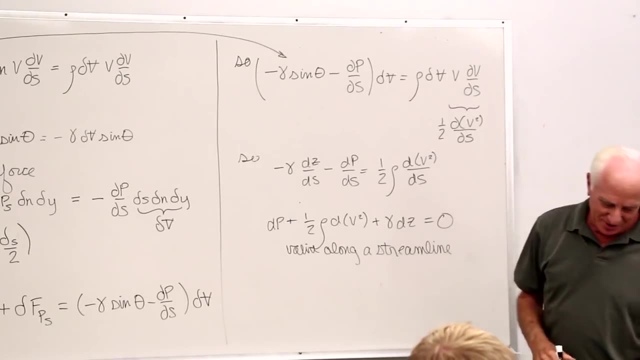 We're getting there. Make some changes here. This guy right here, Multiply through by ds. Put all this stuff on one side of the equation. There it is Okay. We're almost almost there with the for the least, Okay, yeah. 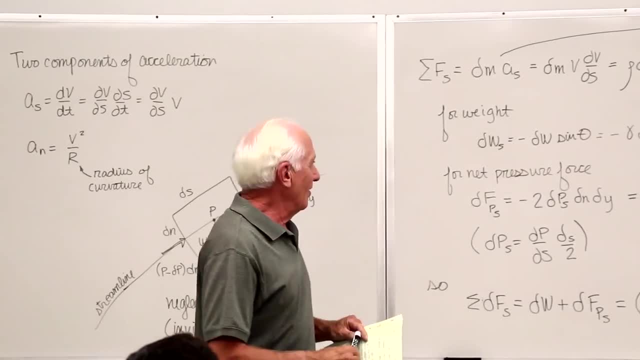 What happened to the sine theta? Oh, let's see Where did the sine theta go? Oh, He's in the. yeah, he's, yeah, he's up here. Gamma, what did we do? Should I get that one right? 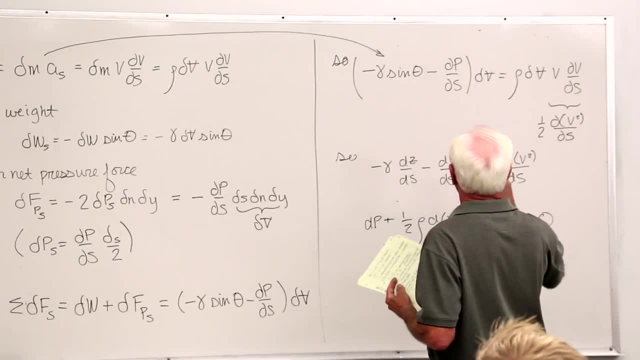 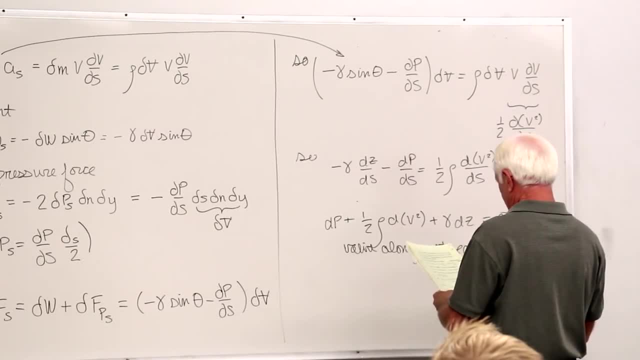 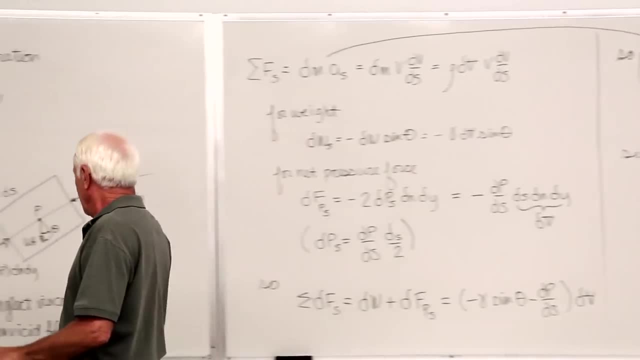 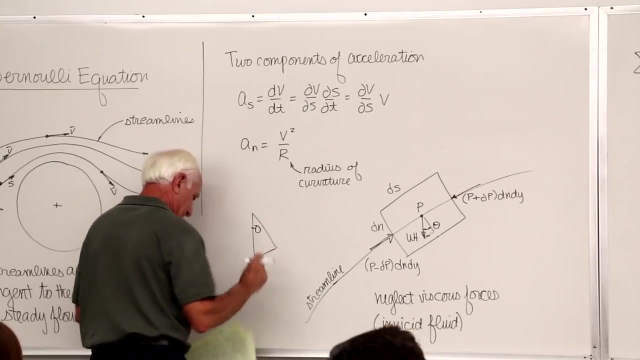 Sine theta dp. Over there we've got sine theta and PdS gamma the PdS, Oh Yeah, Um, This is Let, let me put down. I didn't put this. it's in your textbook, but I'll put it on here. 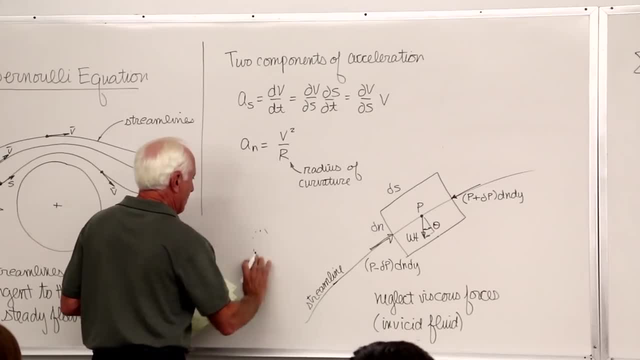 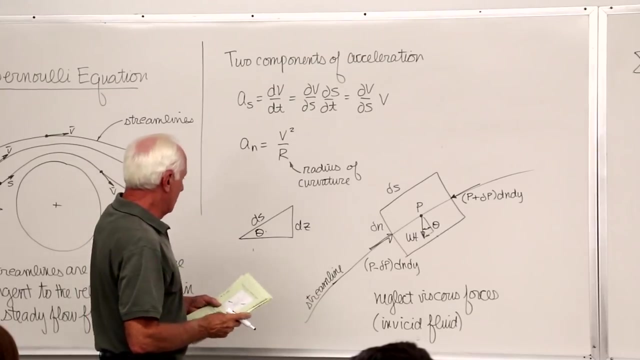 This is theta. Oh, that's the wrong way to talk. Like this, Like this. So again, comme ci, comme ça, comme ça. Right, Right, this is DS. this is easy. this is theta. okay, so sine of theta is what, easy over. 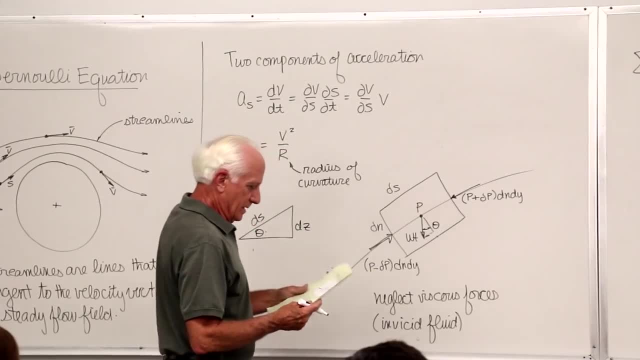 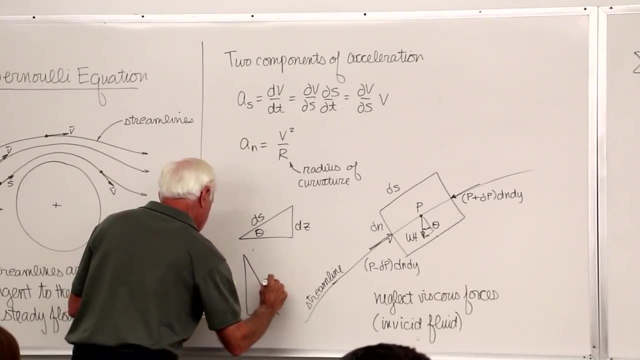 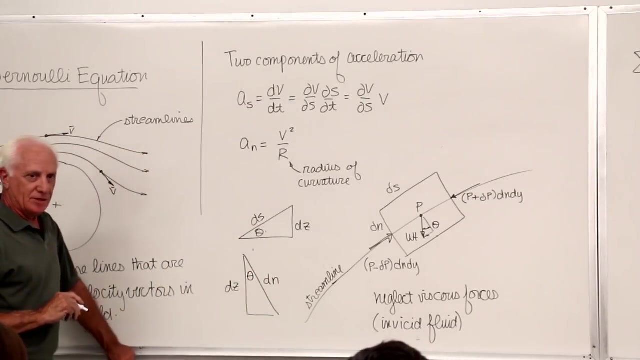 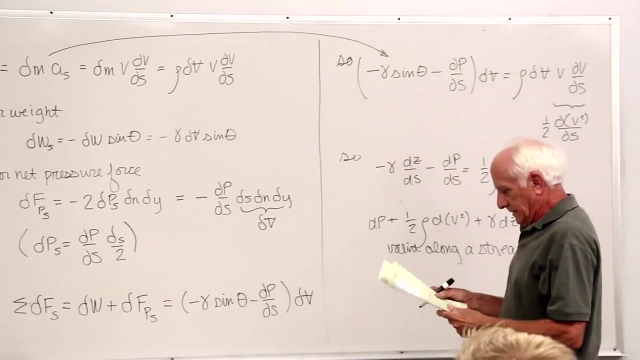 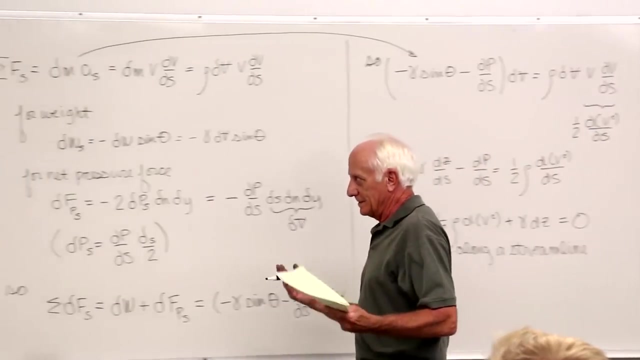 DS, one, draw one more. okay, here, here, here, DN DC, theta, cosine theta, DC over DN. you can play those games. you get rid of the sine theta. okay, just go back into the geometry again. thanks, you mentioned it disappeared, did disappear. I replace it with a differential. okay, now, obviously we don't want EP DB squirting DC. next up obviously is to 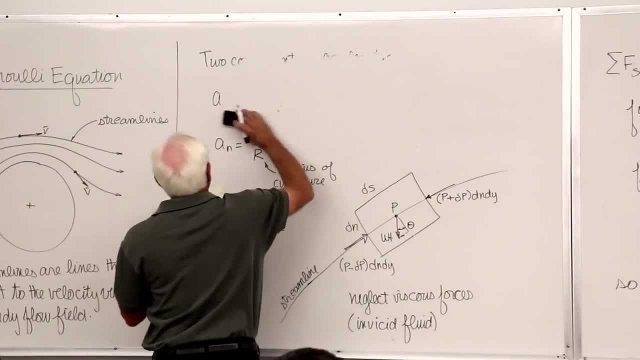 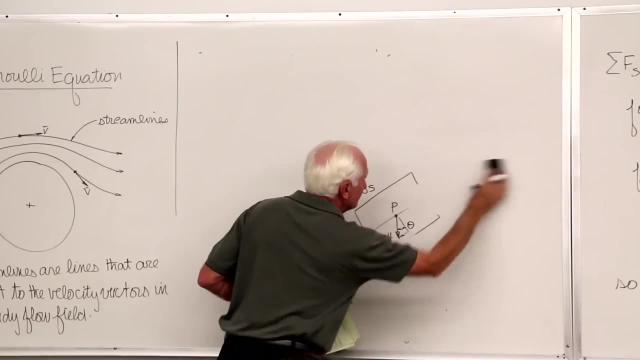 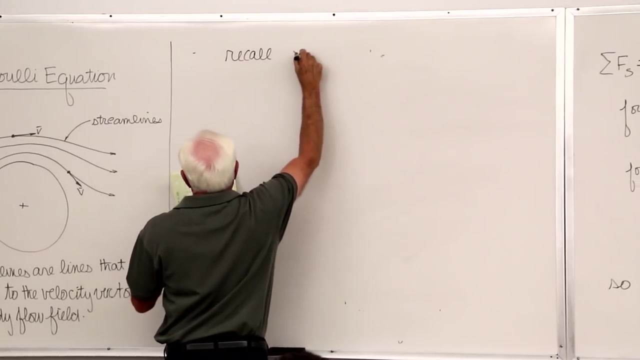 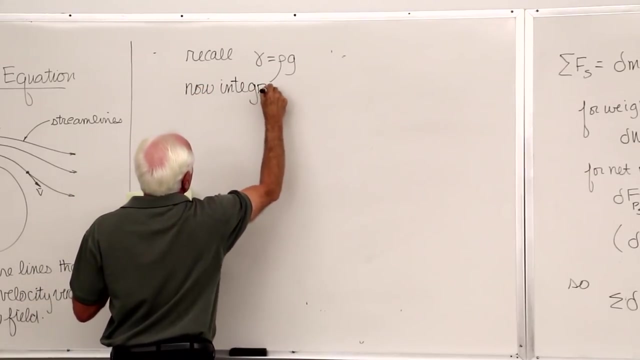 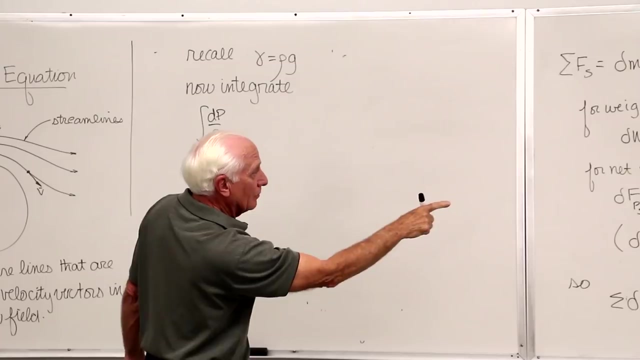 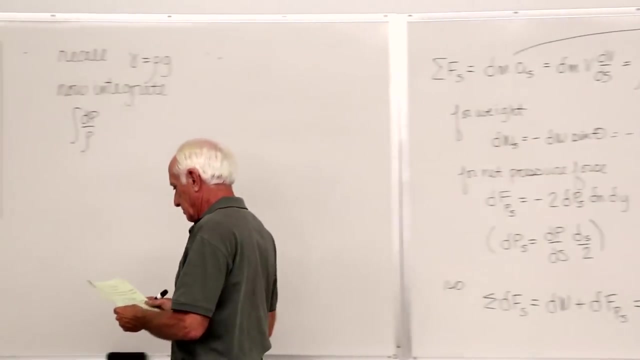 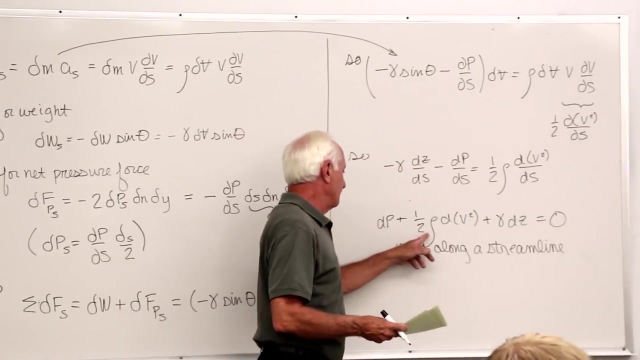 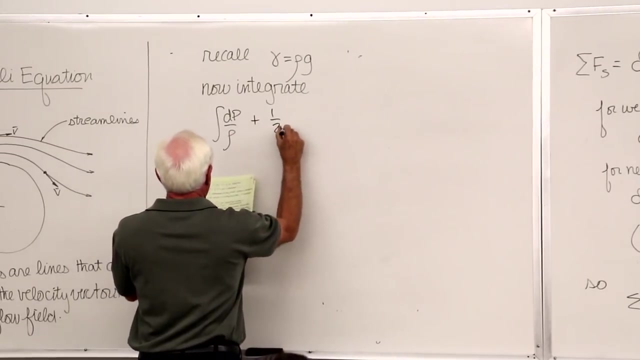 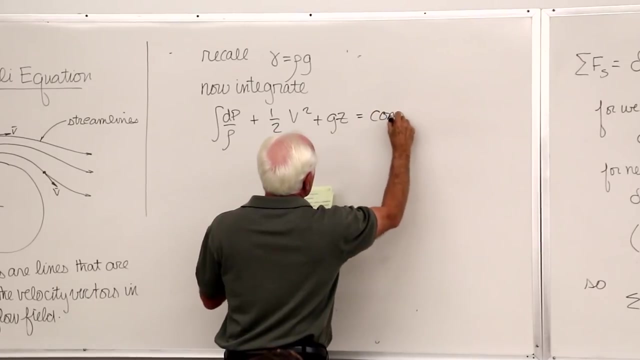 integrate. okay, so we're going to integrate. woah, yeah, all right. here's the terms. we divide through by Rho. divided through that row DP of a row 1, sı 2, they, you gz. g is a constant. pull it outside. Call the constant c When you get a grade, we end. 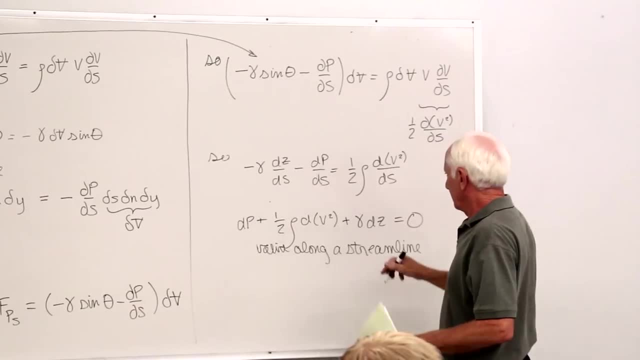 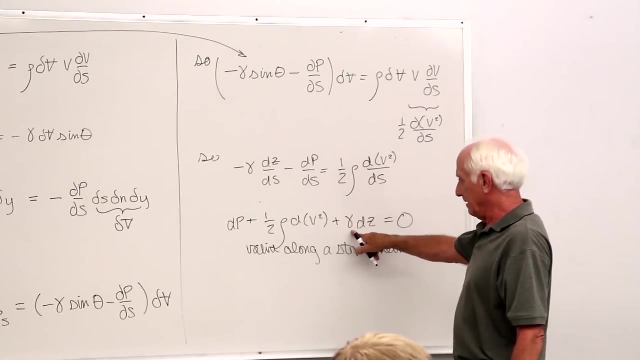 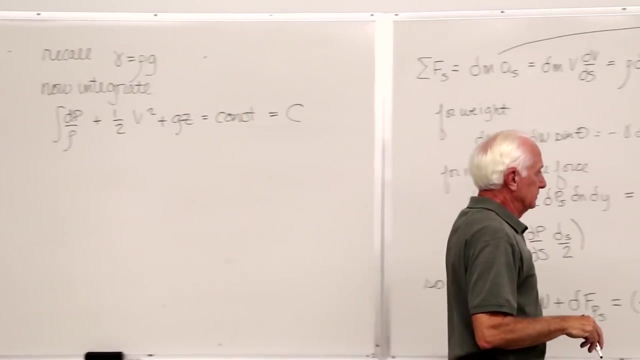 up with a constant c. What's gamma Rho times g? What do we divide by Rho, Rho g divided by rho is what g times z, Yeah, g times z. Integrate him, pull the half outside, pull. 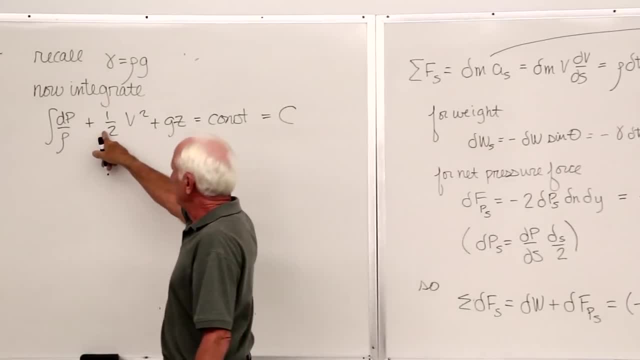 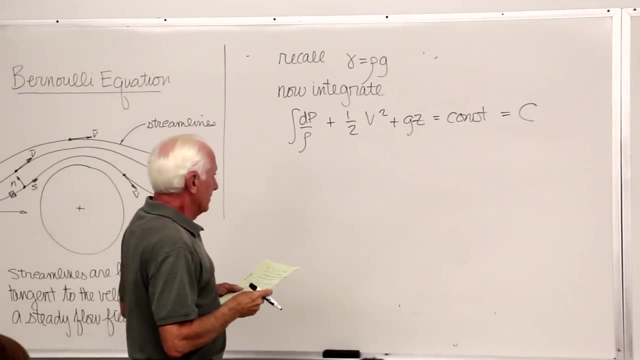 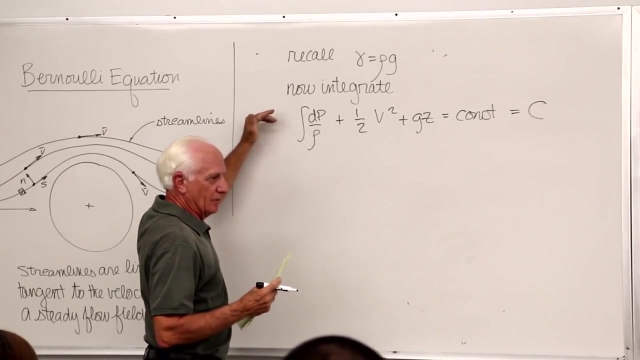 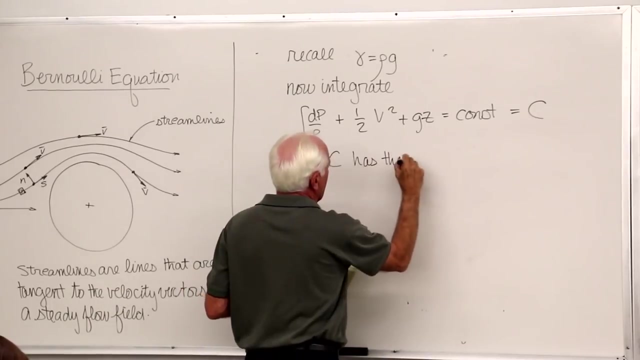 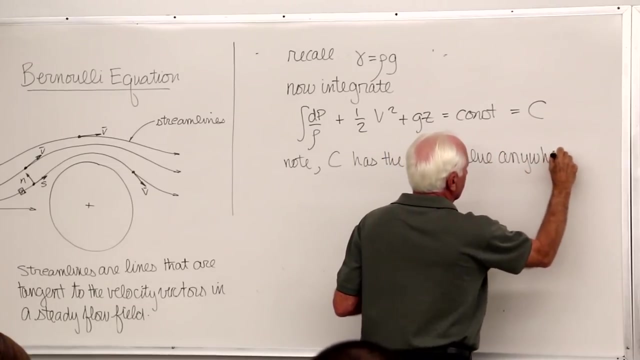 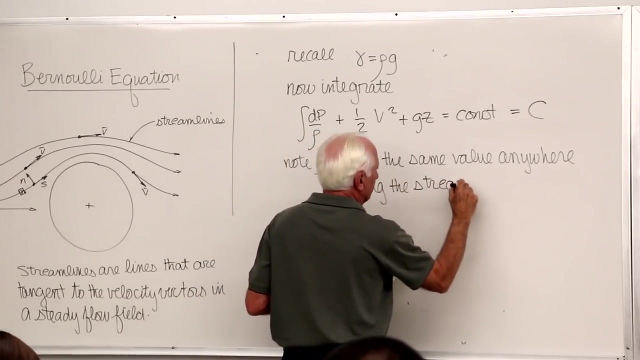 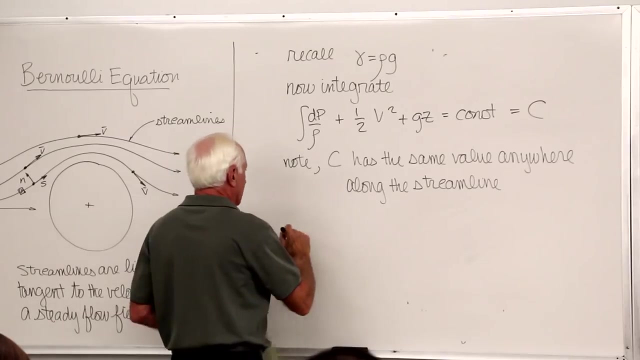 the rho outside divide by rho and that's gone B squared. that's where it came from, So c is a constant Notice that this is written for our streamline. c has the same value- any work along a streamline- Okay. 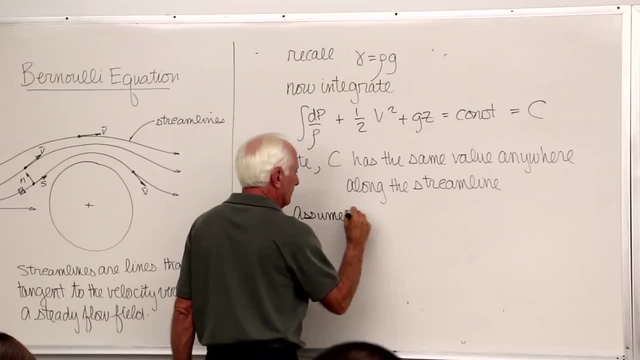 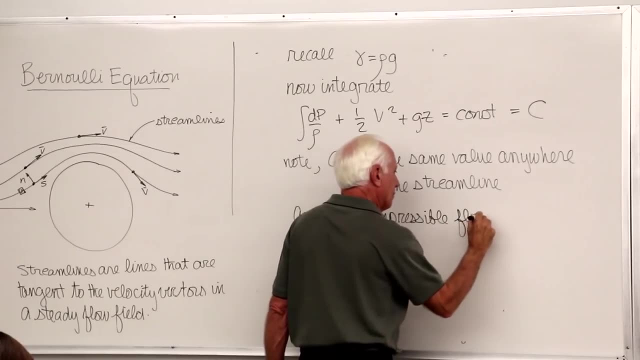 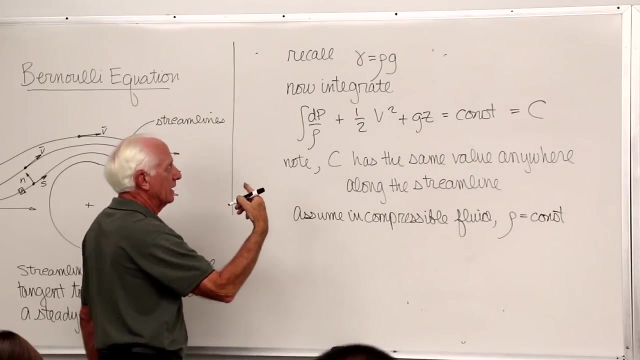 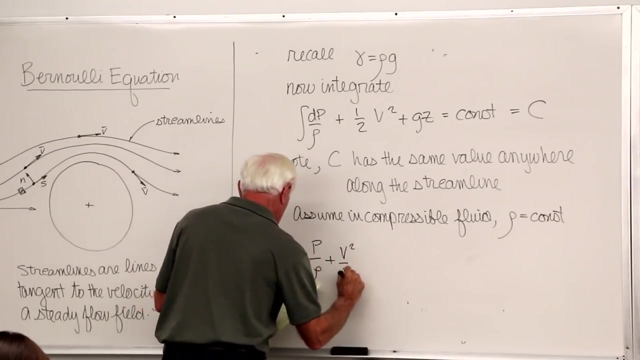 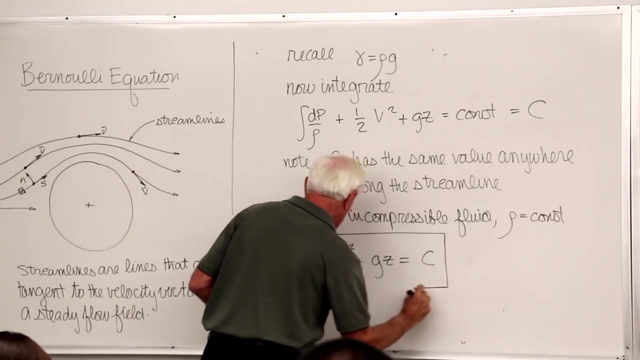 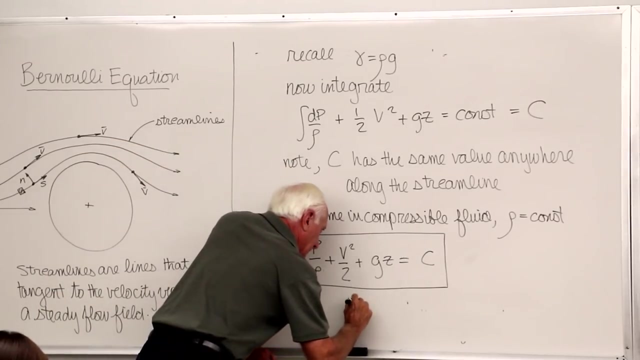 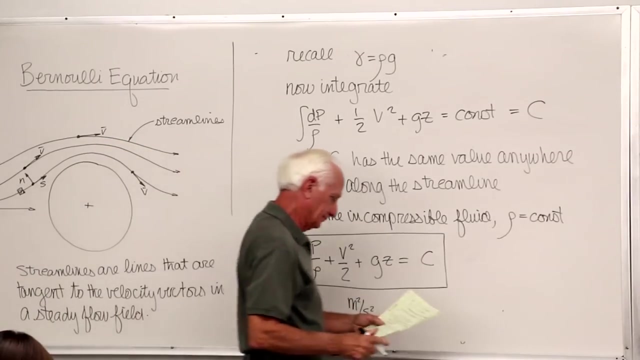 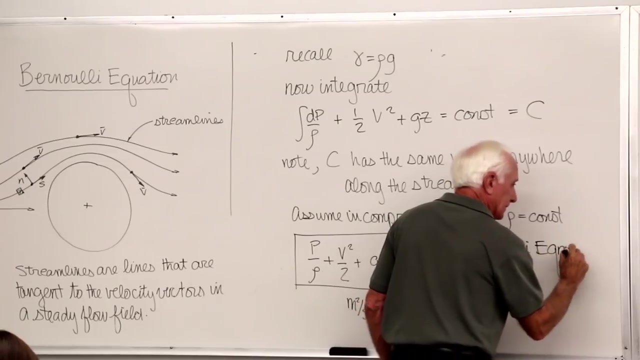 So now we assume incompressible fluid row equal constant pole row outside there, no sign. okay, end up with P over Rho, V square over 2 G, Z equal to constant C. every term has units meters squared per second square, the famous Bernoulli equation. 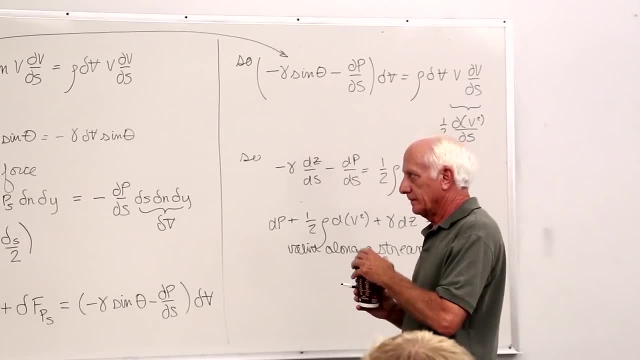 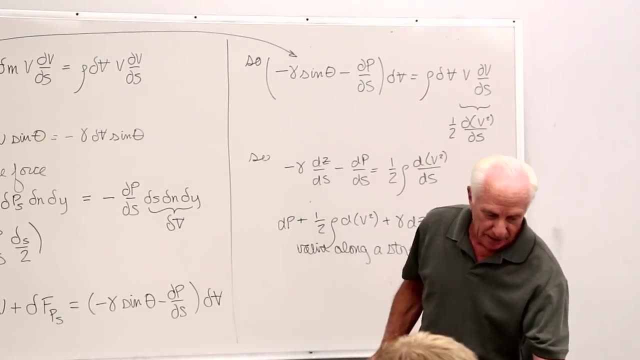 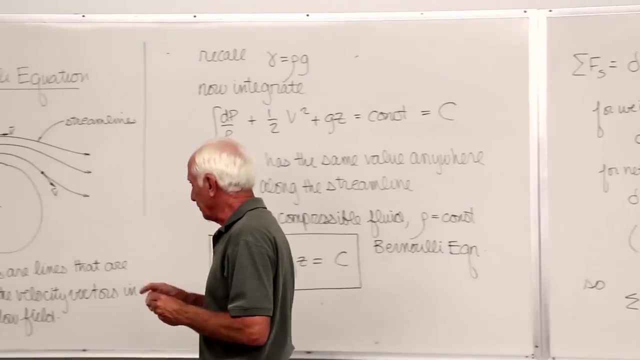 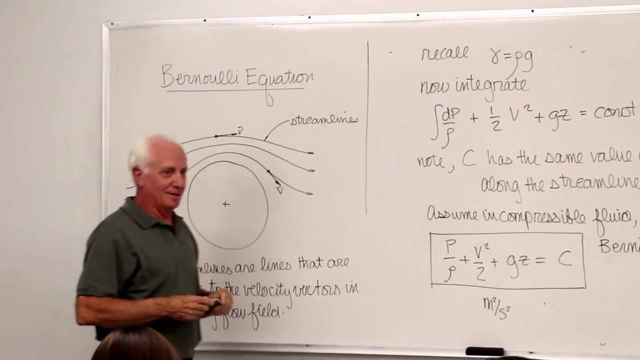 it's a pretty straightforward derivation because it's inviscid. later on we're going to repeat this, but we're going to allow for viscous stress terms where, on the two top and bottom sides of this, that's going to be a lot rougher derivation, but this one is. it is. 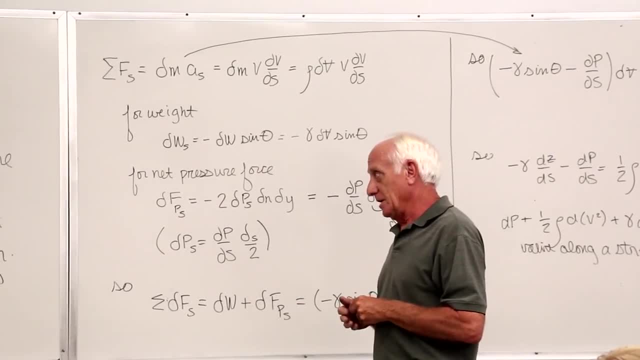 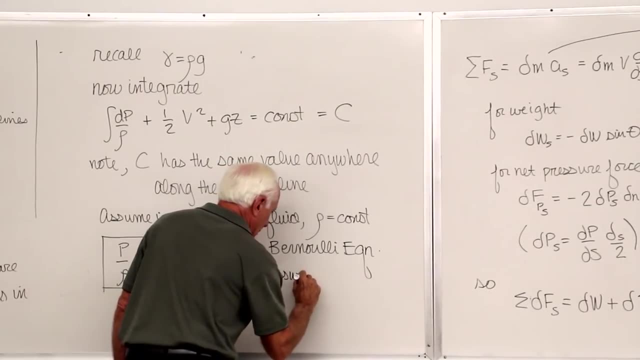 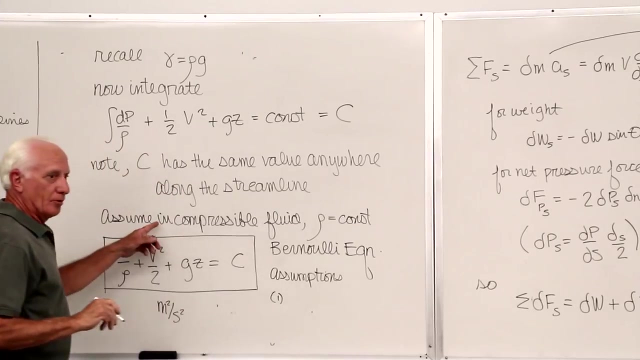 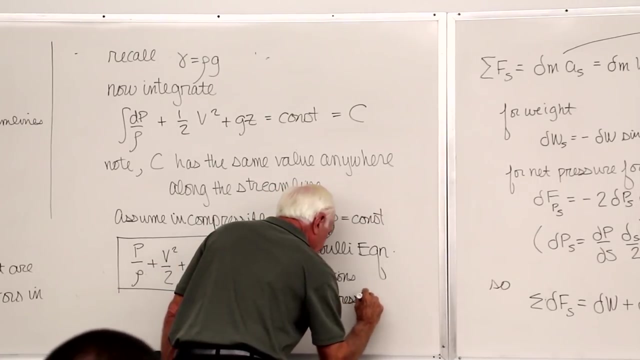 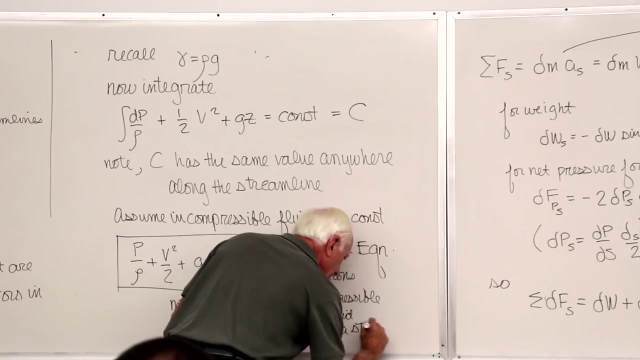 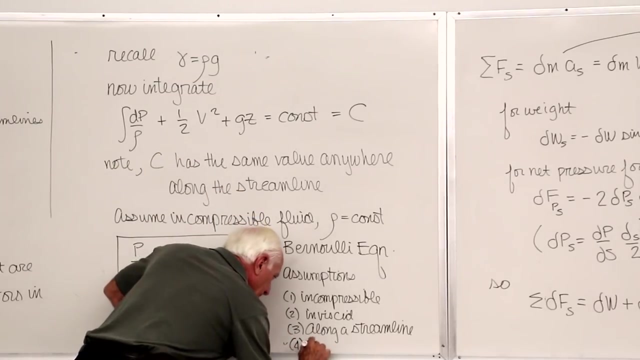 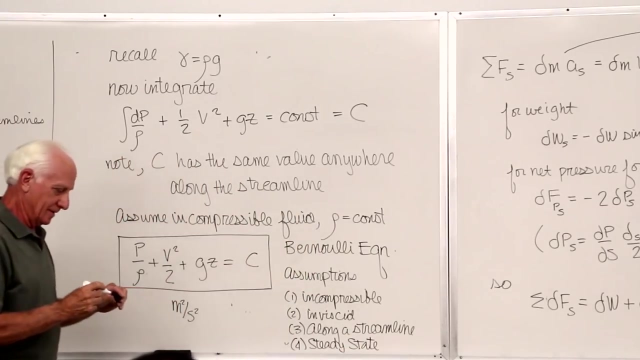 good a lot of times you have to remember though. remember it's assumptions. we pulled row outside and compressible. we said early on in business along a streamline. we didn't emphasize it, but of course it's for steady state. okay, only apply Bernoulli's if those 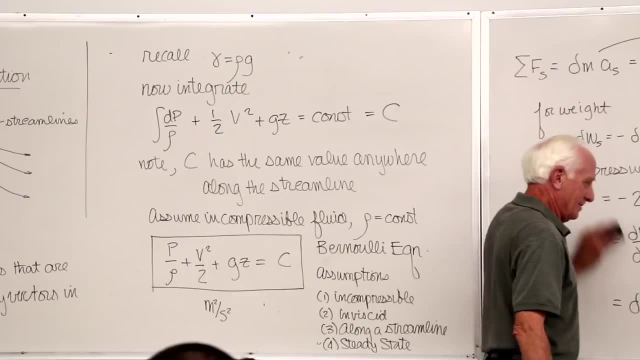 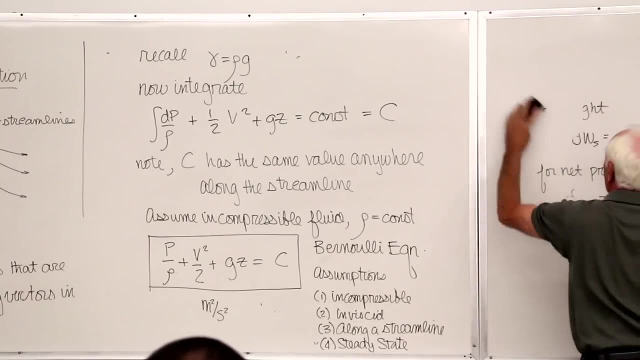 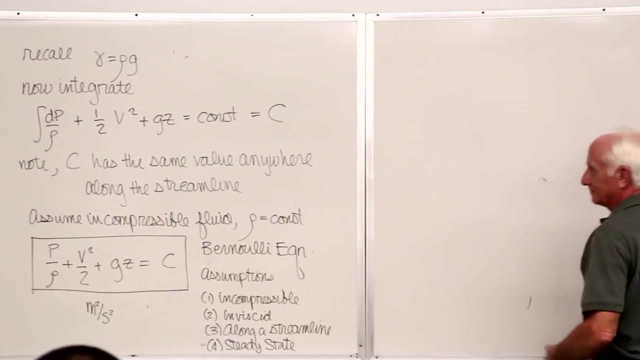 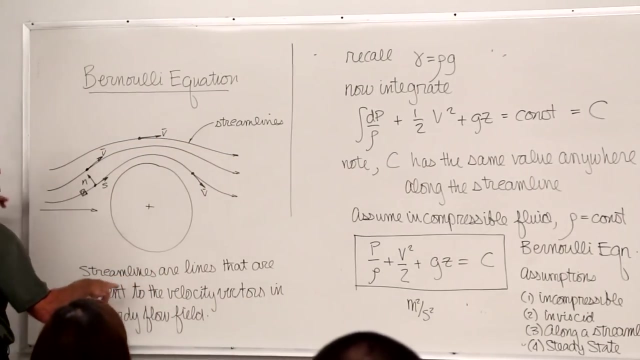 four assumptions are satisfied. oh, there's an exception. oh, there's an exception. oh, there's an exception. later on, but for right now, that's the four that we need. okay, what's a streamline? okay, right here, lines that are tangents of philosophy, vectors at every point, from a steady 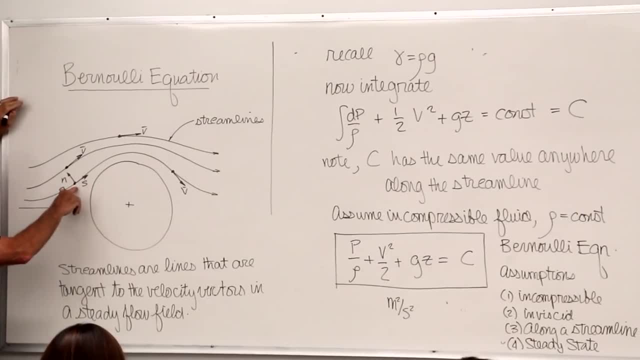 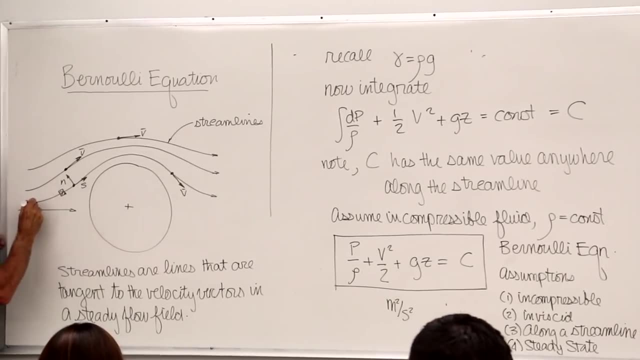 flow alert. the word state okay okay, so a could be a little bit more precise. it has to be applied and it's a streamline. it implies the long a stream line. that equation applies. if you want to call this point one, then you can call this point two and it apply lawness. 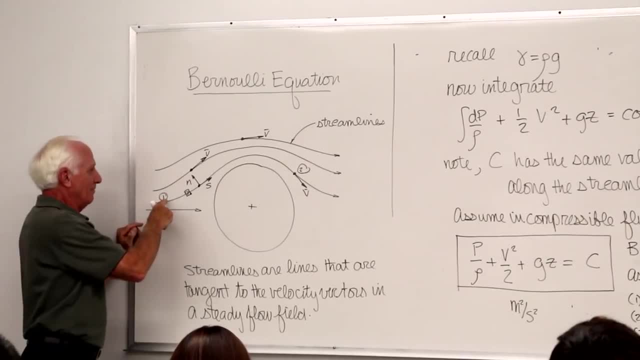 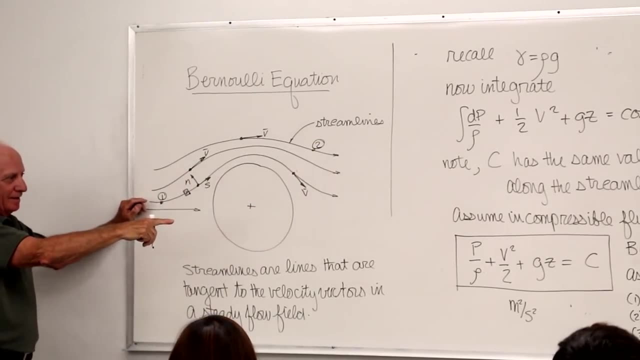 streamlined. here's what you don't want to do. if that's point one, you say I don't like point two, then point two up there. oh no, no, you didn't read the border a well did it. it says it applies along a streamline, not across the. 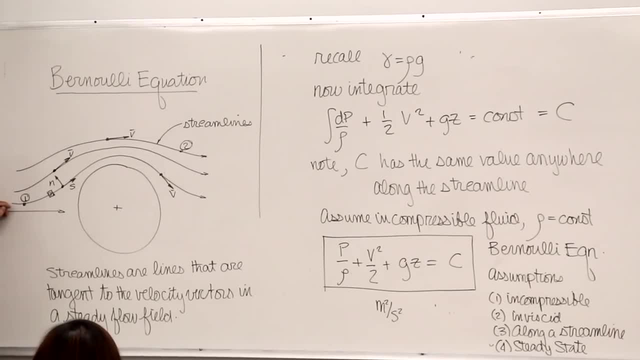 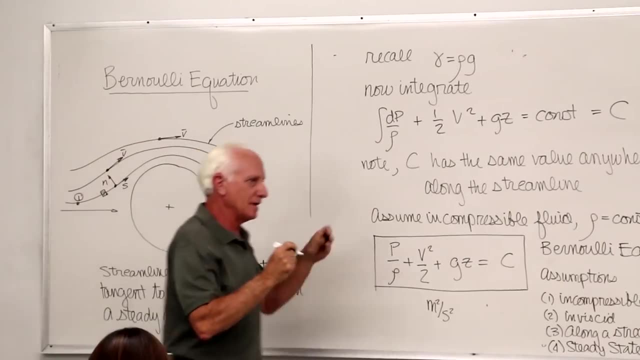 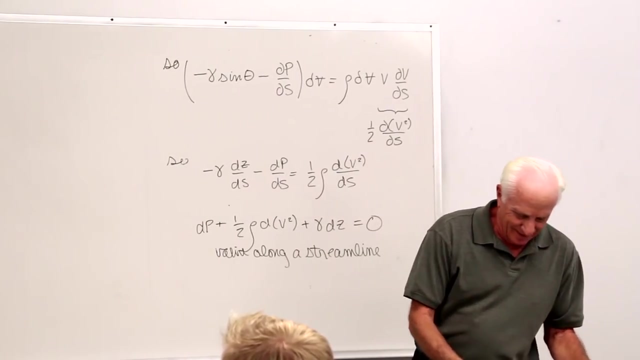 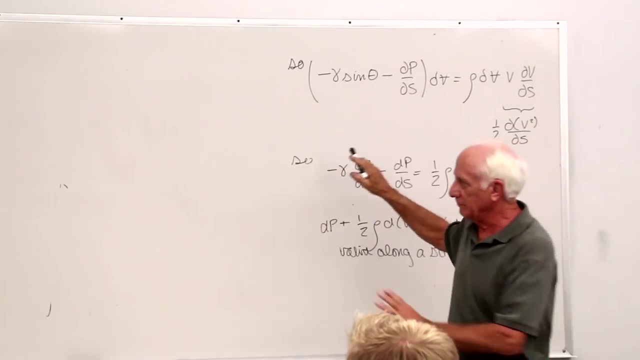 streamline, not across the streamlined it the stream line. so no, you can't do that. point two has to be somewhere along that same stream line to apply the Bernoulli equation. okay, now, if you, if you look at this over here, I'm going to save this middle panel for something else, so I'm. 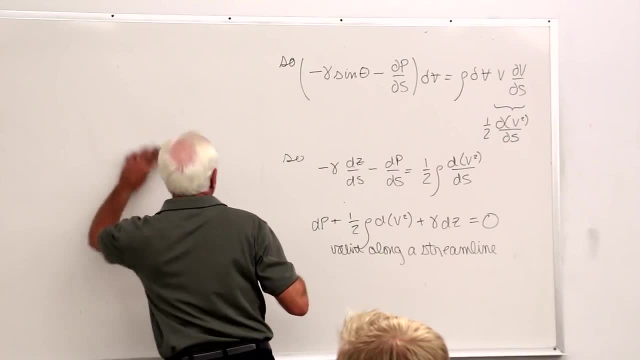 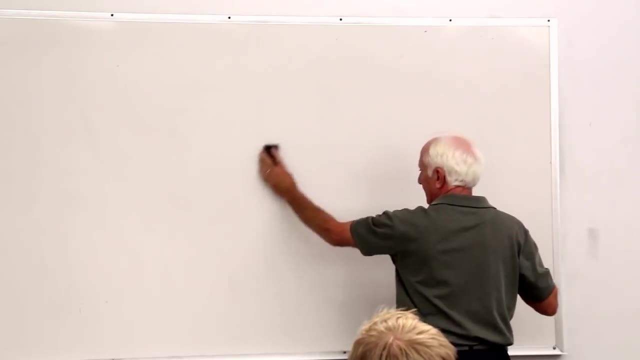 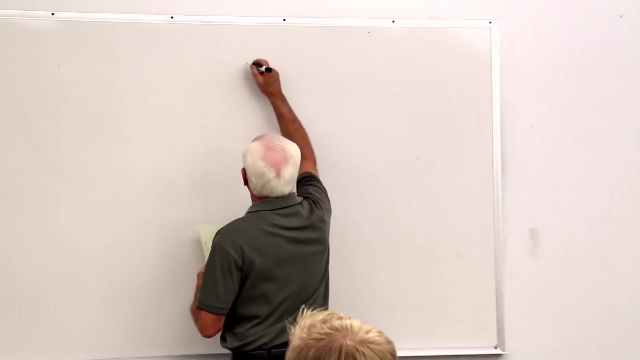 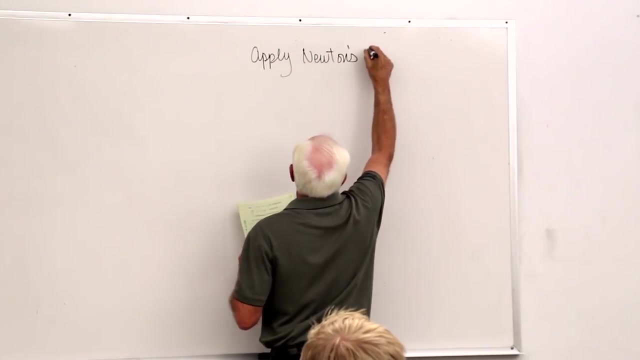 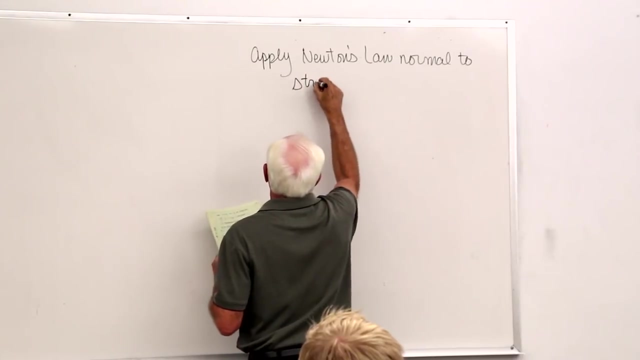 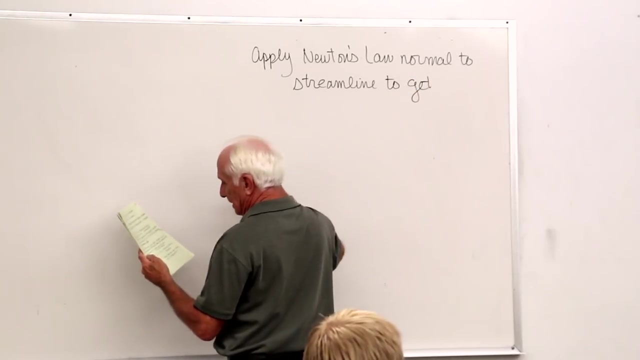 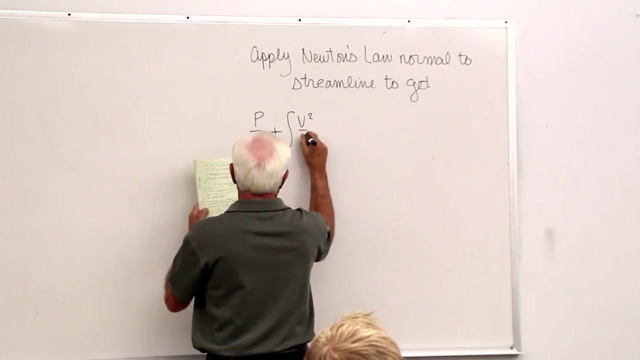 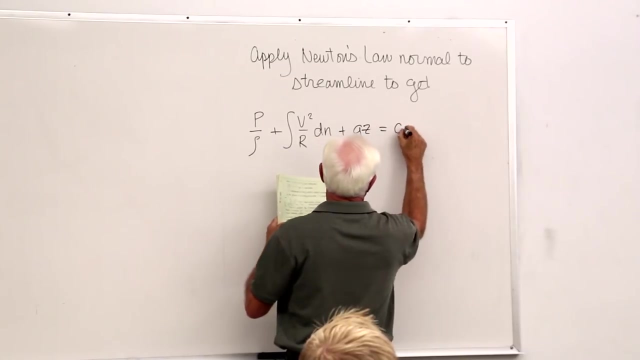 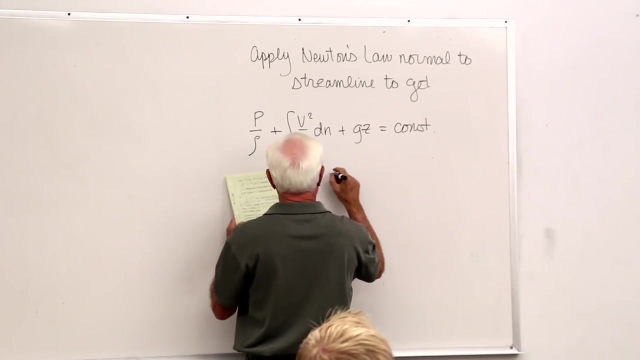 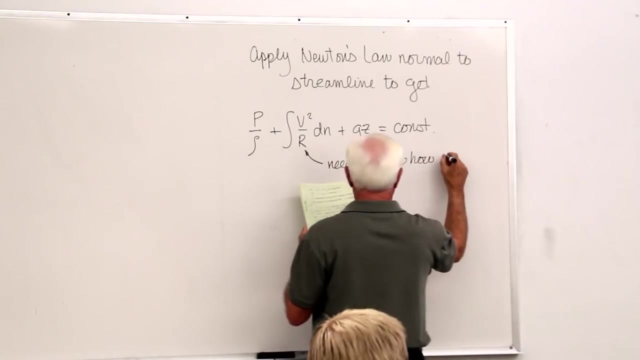 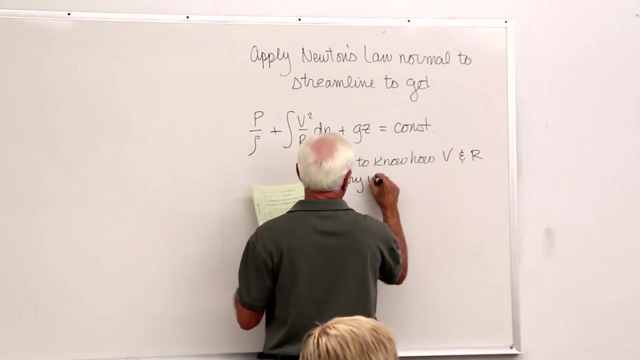 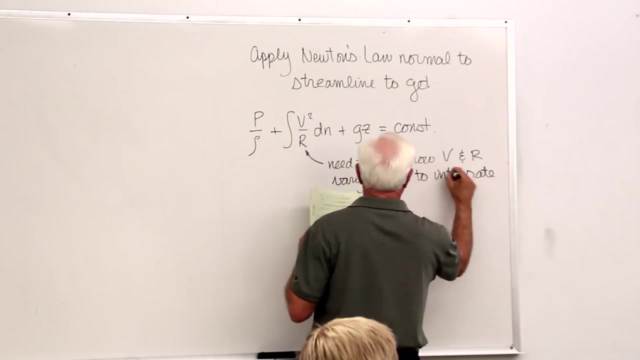 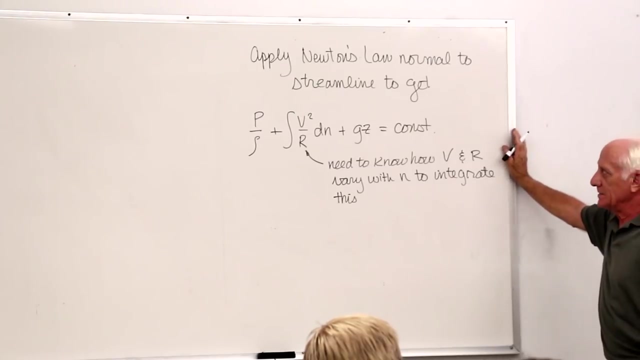 going to erase this and save this place here. you can also apply similar kind of derivation: normal to the stream line, normal to the stream line. if you go through all those details, this is what you end up getting this guy here. radius of curvature: it's more complicated because to integrate that second term, velocity- 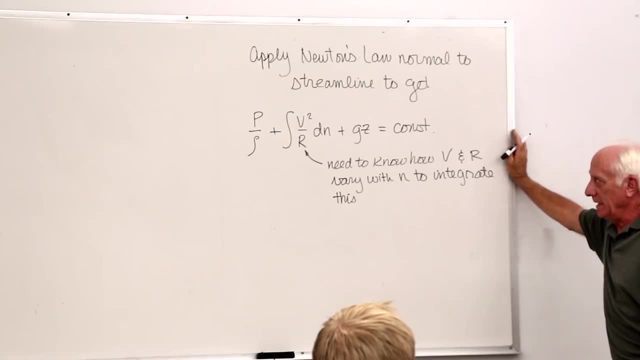 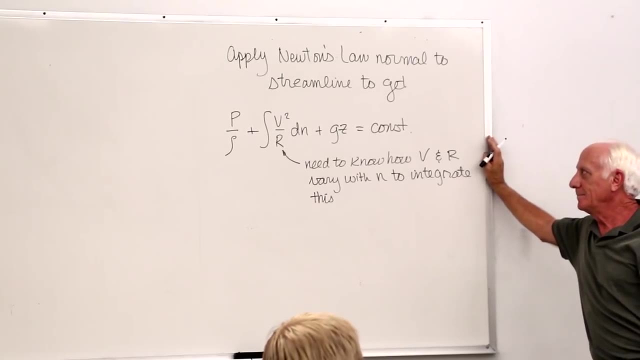 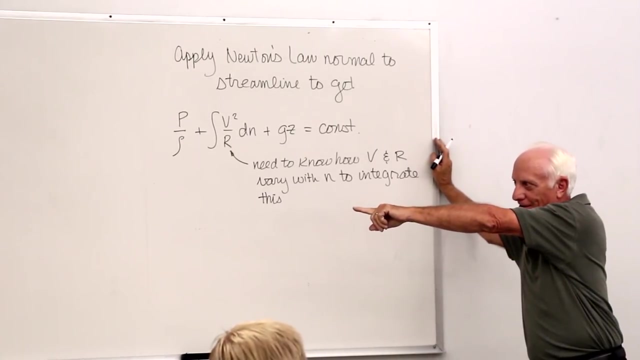 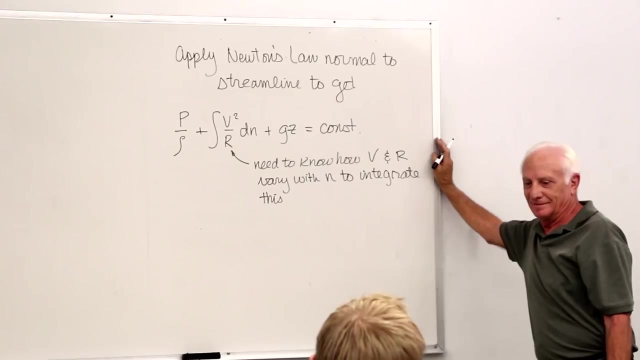 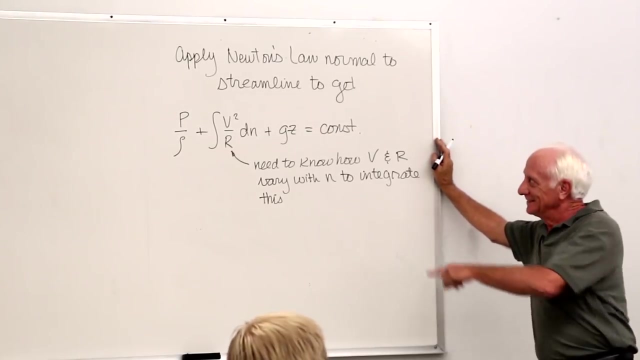 squared, divided by gradient of curvature, DN. you need to know how both B and R vary with N, so that's normal to a stream line that's along the stream line, horizontal flow. what's R infinity? what's one over infinity? if it's horizontal lines, that term drops out. 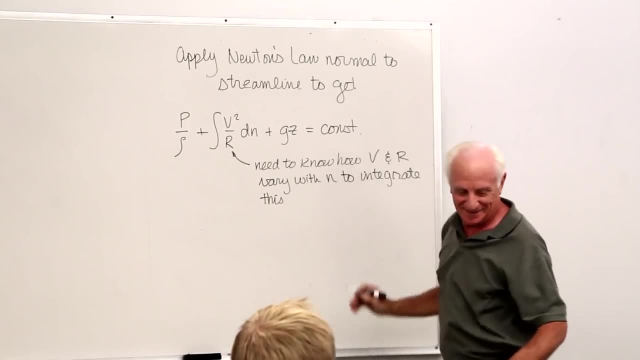 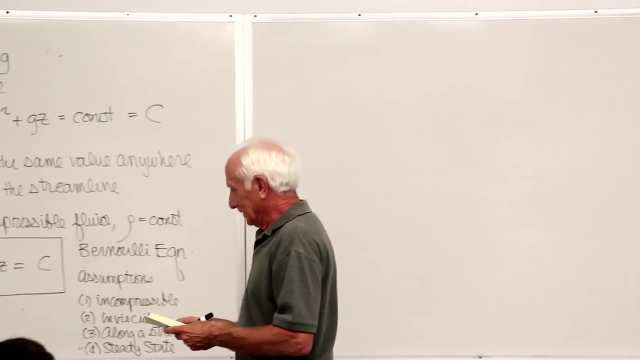 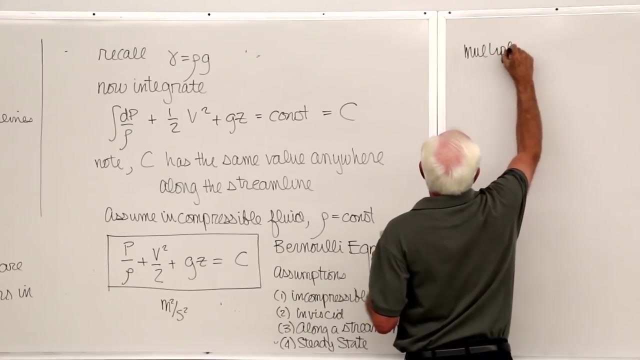 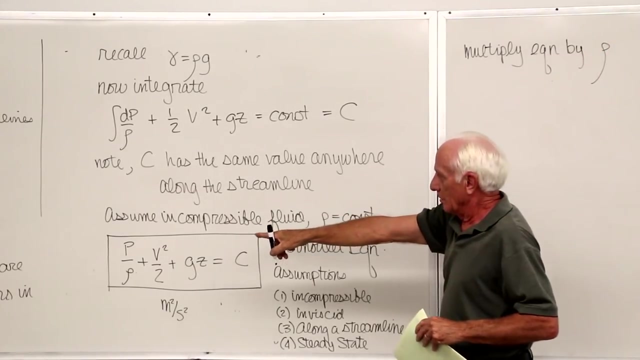 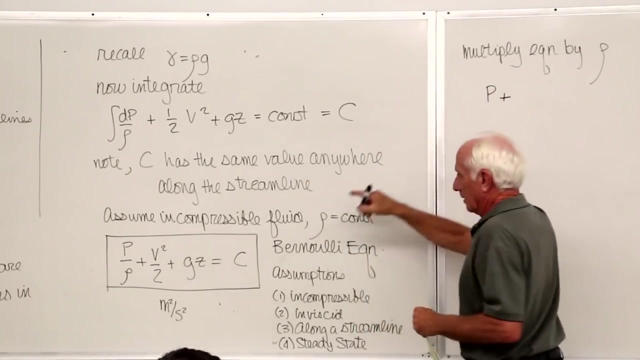 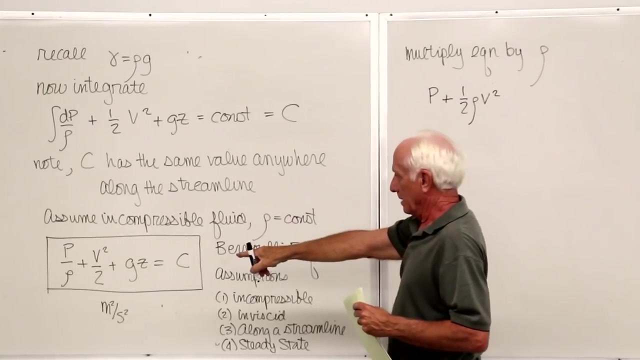 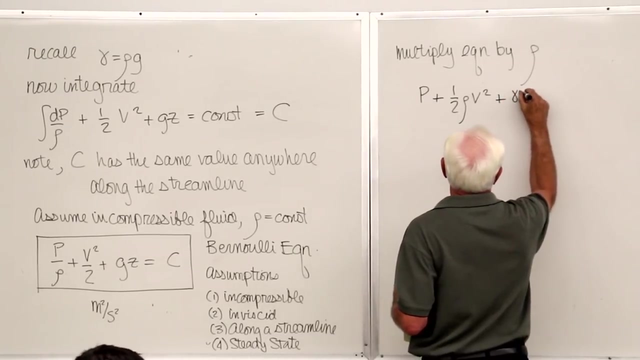 that's the easy case, okay, another form of Bernoulli's multiply through by Rho. okay, okay, row times p divided by Rho. okay, one half Rho b-squared. okay, Rho times G: gamma. Rho times G, gamma. gamma. gamma P, gamma p. 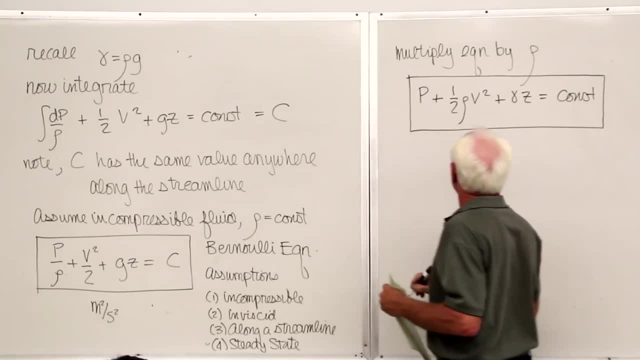 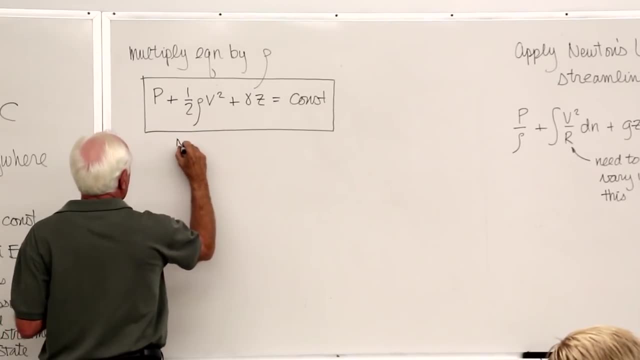 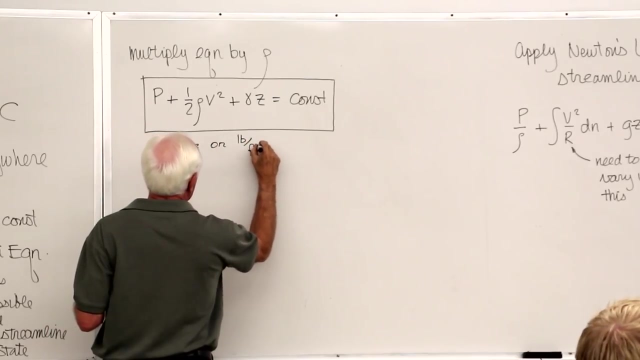 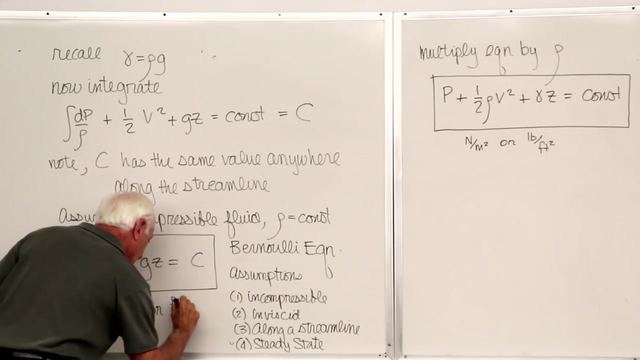 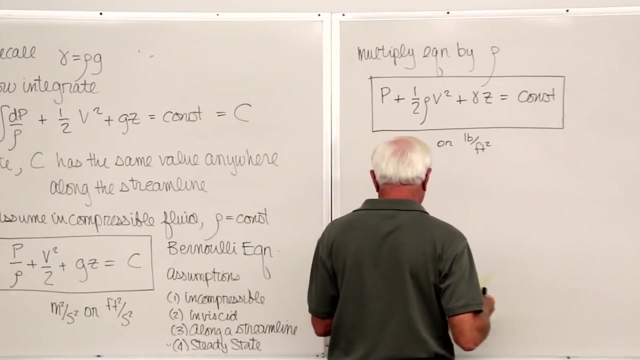 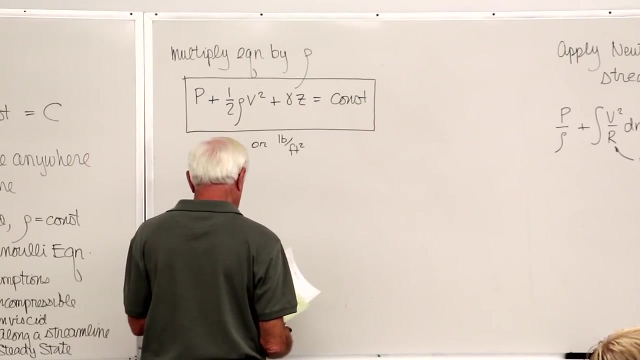 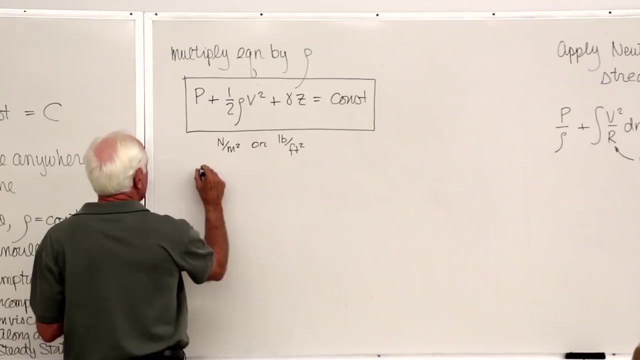 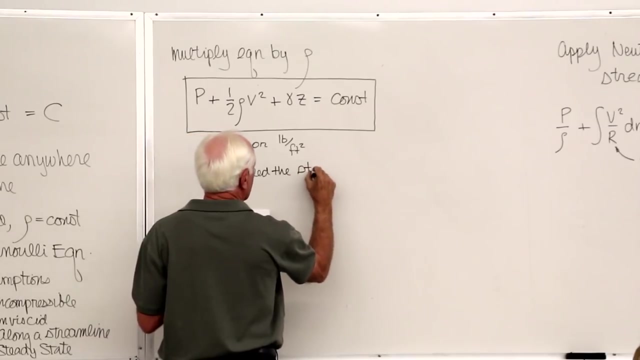 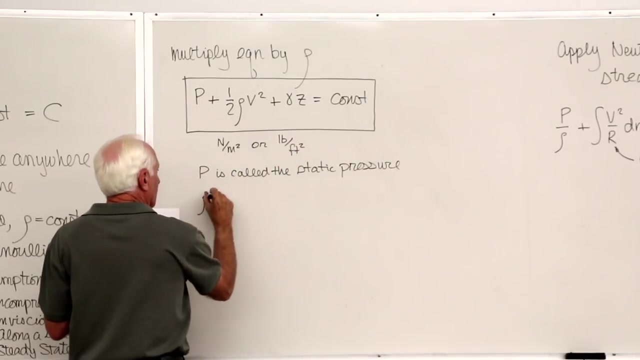 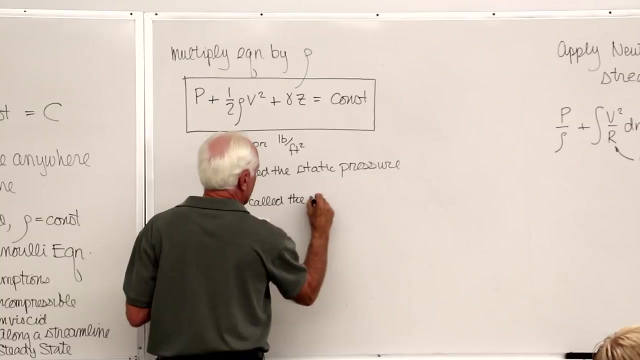 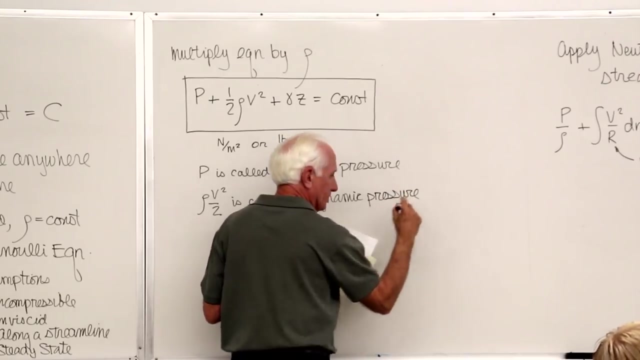 and Y times, p Units, pressure: okay, Okay, On the right. P by itself is called the static pressure. Okay, Okay, Okay. So B squared over 2 is called the dynamic pressure. Of course it depends on velocity, so it's called the dynamic pressure. 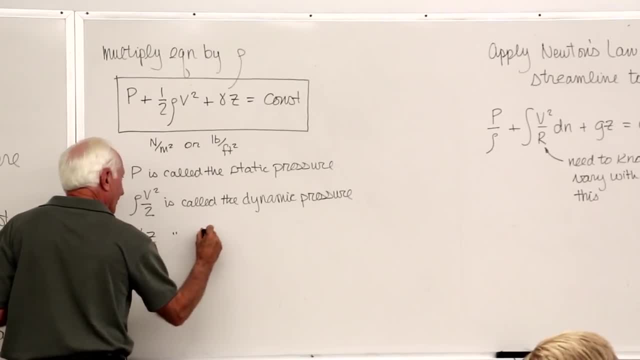 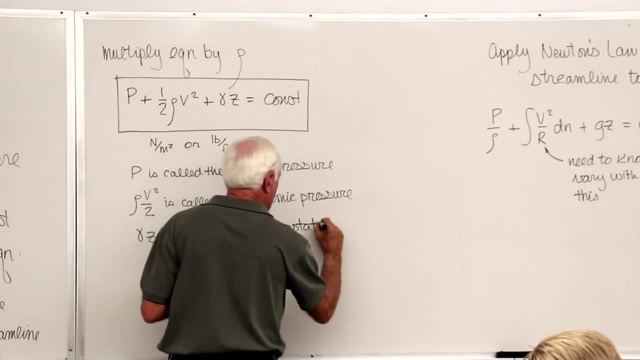 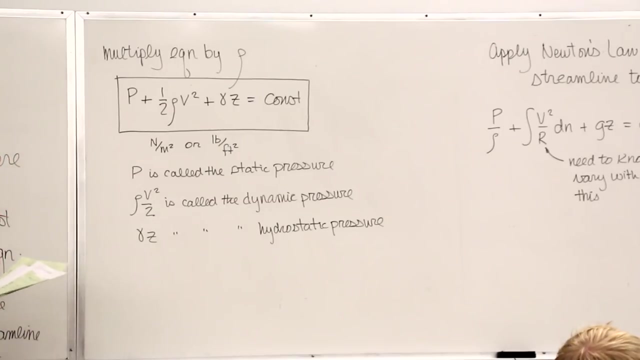 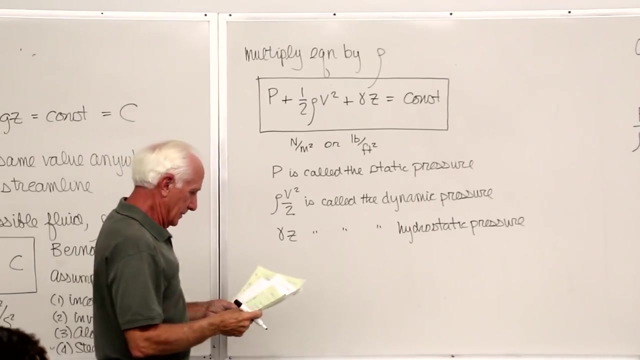 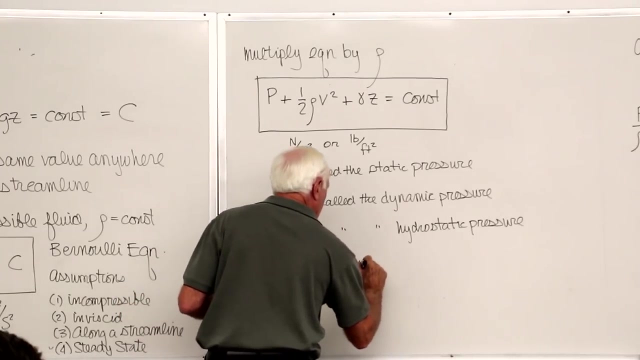 Gamma times Z. Gamma times Z is called the hydrostatic pressure. Gamma times Z is hydrostatic. It depends on the height of your. we did this back in chapter 2.. P plus rho, B, squared over 2, is called the stagnation pressure. 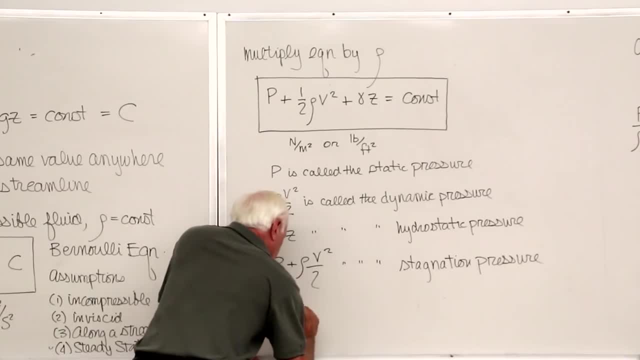 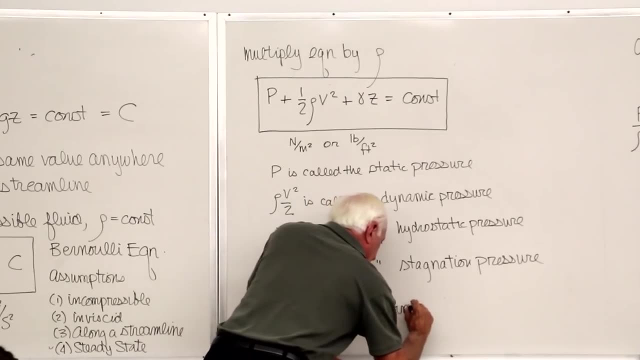 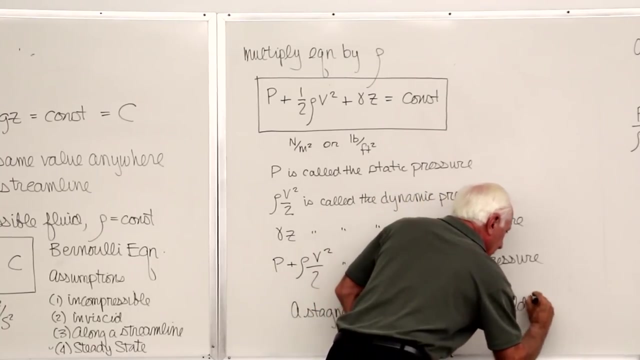 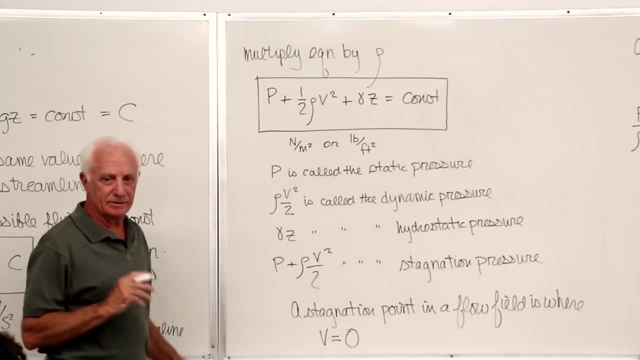 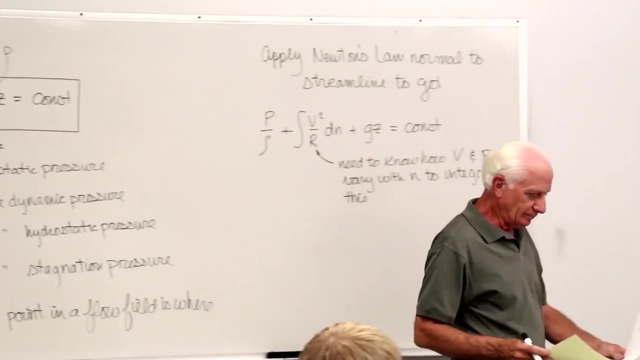 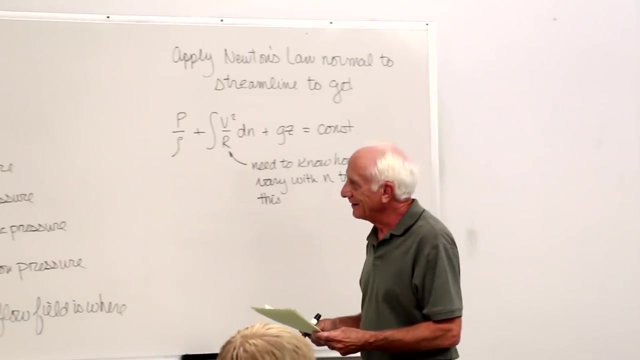 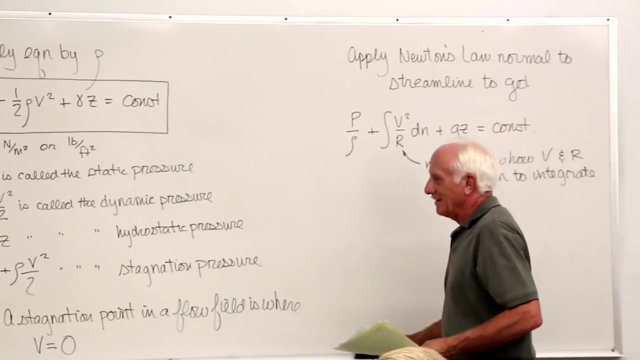 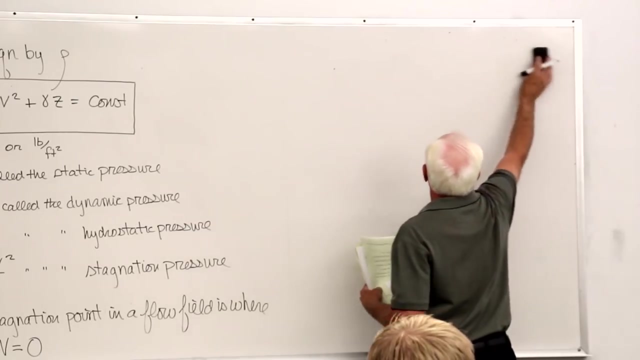 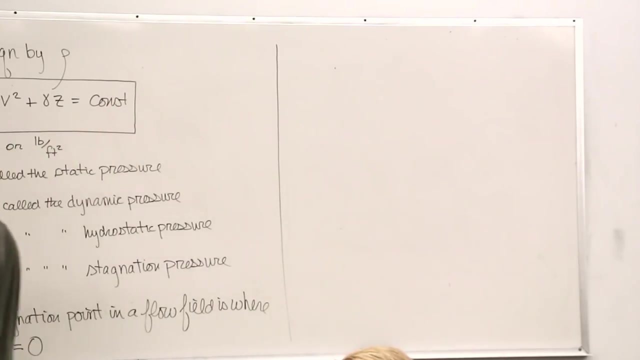 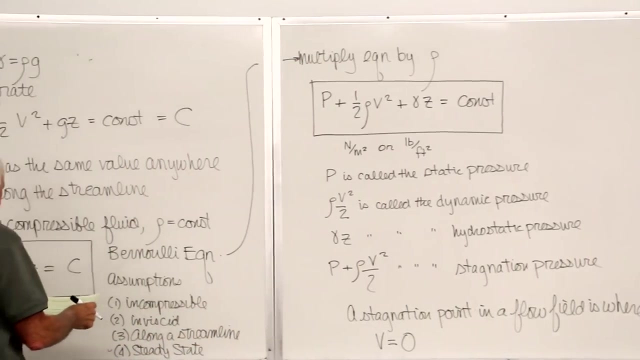 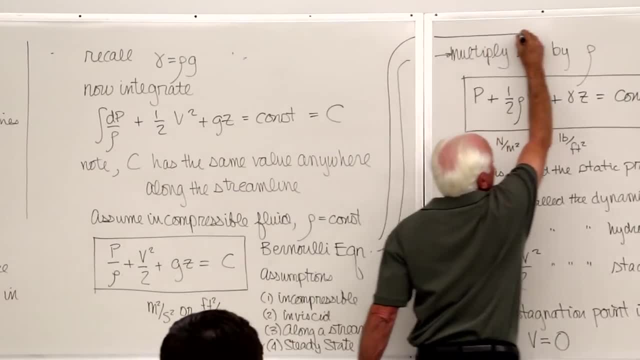 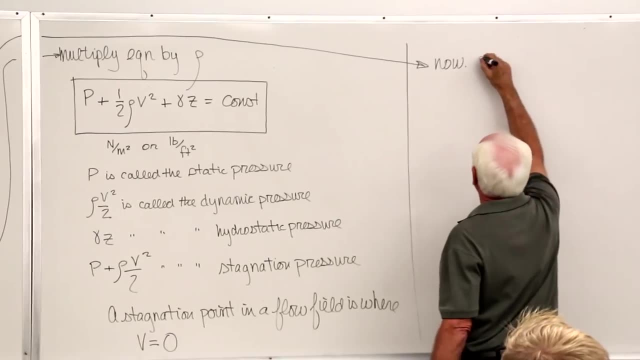 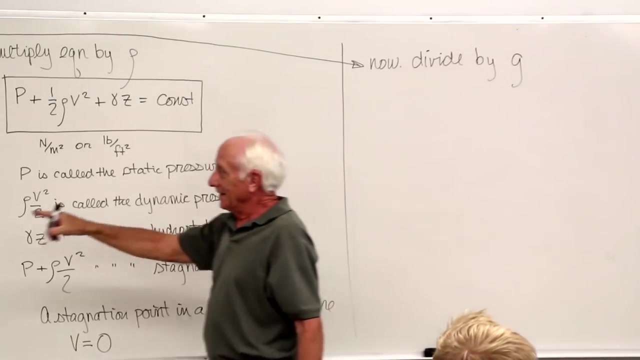 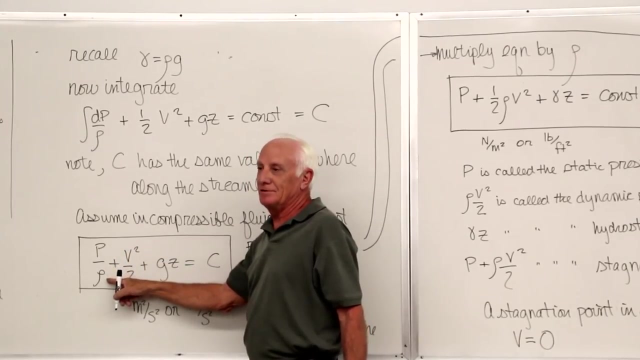 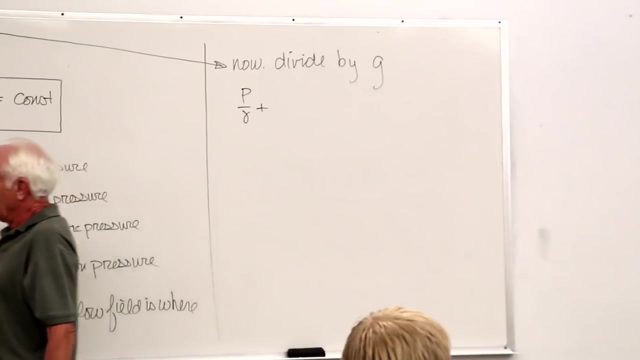 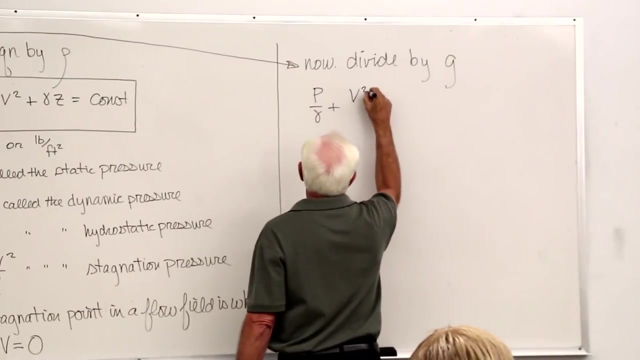 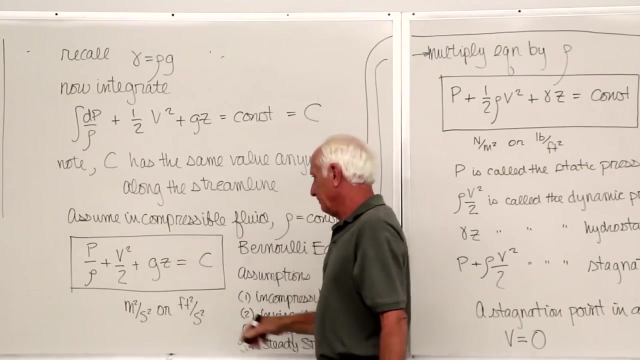 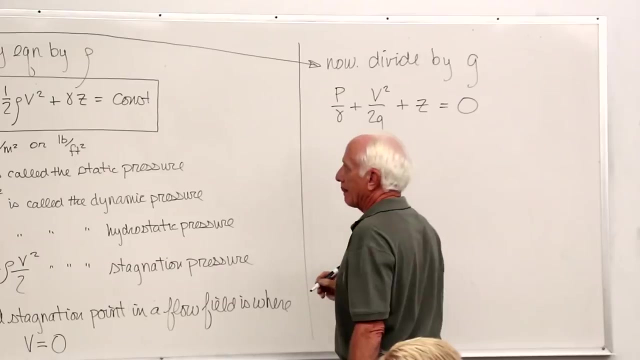 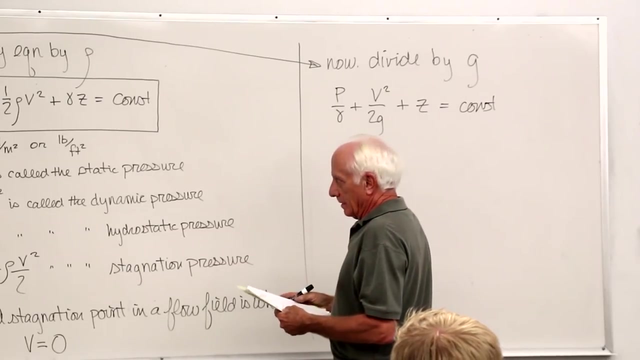 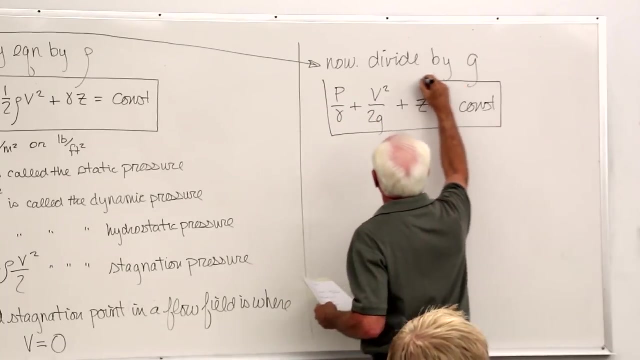 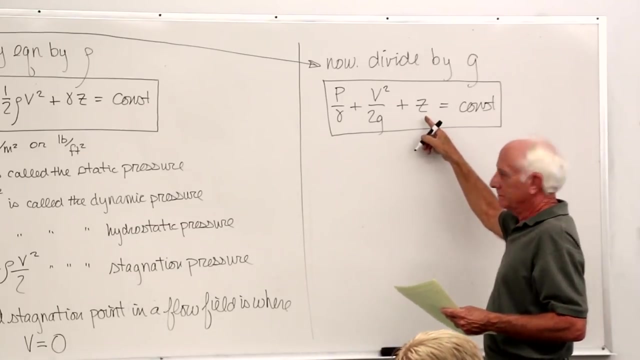 now divide by G. Okay, there it is. Divide by G P divided by row G: Row G is gamma. Divide by G P squared divided by 2G. Divide by G RLZ: Okay, Oxygen Units- I'll take this guy, the third guy. Meters or feet, This is. 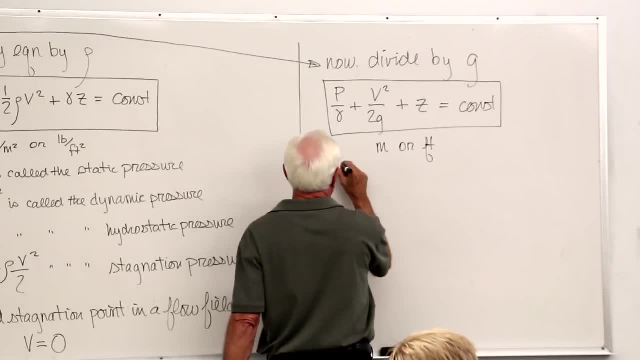 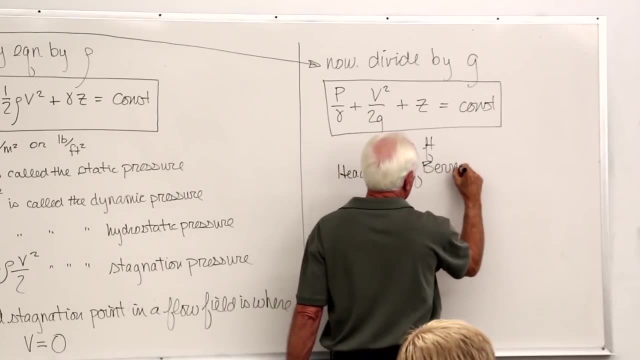 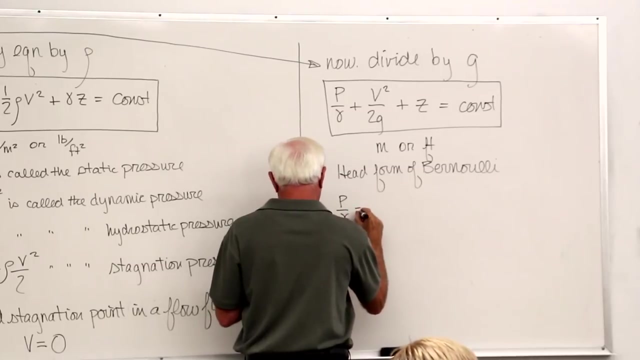 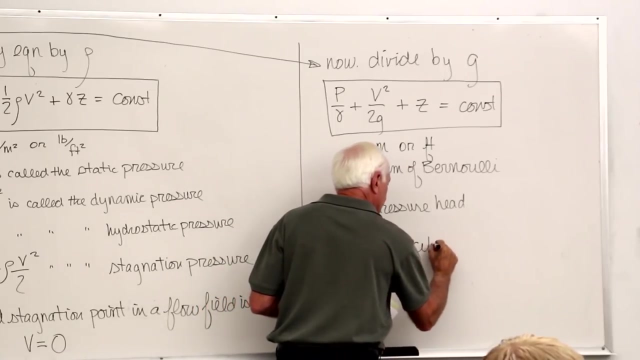 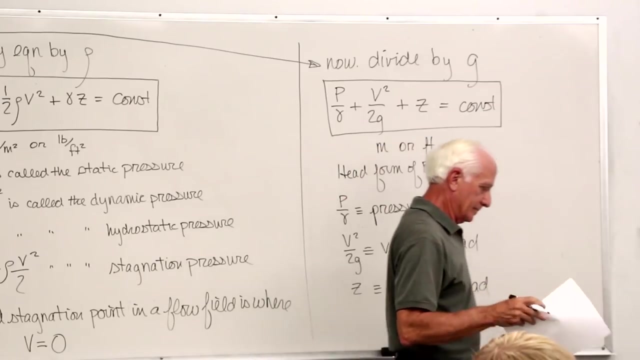 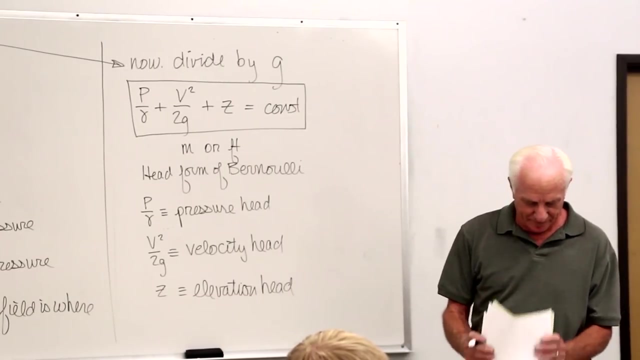 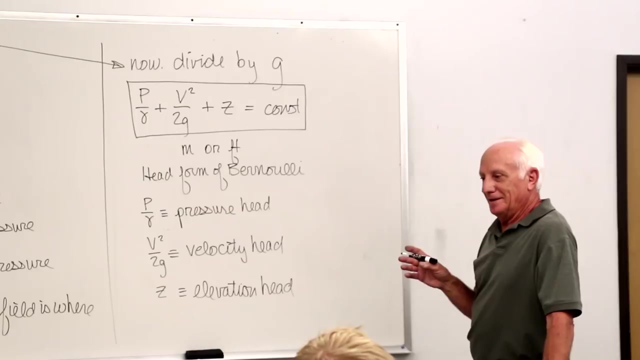 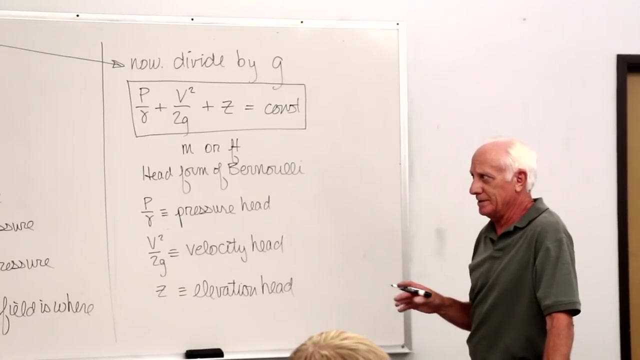 called the head form of Bernoulli: P over gamma Pressure head. V squared over 2G Velocity head. Z- Elevation head. Okay, You got three different forms of Bernoulli equation. They're all the same equation but they're just packaged in different ways. It depends the problem. 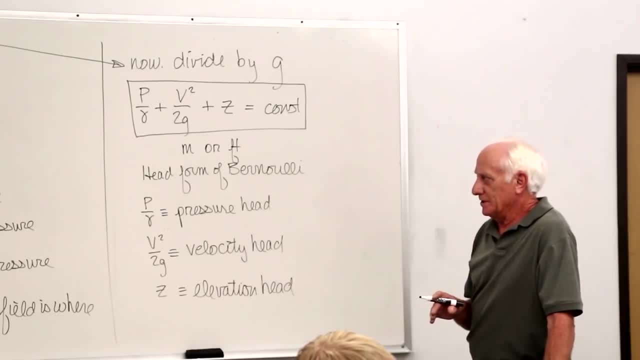 you've got which one you want to use. If somebody asks you for the stagnation pressure, use the middle one, But it's up to you which one you use. Sometimes some are easier than others. If I know, gamma of oil is 8,200, I'll. 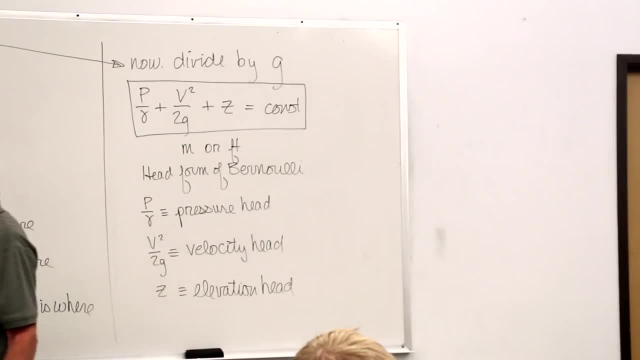 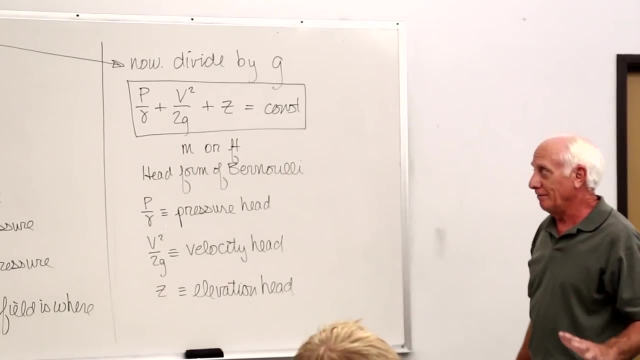 use this guy. I won't try and get rowed. I don't have to. So again, it depends on what's more convenient to you, But they are different. If you want to talk about the equivalent pressures, this guy talks about the equivalent pressures. 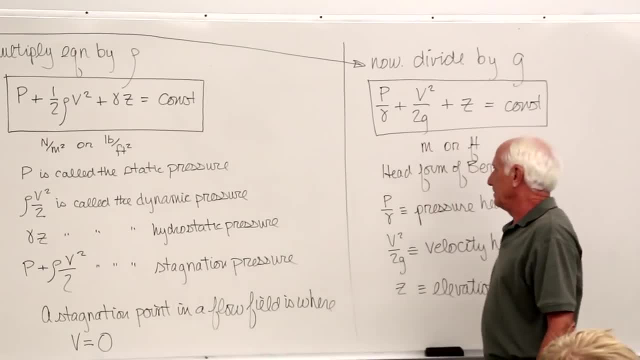 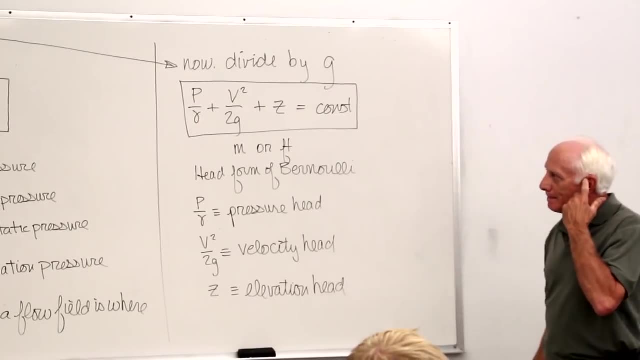 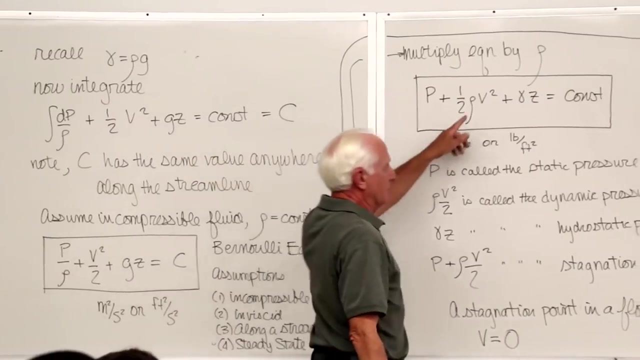 Static, dynamic, hydrostatic stagnation. You want to talk about the head form of the equation, the pressure head, the velocity head, the elevation head. This was the one we derived, so this has rho in it. this has rho in it, this has gamma in it. So it depends. 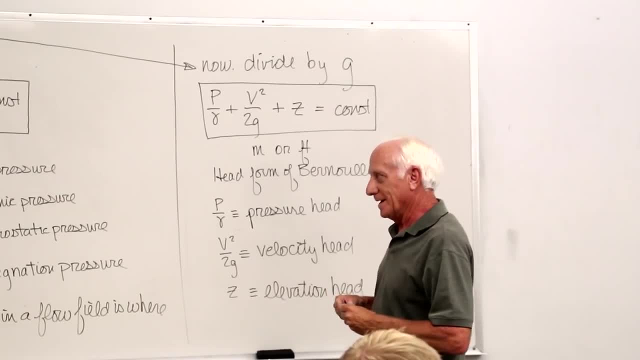 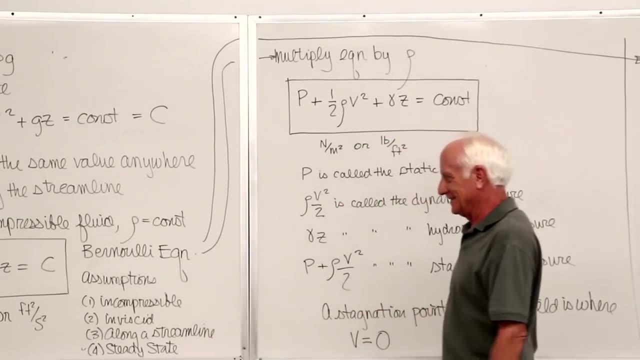 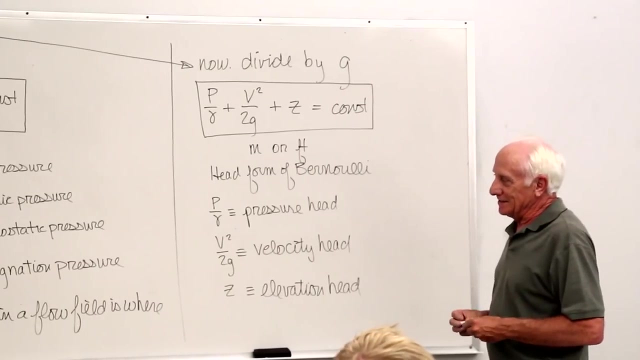 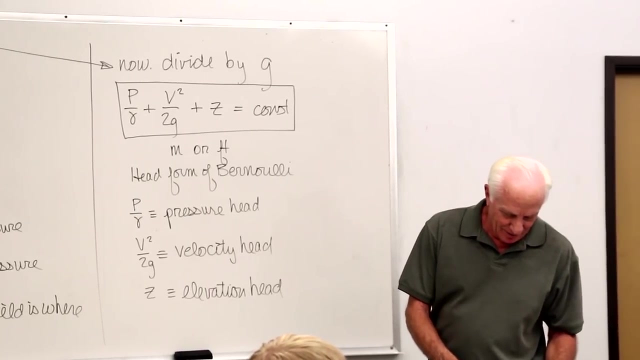 again which one you want to use. But no matter which one you want to use, for right now these four things happen to be satisfied, okay. incompressible fluid in the visit fluid. steady state situation and only applied along a streamline. okay, so let's take a look at a problem. let me see if, uh. 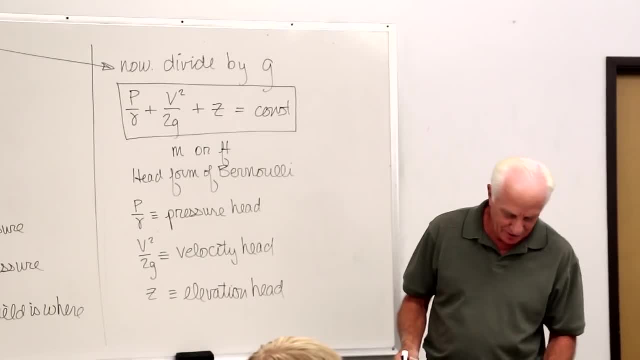 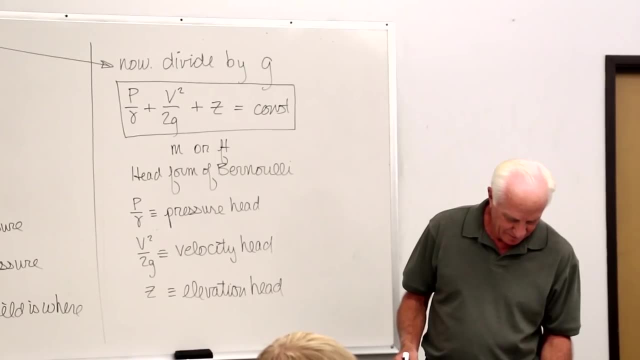 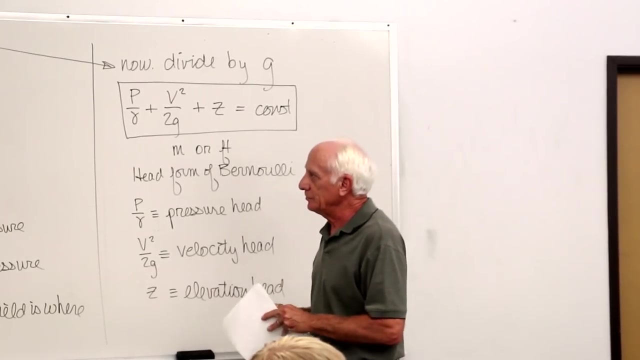 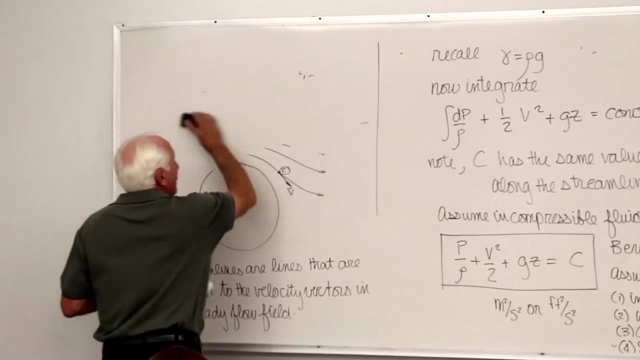 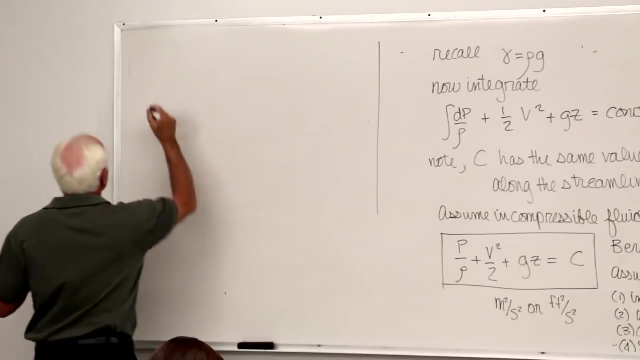 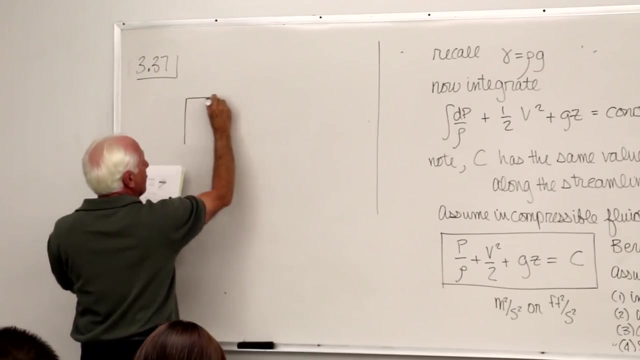 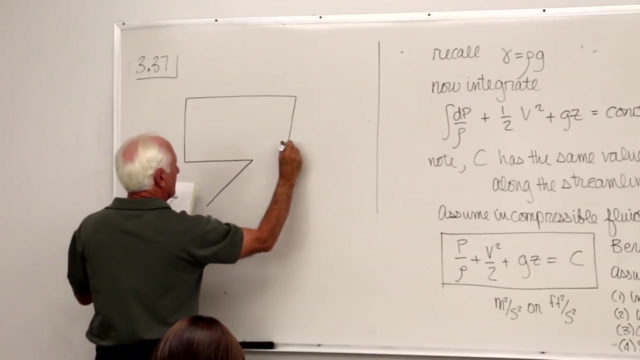 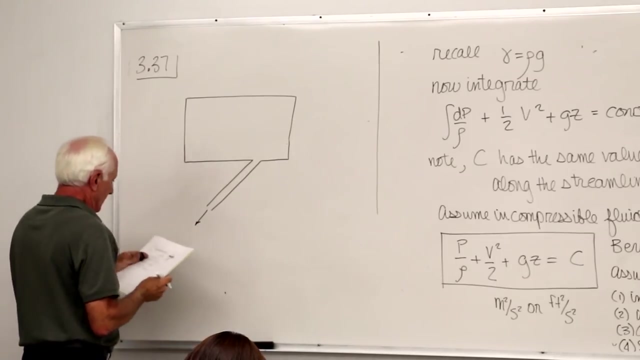 yeah, that's in our book 337, so i'll do 337, put it over here. all right, here we have a tank which is pressurized. let's see what that is. that comes out of there, okay, okay, and in this is what it says. now an inviscid, incompressible liquid flows steadily. 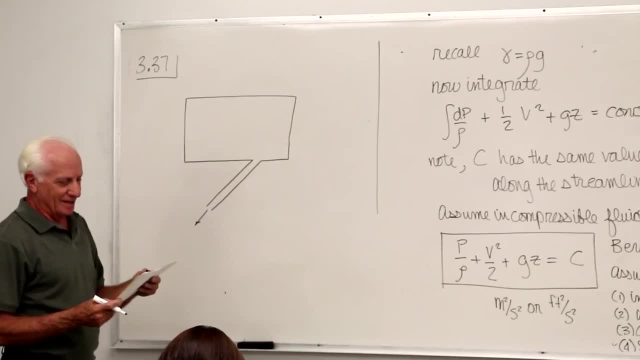 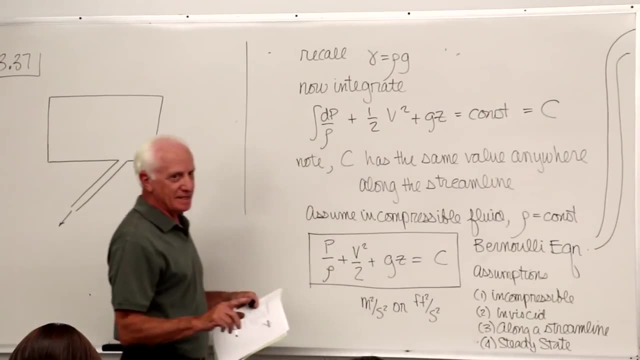 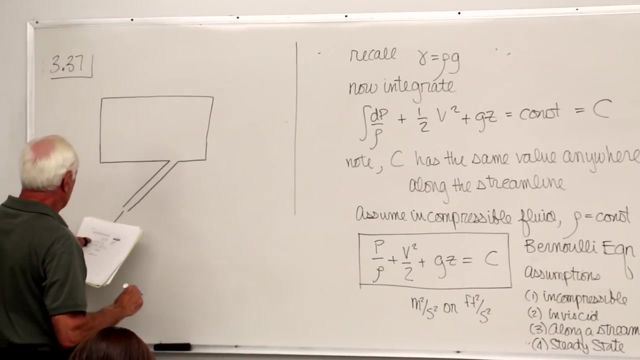 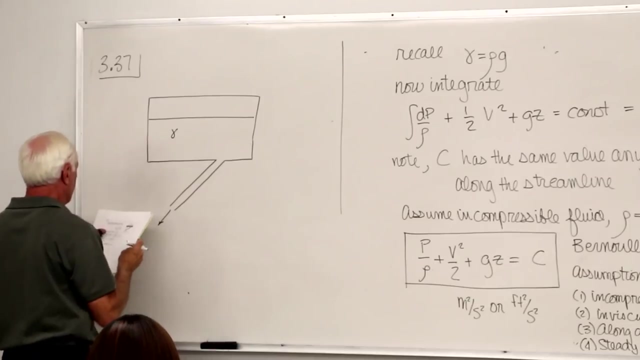 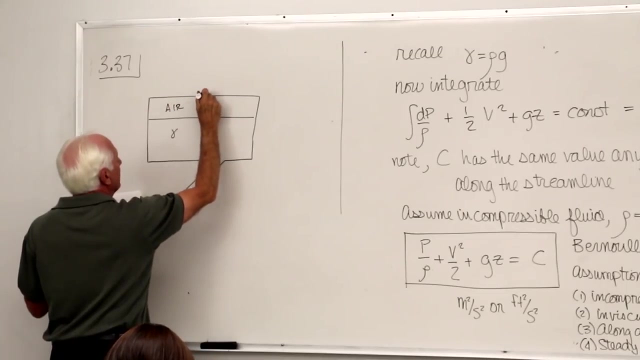 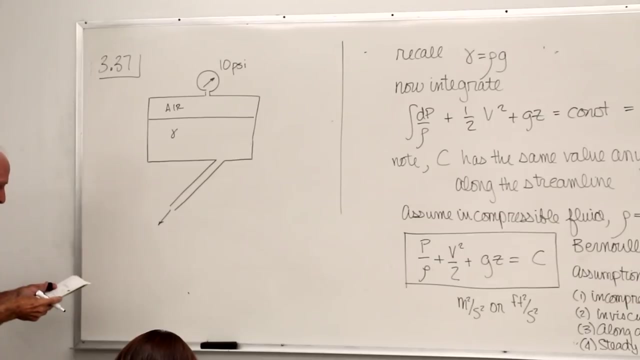 first six words: major giveaway and visit: incompressible flow, steadily okay. yes, yes, yes, not three yet, not three yet we'll get there. okay, in this tank is a liquid gas gamma pressurized tank. air pressure gauge: 10 psi. velocity at the exit: 40 feet per second. 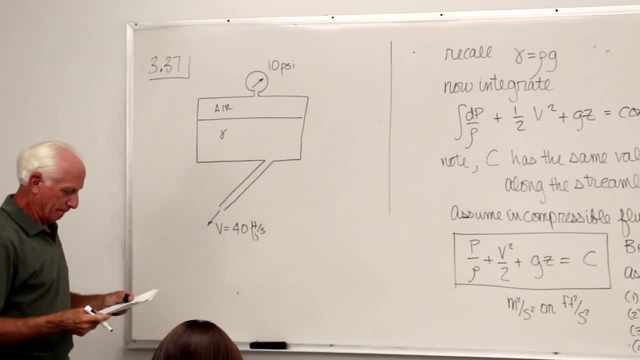 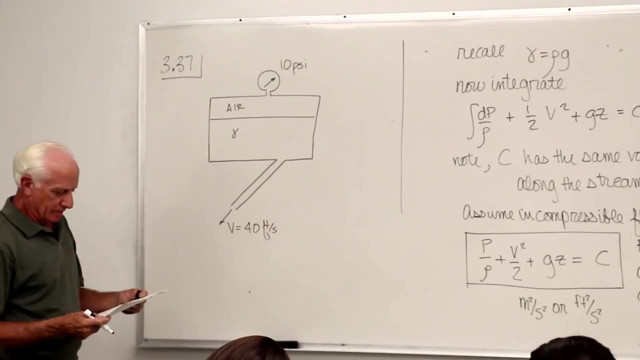 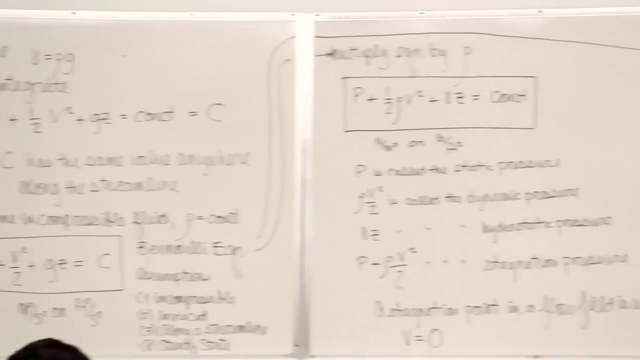 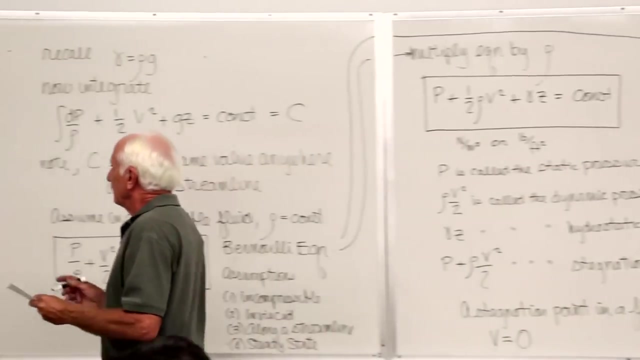 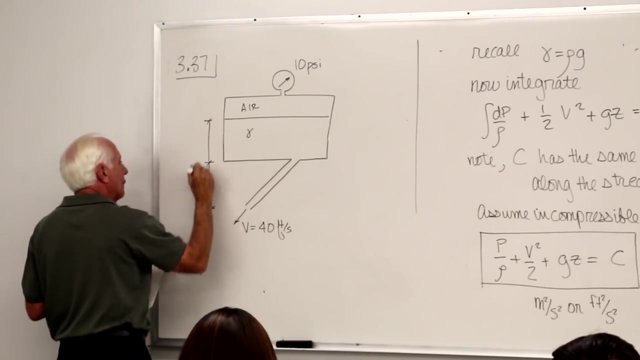 uh, 16, about 16 feet. i'm not sure i've got 15 of them down here. oh, i'm sorry, 10 feet, 10 feet, 5 feet, so 10 feet from here to here and five feet from here to here. okay, basically, the initial density is really important. 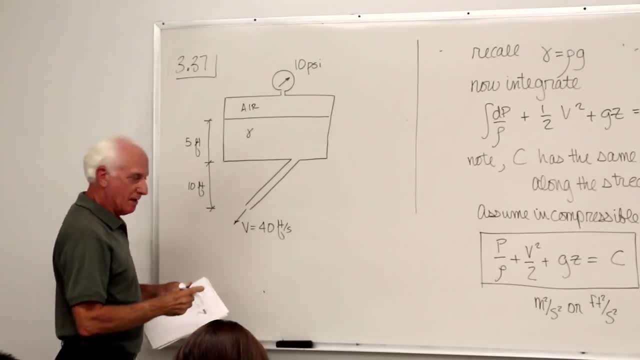 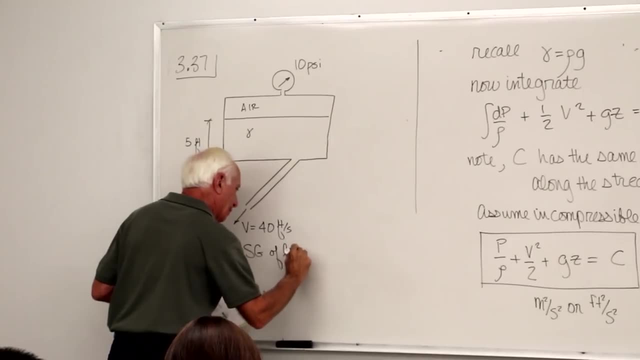 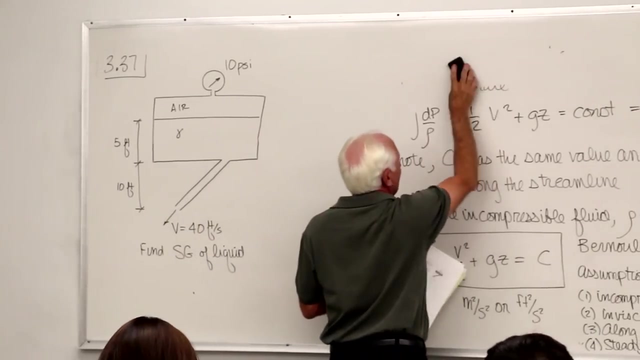 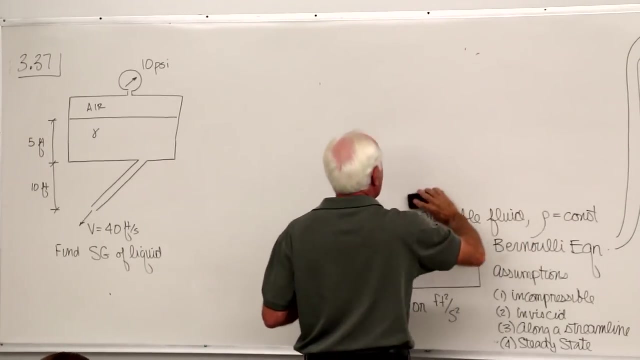 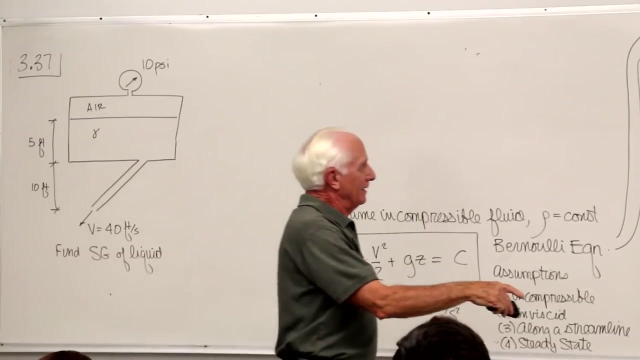 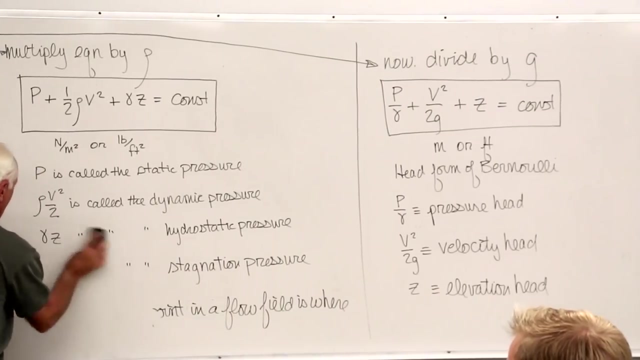 10 and the velocity of the liquidаться. absolutely go. okay. what is the specific gravity of reheating the tank? so find the specific gravity of the liquid. okay, I could use any one of those two. I like to use that one, so I'll use that one, unless there's a reason not to. 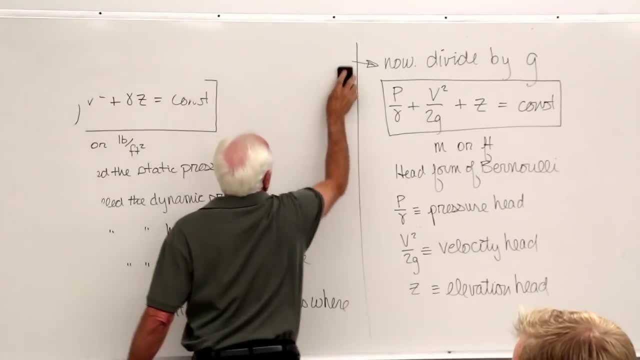 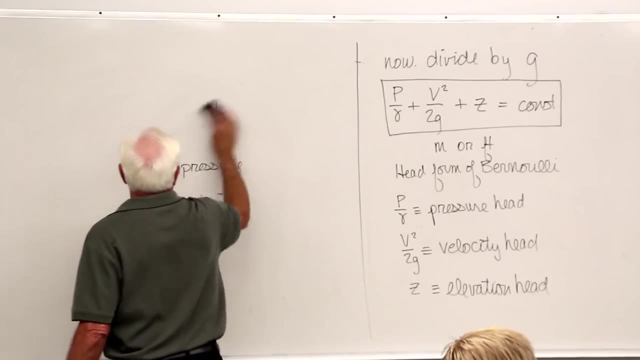 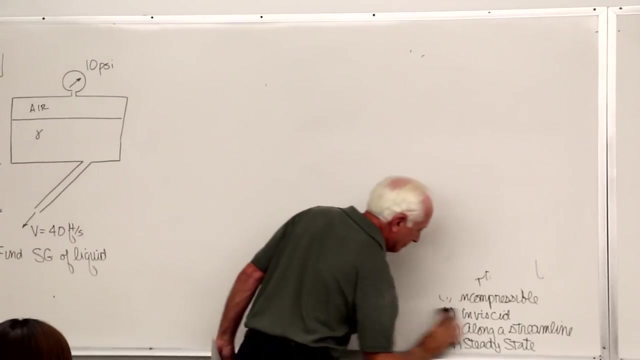 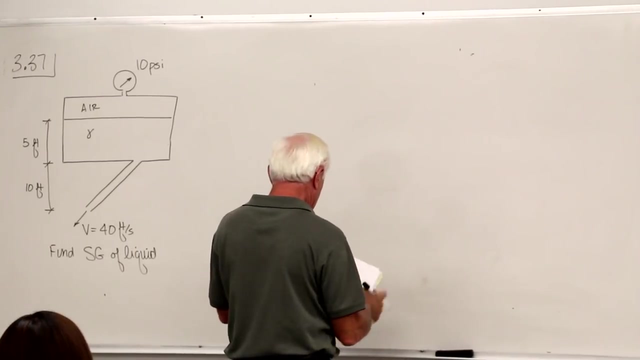 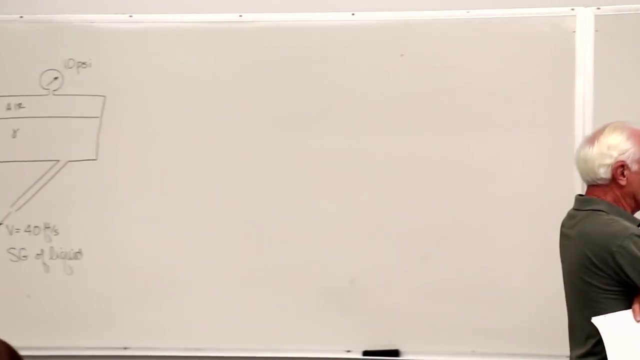 So let's get rid of this one and let's get rid of the other one, and we'll just leave this one on the board. This is the head form of the Bernoulli equation. Okay, so when you want to apply the Bernoulli equation, you're going to apply it between: 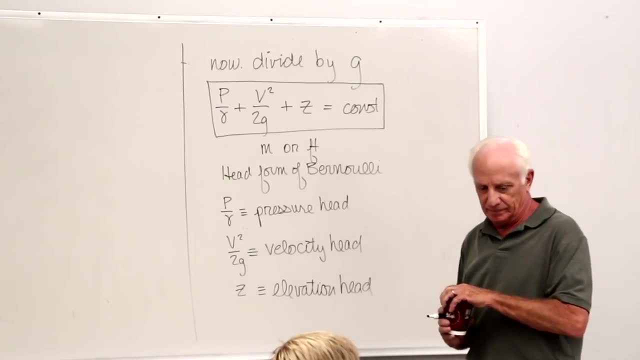 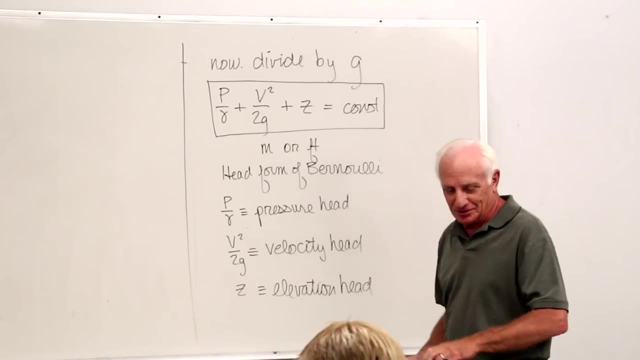 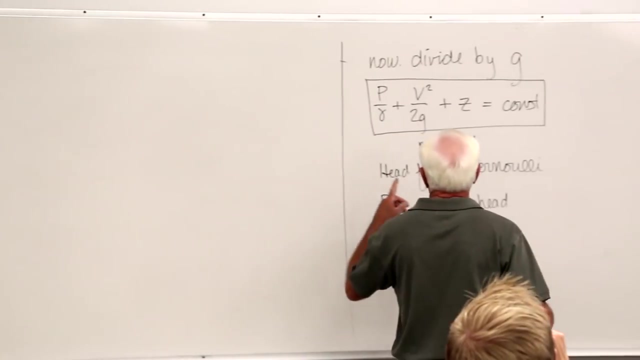 two points in the flow field. Two points in the flow field. You want to choose those two points so that you know the most stuff about the problem. You say, okay, if I choose a point, can I find P, B or Z there? 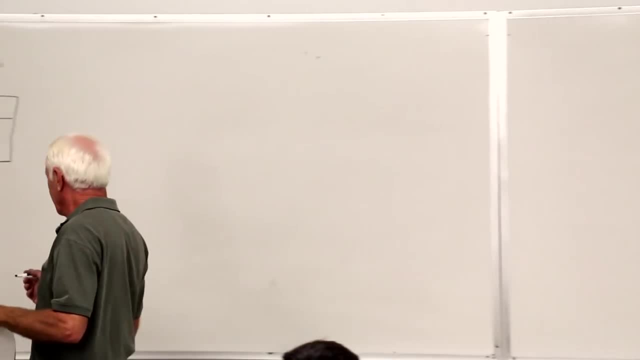 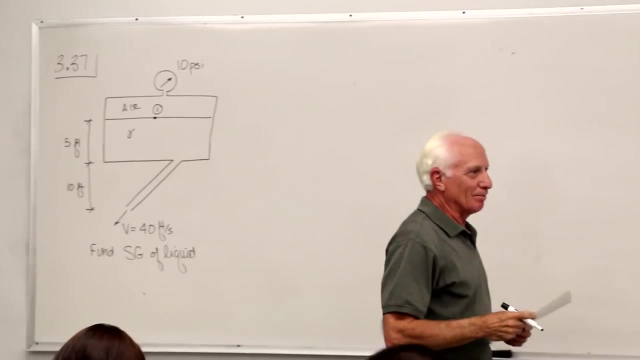 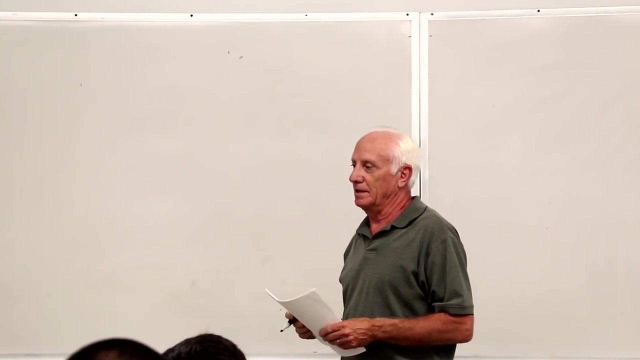 And of course I'm going to give you the obvious point first. I'm going to choose point one here. Why would I do that? Because I know what the pressure is: It's 10.. I know what the velocity is: It's a free surface zero. 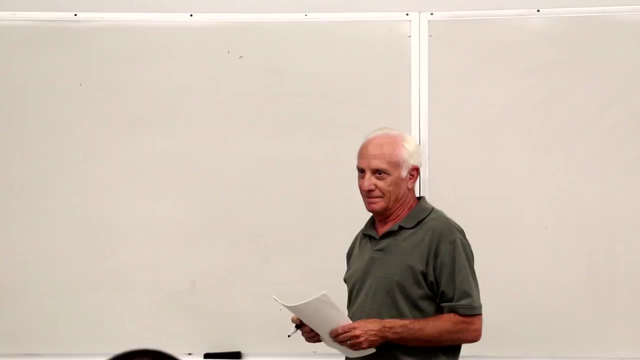 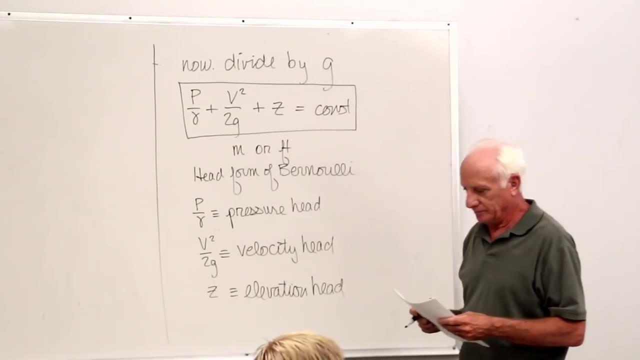 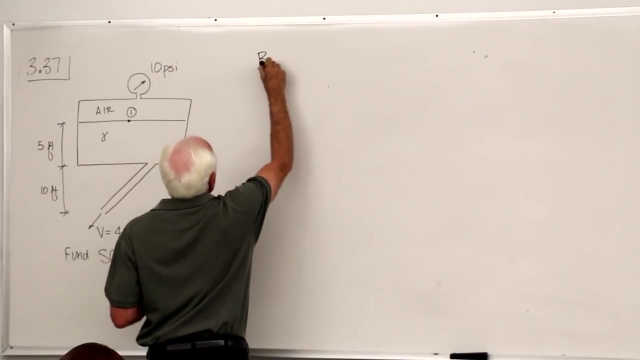 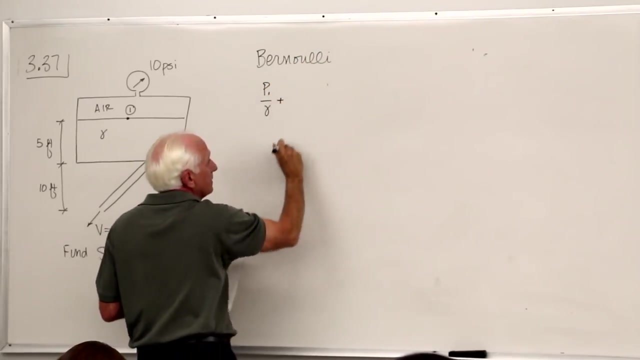 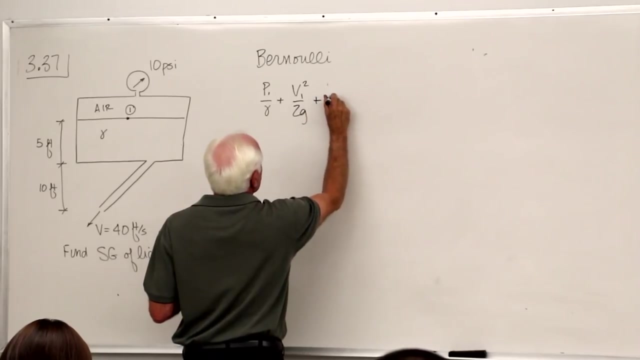 I know how far above the exit it is: It's 15 feet. That's how you decide where to put point one, where you know the most information. So I'm going to write down that equation. Put the subscript one P1 over gamma plus B1, squared 2G plus Z1.. 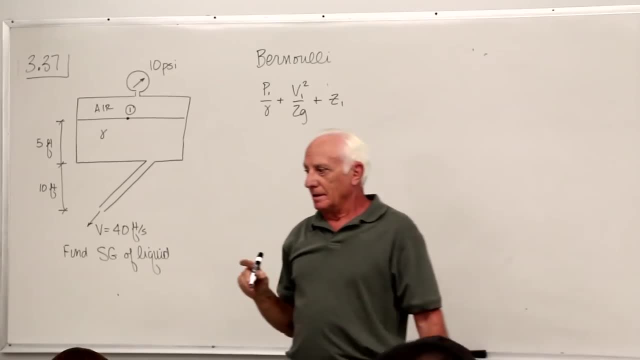 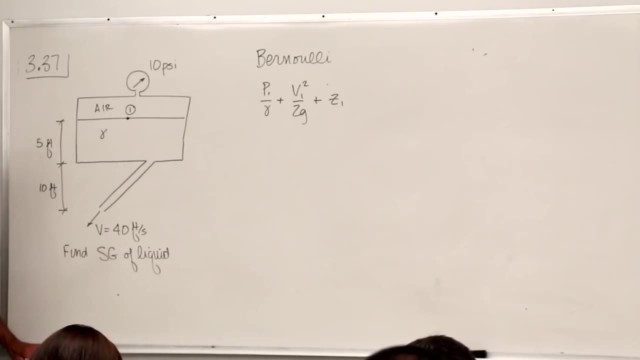 Okay, now I go along a streamline until I find a point where I know some more stuff. Oh, I know this point. down here It's 15 feet below the free surface. Oh, I know the velocity here: 40 feet per second. 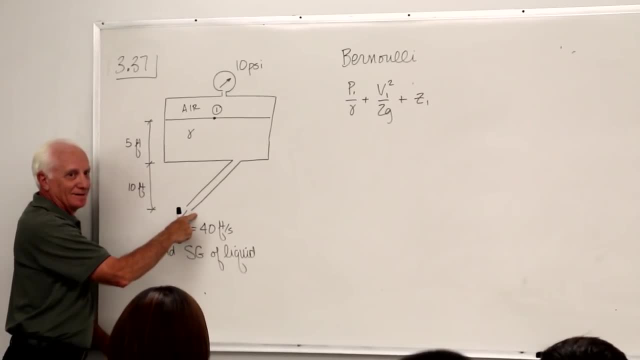 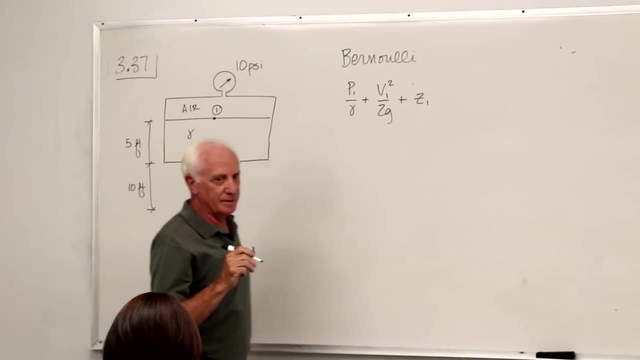 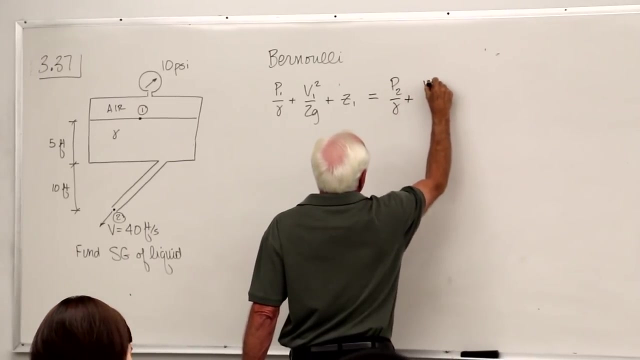 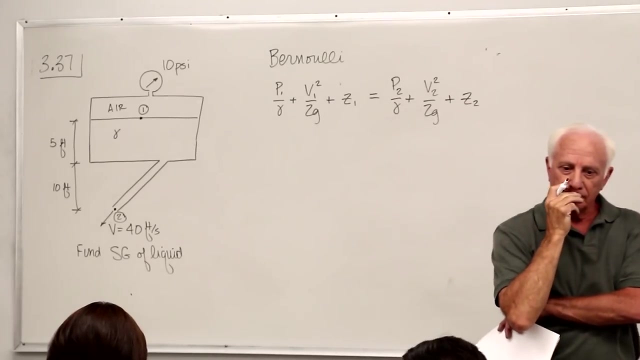 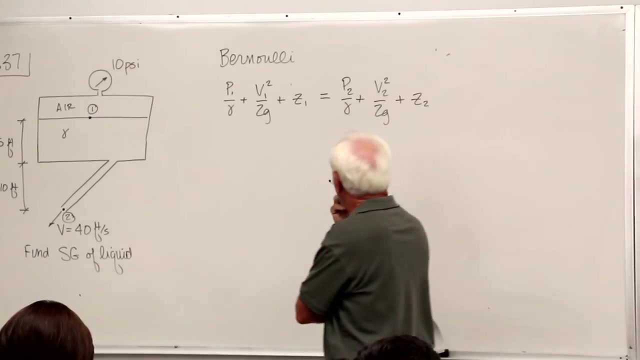 Oh, I know the pressure here. It's zero, Voila. That's point two. I know three things there. Now there's the Bernoulli equation applied between points one and two. All right, let's put the zero stuff in first. 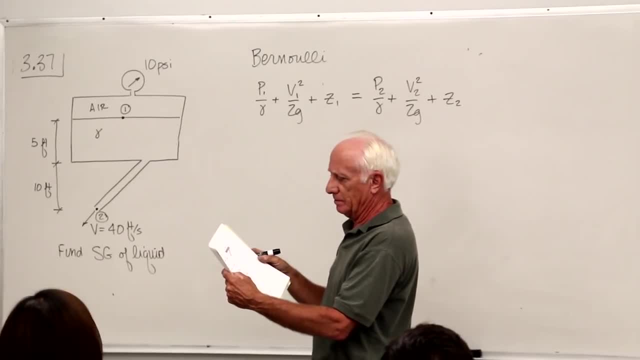 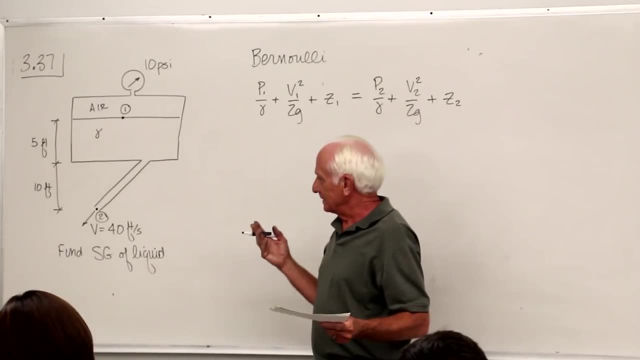 P2, exhaust to atmosphere. Why do I know that It shows in the picture? It shows the pipe ending and the velocity vector coming out of that pipe. That means you always assume in that situation that it's exiting to atmospheric pressure. P2, zero. 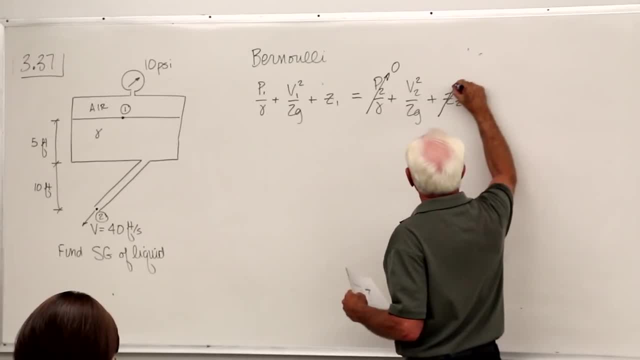 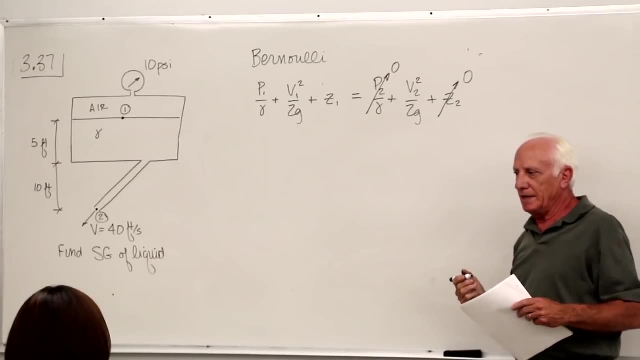 I'm going to call Z2, zero. That's my choice. That's called the datum D-A-T-U-M. D-A-T-U-M- Datum, Where you measure things from If you're in a plant, a factory or a plant. the datum is typically the floor of the plant. 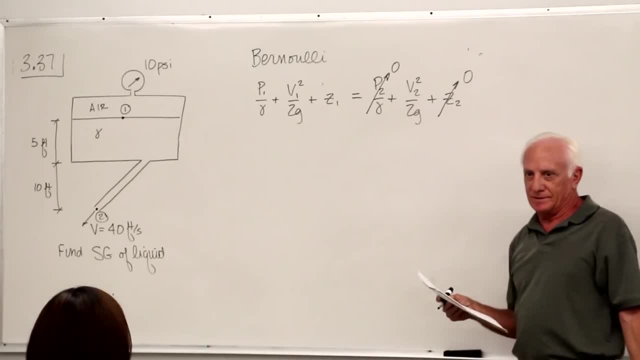 How high is the water tank above the floor? 30 feet, et cetera, et cetera. So the datum You're free to choose. You can take the top, I don't care. Take point one. I'm taking point two. 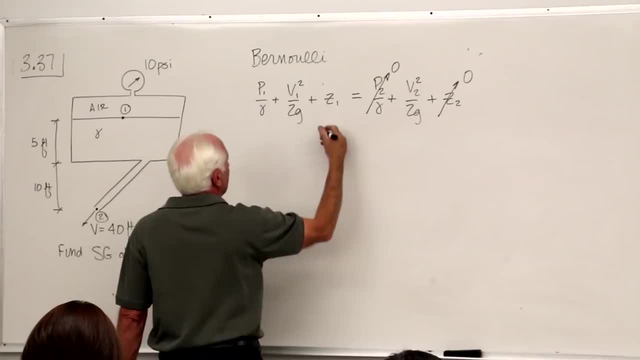 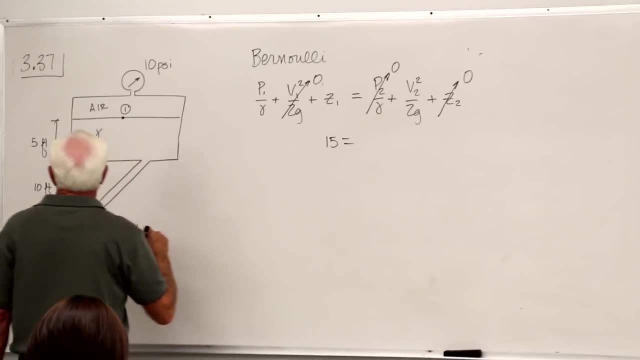 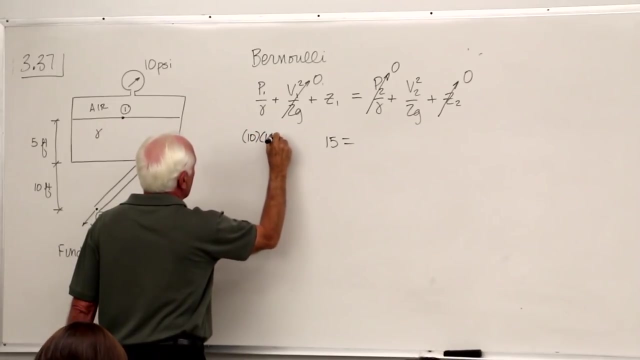 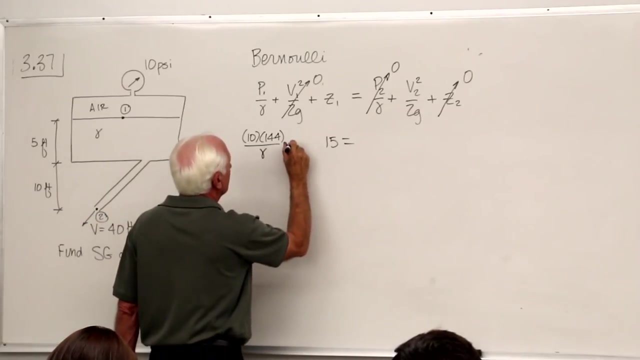 How far above is point one? 15 feet. What's the velocity at one? Zero? The pressure at one? 10 psi, 144.. Divided by what? Gamma Of what? The fluid in the tank Gamma, I don't know it. 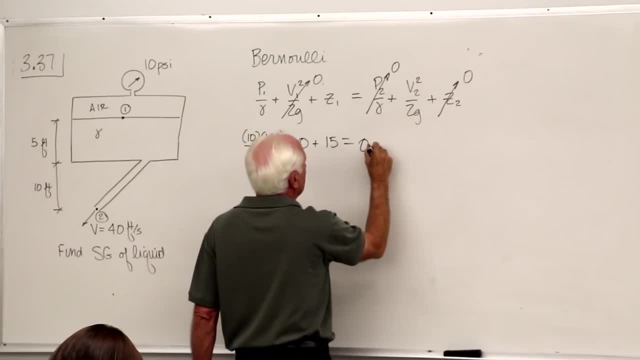 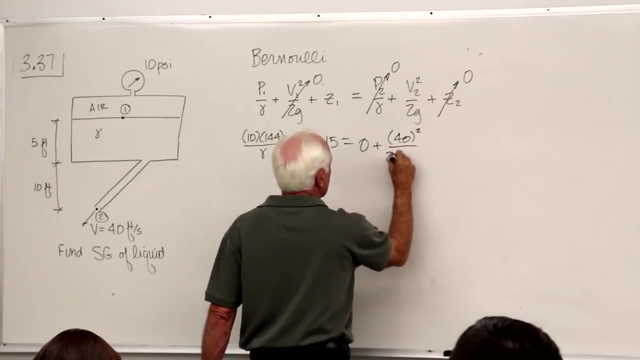 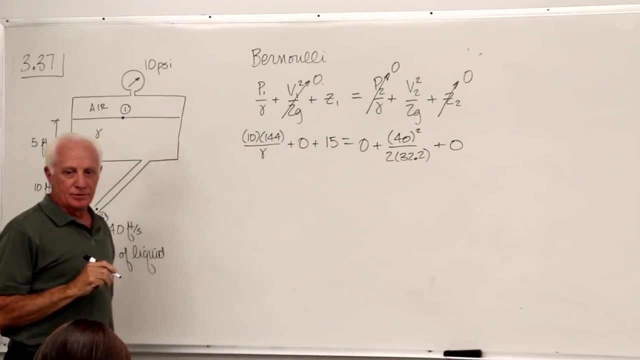 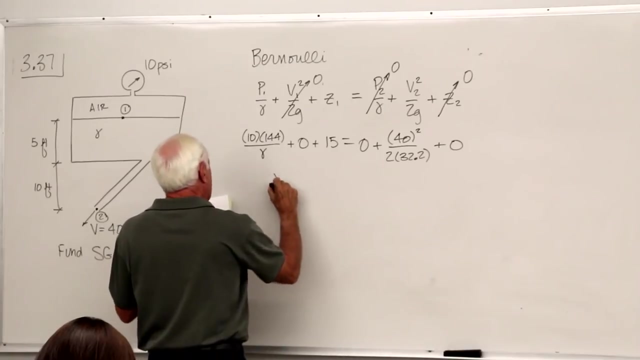 Equal. These guys are gone. Zero plus V2 squared Two: 32.2 plus zero. If you don't know G, always assume 32.2 or 9.81.. That's the default value. Solve for gamma.